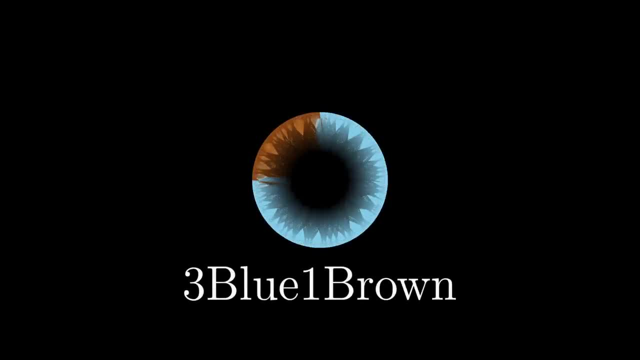 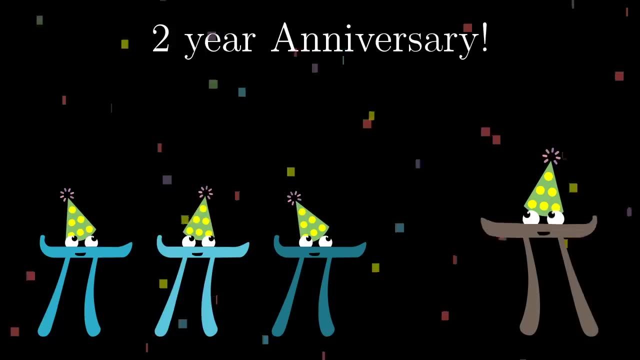 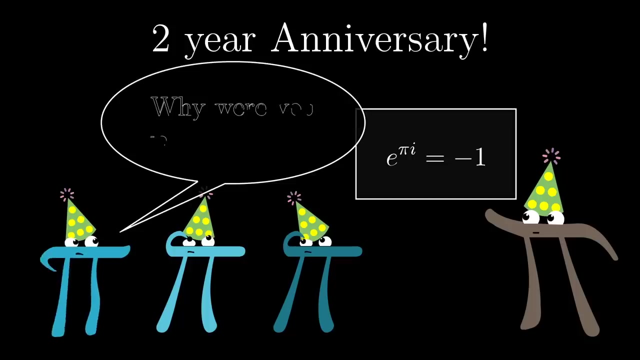 Two years ago, almost to the day actually, I put up the first video on this channel about Euler's formula e to the pi i equals negative 1.. As an anniversary, of sorts, I want to revisit that same idea. For one thing, I've always wanted to improve on the presentation, but 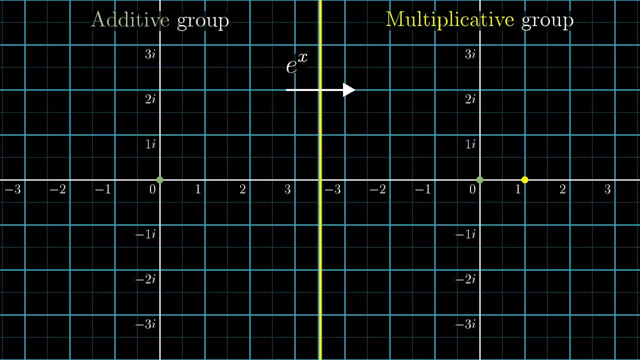 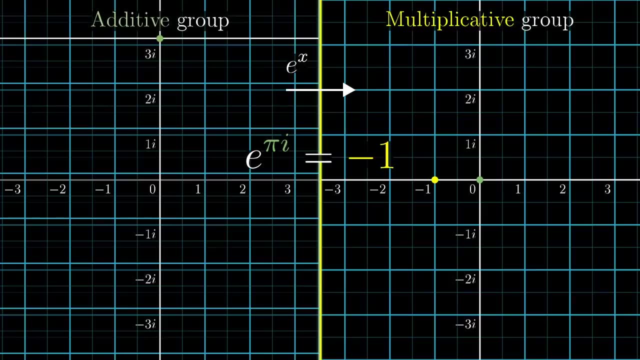 I wouldn't rehash an old topic if there wasn't something new to teach. You see, the idea underlying that video was to take certain concepts from a field in math called group theory and show how they give Euler's formula a much richer interpretation than a mere 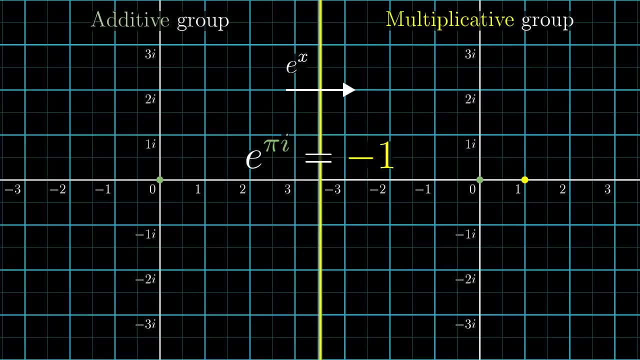 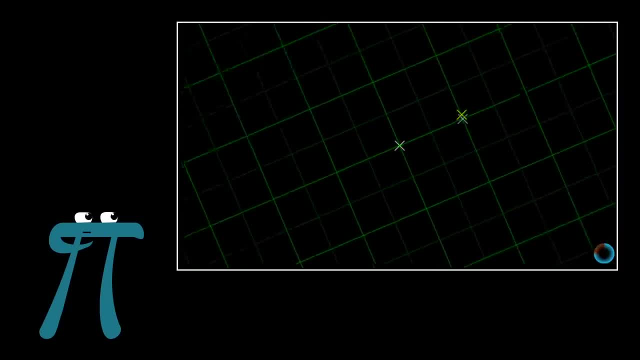 association between numbers, And two years ago I thought it might be fun to use those ideas without referencing group theory itself or any of the technical terms within it. But I've come to see that you all actually quite like getting into the math itself, even if 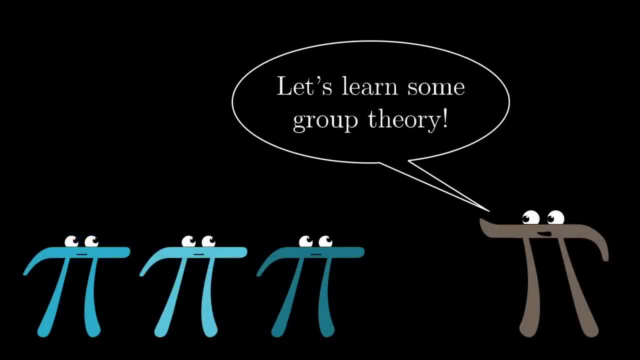 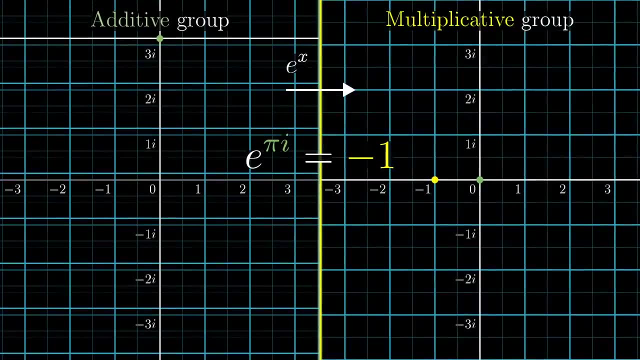 it takes some time. So here, two years later, let's you and me go through an introduction to the basics of group theory, building up to how Euler's formula comes to life under this light. If all you want is a quick explanation of Euler's formula, and if you're comfortable, 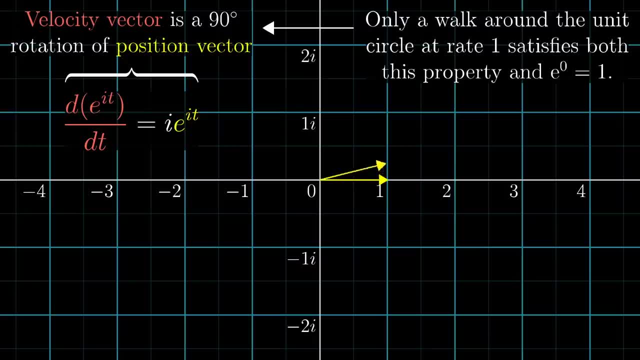 with vector calculus. I'll go ahead and put up a particularly short explanation on the screen that you can pause and ponder on. If it doesn't make sense, don't worry about it, it's not needed for where we're going. The reason that I want to put out this group theory view, though, is not because I think 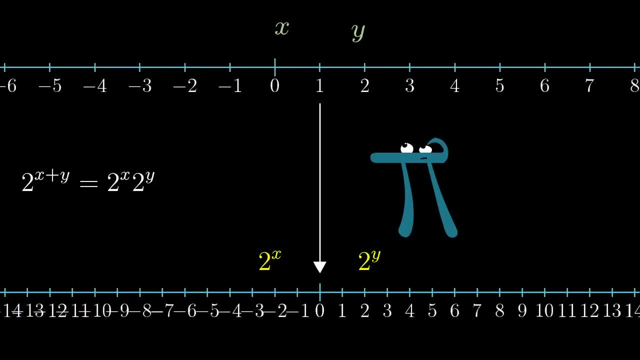 it's a better explanation. Heck, it's not even a complete proof, it's just an intuition. really. It's because it has the chance to change how you think about numbers and how you think about algebra. You see, group theory is all about studying the nature of symmetry. For example, a square. 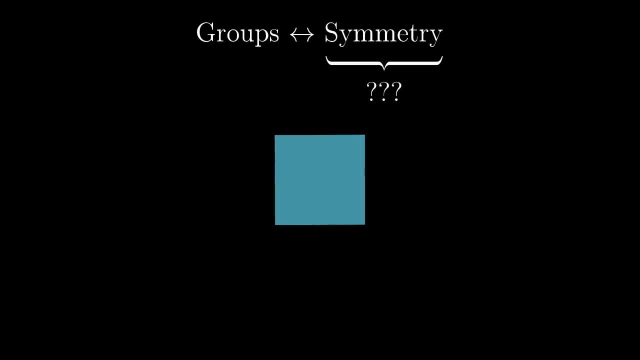 is a very symmetric shape, but what do we actually mean by that? One way to answer that is to ask about what are all the actions you can take on the square that leave it looking indistinguishable from how it started. For example, you could rotate it 90 degrees counterclockwise. 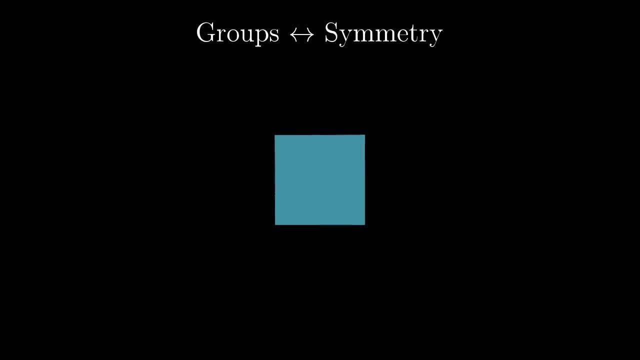 and it looks totally the same to how it started. You could also flip it around this vertical line, and again it still looks identical. In fact, the thing about such perfect symmetry is that it's hard to keep track of what action has actually been taken. so to help out, I'm 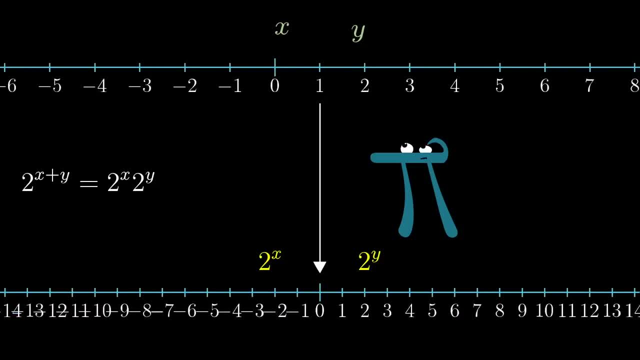 it's a better explanation. Heck, it's not even a complete proof, it's just an intuition. really. It's because it has the chance to change how you think about numbers and how you think about algebra. You see, group theory is all about studying the nature of symmetry. For example, a square. 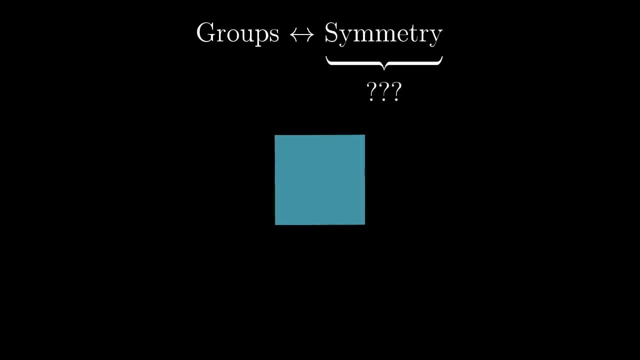 is a very symmetric shape, but what do we actually mean by that? One way to answer that is to ask about what are all the actions you can take on the square that leave it looking indistinguishable from how it started. For example, you could rotate it 90 degrees counterclockwise. 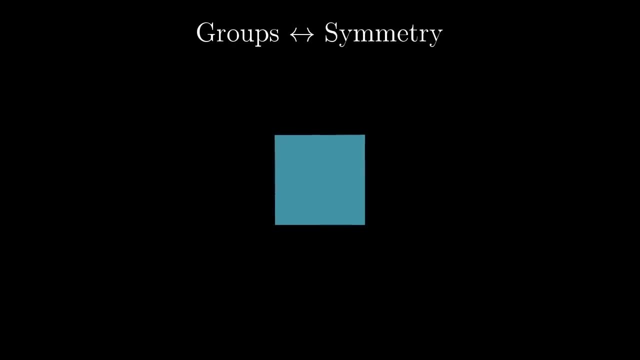 and it looks totally the same to how it started. You could also flip it around this vertical line, and again it still looks identical. In fact, the thing about such perfect symmetry is that it's hard to keep track of what action has actually been taken. so to help out, I'm 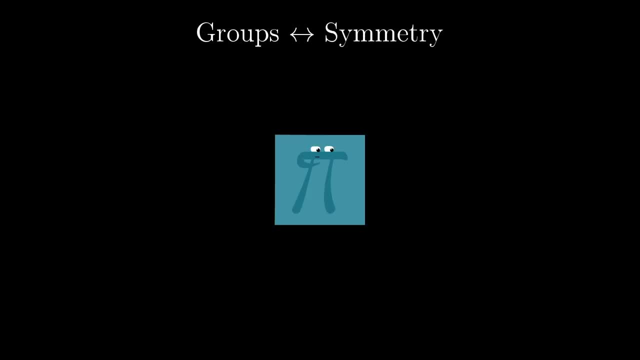 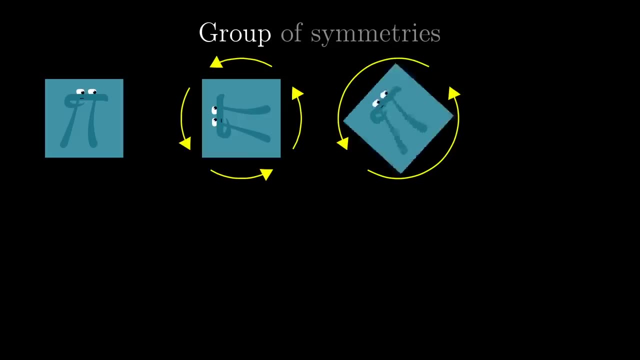 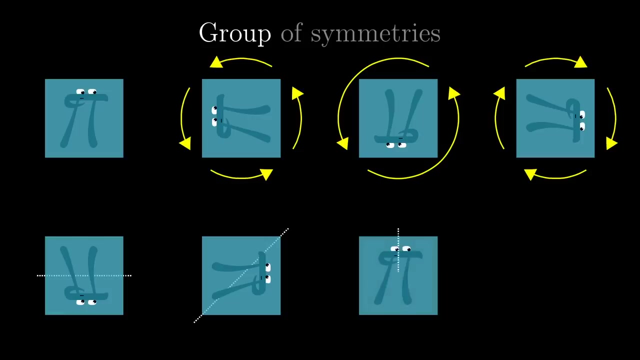 going to go ahead and stick on an asymmetric image. here We call each one of these actions a symmetry of the square, and all of the symmetries together make up a group of symmetries, or just group, for short, Symmetry of a square. 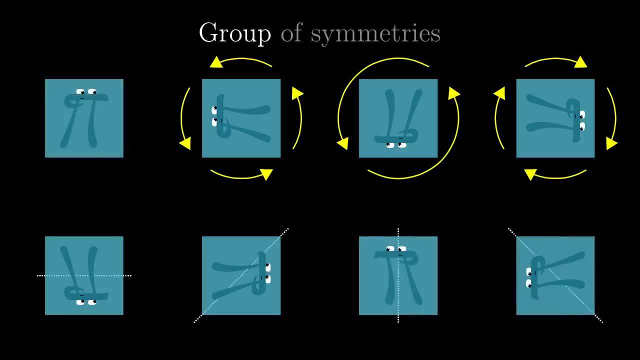 consists of 8 symmetries. There's the action of doing nothing, which is one that we count plus 3 different rotations, and then there's 4 ways that you can flip it over And, in fact, this group of 8 symmetries has a special name: It's called the dihedral group of order 8.. 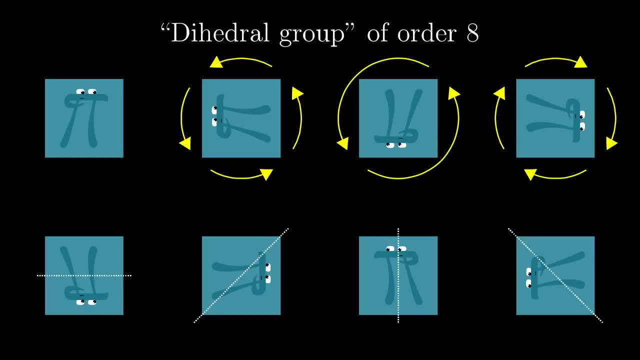 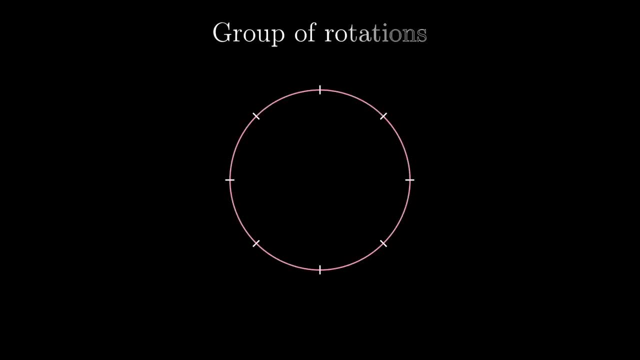 And that's an example of a finite group consisting of only 8 actions, But a lot of other groups consist of infinitely many actions. Think of all possible rotations, for example, of any angle. Maybe you think of this as a group that acts on a circle, capturing all of the symmetries. 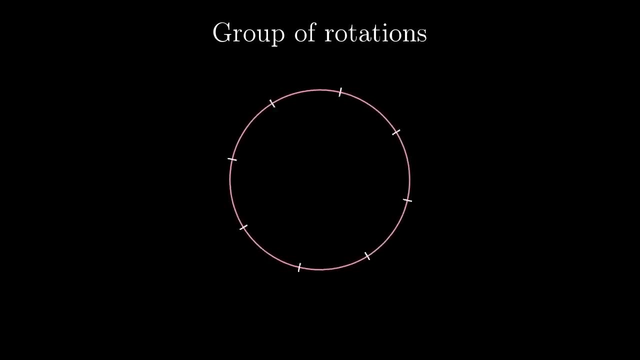 of that circle that don't involve flipping it Here. every action from this group of rotation lies somewhere on the infinite continuum between 0 and 2 pi radians. One nice aspect of these actions is that we can associate each one of them with a single. 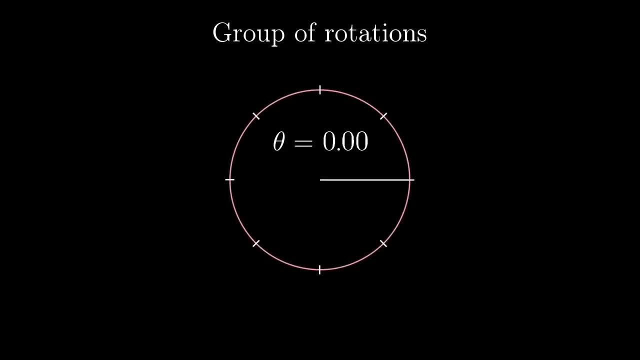 point on the circle itself, the thing being acted on. You start by choosing some arbitrary point, Maybe the one on the right here. Then every circle symmetry and every possible rotation takes this marked point to some unique spot on the circle And the 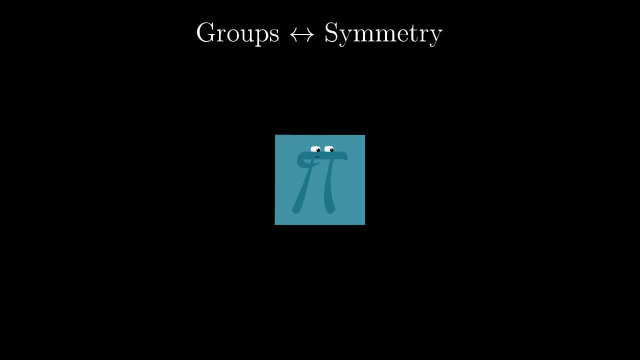 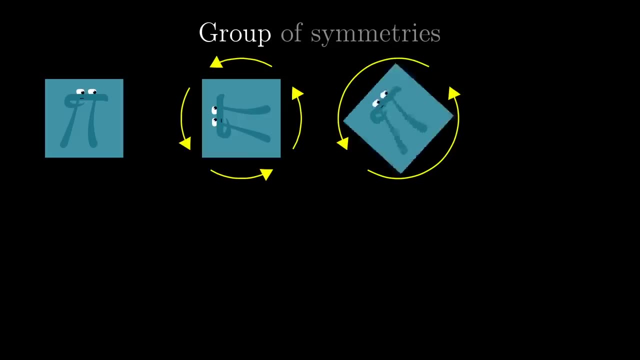 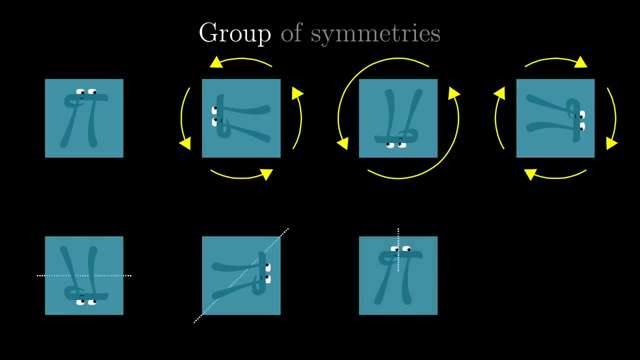 going to go ahead and stick on an asymmetric image. here. We call each one of these actions a symmetry of the square, and all of the symmetries together make up a group of symmetries, or just group for short. This particular group consists: 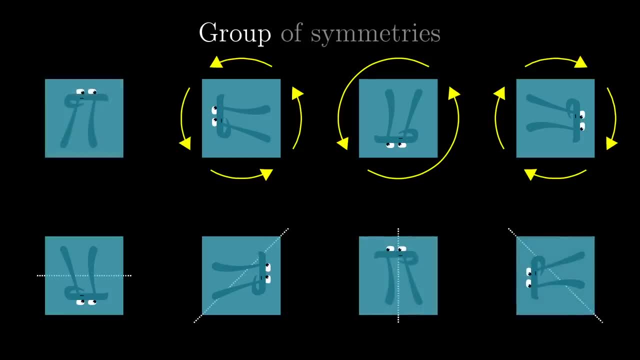 of eight symmetries. There's the action of doing nothing, which is one that we count plus three different rotations, and then there's four ways that you can flip it over And, in fact, this group of eight symmetries has a special name: It's called the dihedral group. 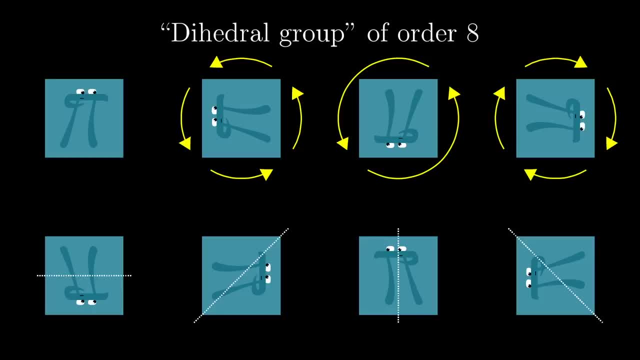 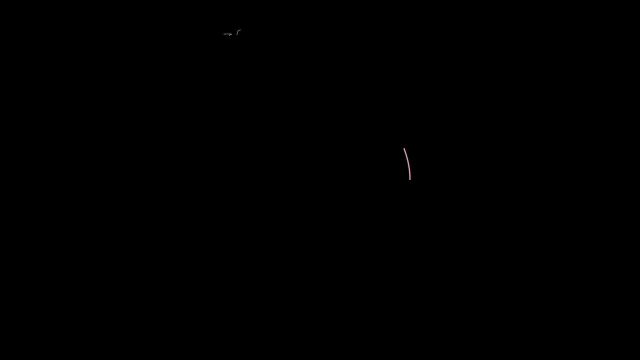 of order eight, And that's an example of a finite group consisting of only eight actions. But a lot of other groups consist of infinitely many actions. Think of all possible rotations, for example, of any angle. Maybe you think of this as a group that acts on a circle, capturing all of the symmetries. 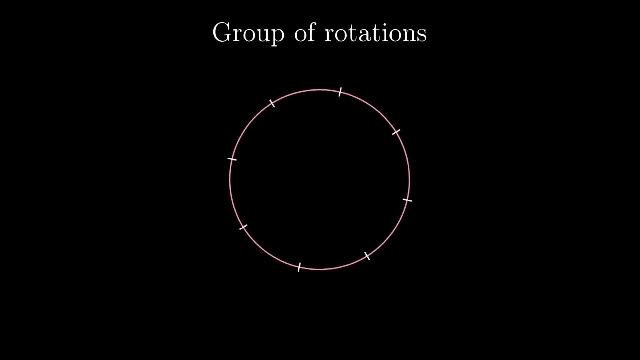 of that circle. that don't involve flipping it Here. every action from this group of rotation lies somewhere on the infinite continuum between zero and two pi radians. One nice aspect of these actions is that we can associate each one of them with a single. 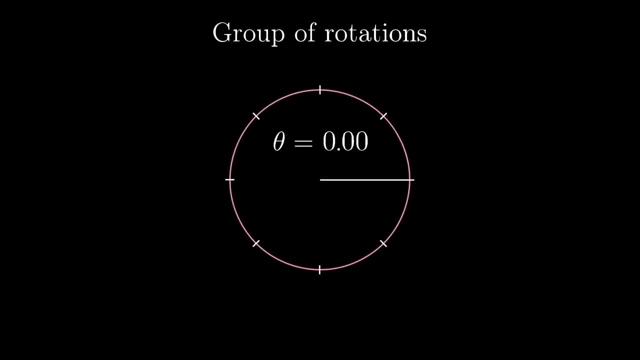 point on the circle itself, the thing being acted on. You start by choosing some arbitrary point, maybe the one on the right here. Then every circle, symmetry, every possible rotation takes this marked point to some unique spot on the circle and the action itself. 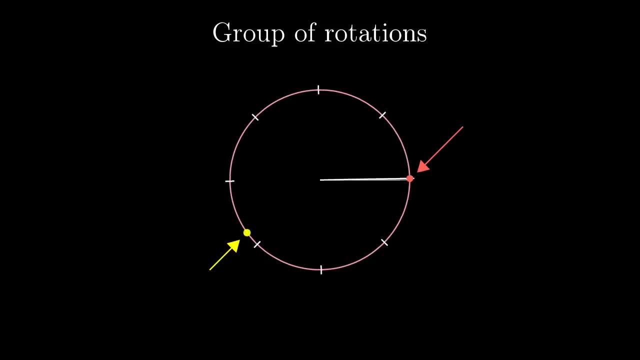 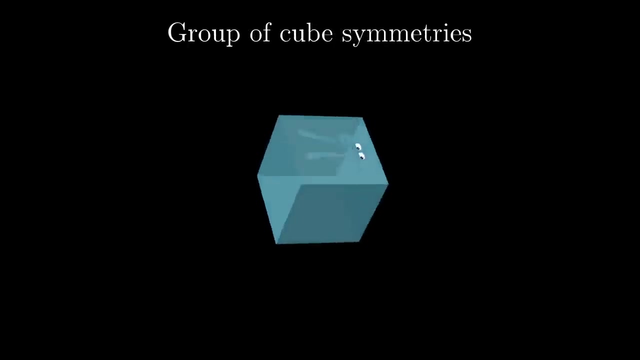 is completely determined by where it takes that spot. Now, this doesn't always happen with groups, but it's nice when it does happen, because it gives us a way to label the actions themselves, which can otherwise be pretty tricky to think about. The idea of groups is not just about what a particular set of symmetries is, whether 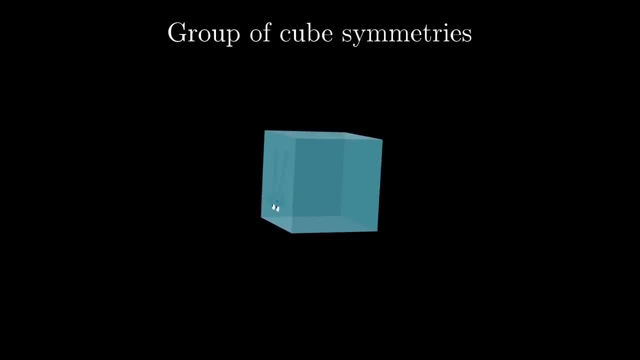 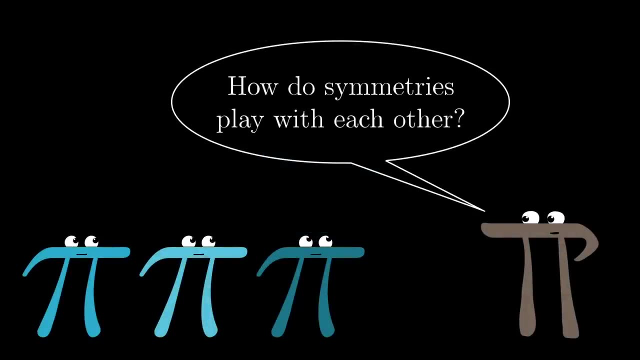 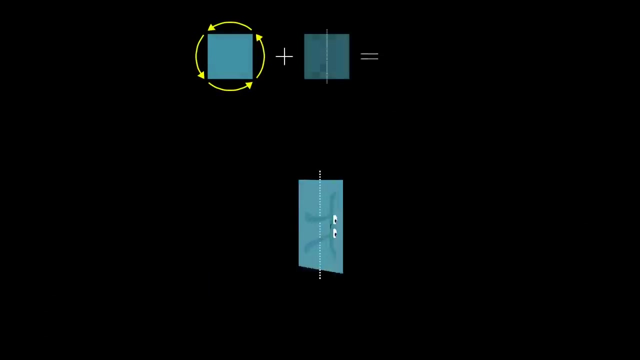 that's the 8 symmetries of a square, the infinite continuum of symmetries of the circle or anything else you dream up. The real heart and soul of the study is knowing how these symmetries play with each other On the square. if I rotate 90 degrees and then flip around the vertical axis, the overall 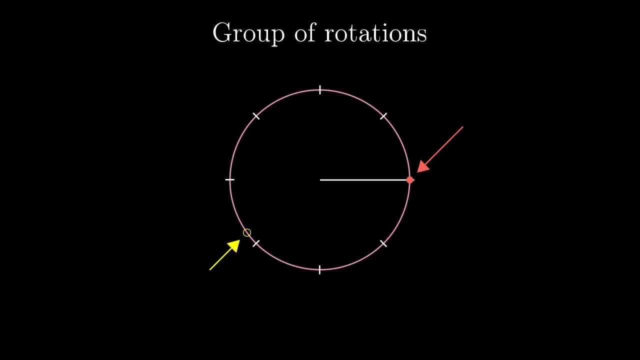 action itself is completely determined by where it takes that spot. Now, this doesn't always happen with groups, but it's nice when it does happen, because it gives us a way to label the actions themselves, which can otherwise be pretty tricky to think about. 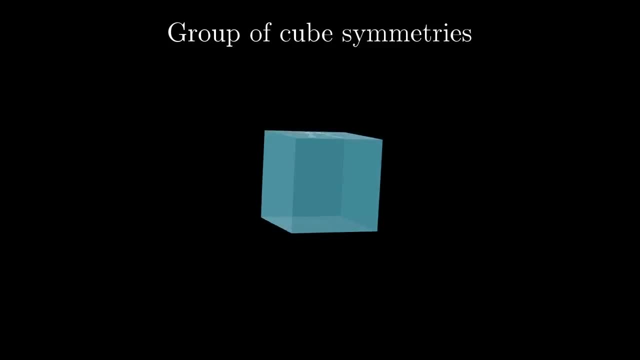 is not just about what a particular set of symmetries is, whether that's the eight symmetries of a square, the infinite continuum of symmetries of the circle or anything else you dream up, The real heart and soul of the study. 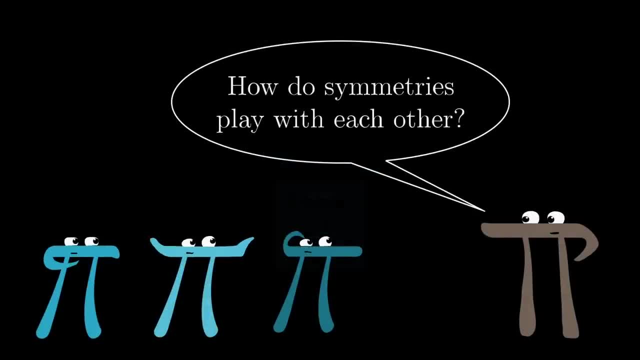 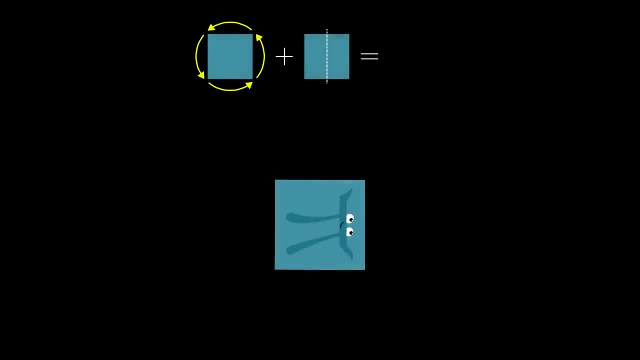 is knowing how these symmetries play with each other On the square. if I rotate 90 degrees and then flip around the vertical axis, the overall effect is the same as if I had just flipped over this diagonal line. So in some sense, that rotation- 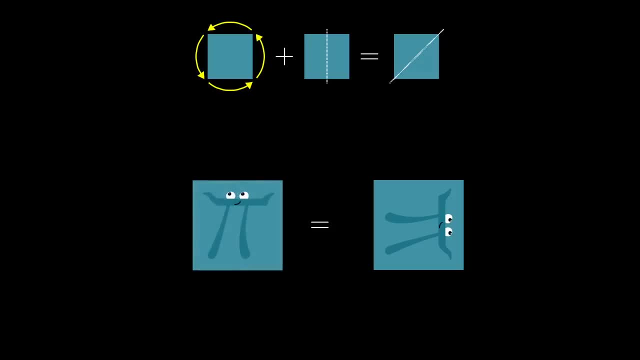 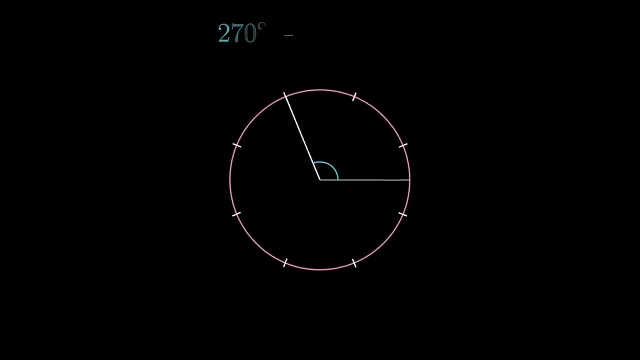 plus the vertical flip equals that diagonal flip On the circle. if I rotate 270 degrees and then follow it with a rotation of 120 degrees, the overall effect is the same as if I had just rotated 30 degrees to start with. So in this circle group, a 270-degree rotation. 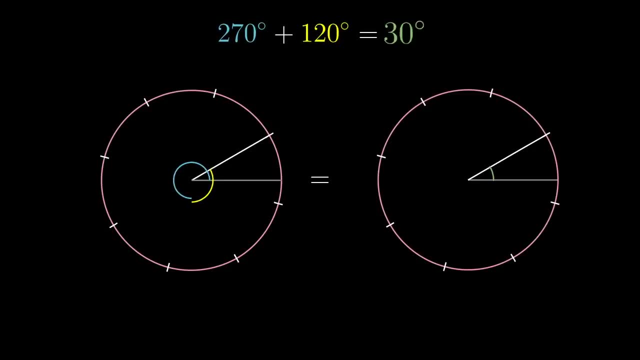 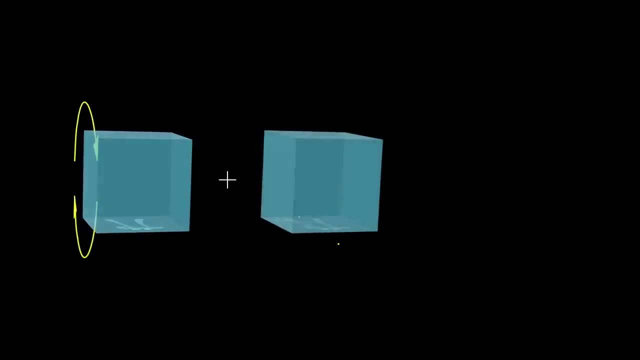 plus a 120-degree rotation equals a 30-degree rotation And in general, with any group, any collection of these sorts of symmetric actions, there's a kind of arithmetic where you can always take two actions and add them together to get a third one. 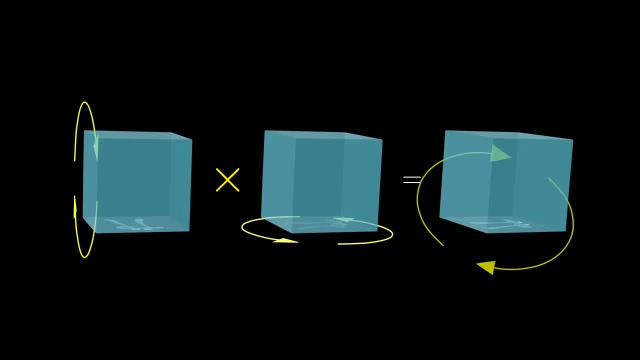 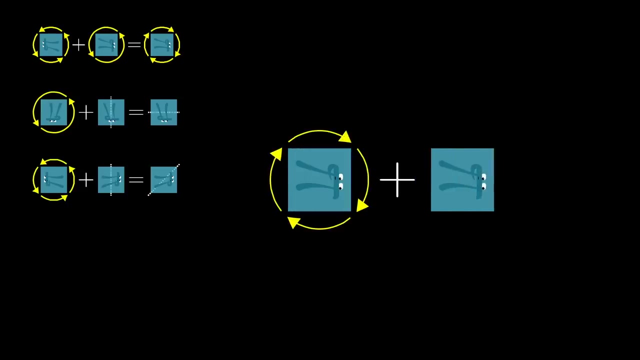 by applying one after the other. Or maybe you think of it as multiplying actions. It doesn't really matter. The point is that there is some way to combine the two actions, to get out another one, That collection of underlying relations, all associations between pairs of actions. 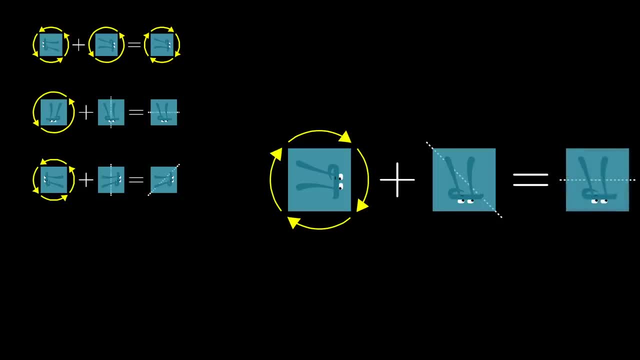 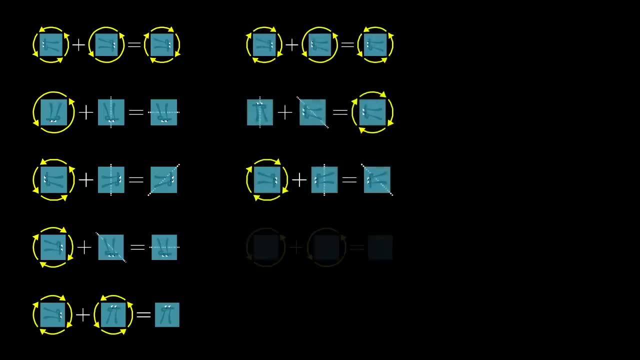 and the single action that's equivalent to applying one after the other. that's really what makes a group a group. It's actually crazy how much of modern math is rooted in well this, in understanding how a collection of actions is organized by this relation. 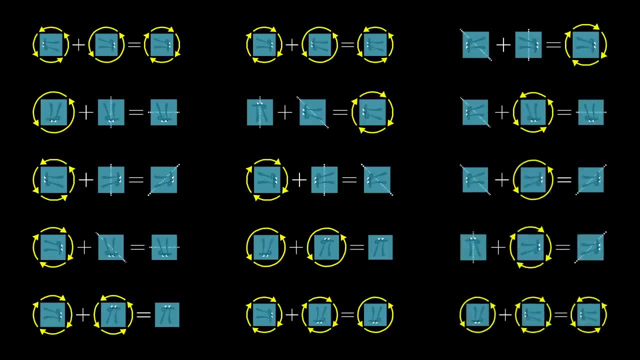 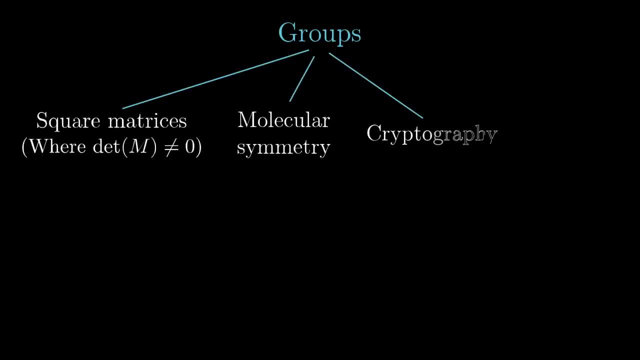 this relation between pairs of actions and the single action you get by composing them. Groups are extremely general. A lot of different ideas can be framed in terms of symmetries and composing symmetries, And maybe the most familiar example is numbers, just ordinary numbers. 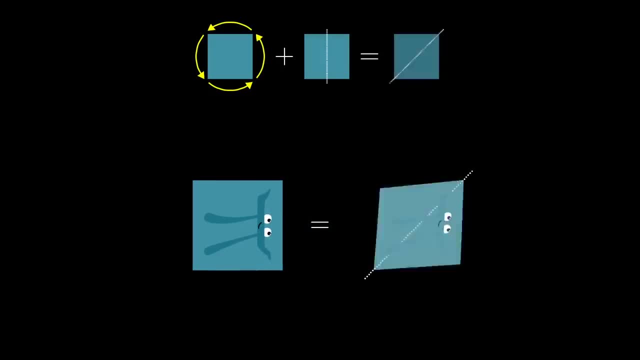 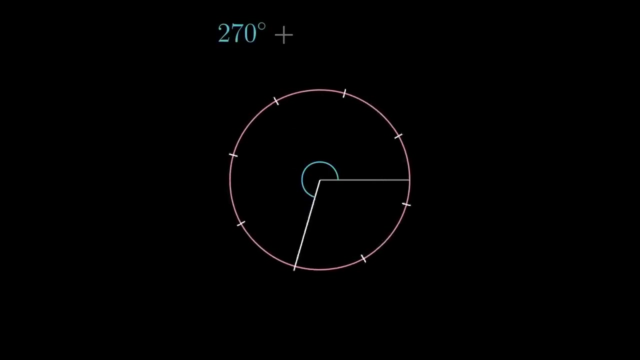 effect is the same as if I had just flipped over this diagonal line. So in some sense that rotation plus the vertical flip equals that diagonal flip On the circle. if I rotate 270 degrees and then follow it with a rotation of 120 degrees, 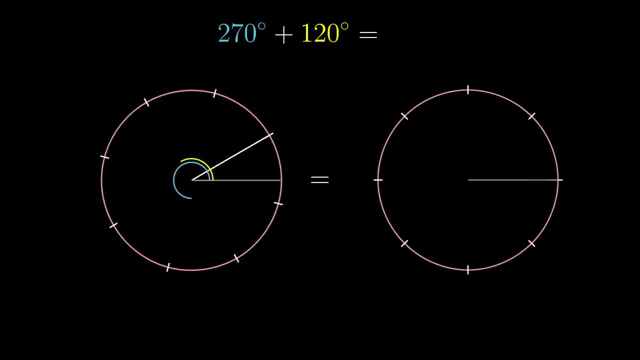 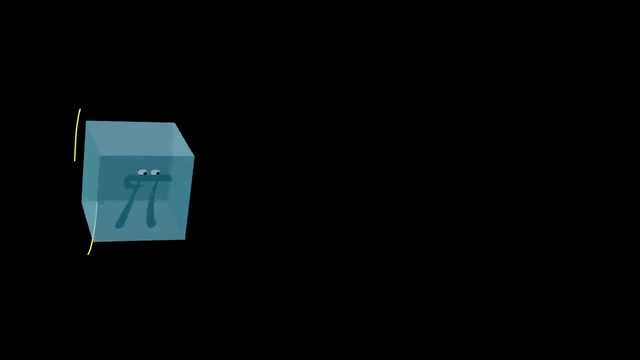 the overall effect is the same as if I had just rotated 30 degrees to start with. So in this circle group a 270 degree rotation plus a 120 degree rotation equals a 30 degree rotation. Throughout the earlier sections of the study we learned that with any group, any collection, 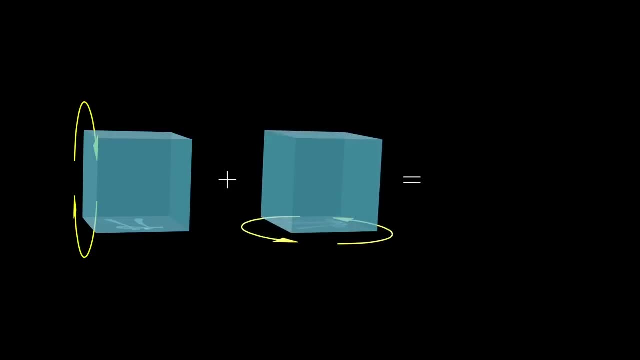 of these sorts of actions. there's a kind of arithmetic in which we can always take 2 actions and add them together to get a third one by applying one after the other. Or maybe you think of multiplying actions. It doesn't really matter. the point is that there is a way to combine the two actions. 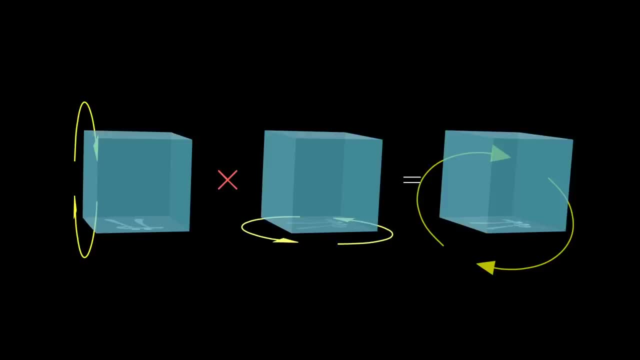 to get another one. That collection of underlying relations, That collection of underlying relations, All of that is actually the properties of a solved equation. It's really not all set up. it's all set up in one place. The whole things that are going to changes in time needs to be taken into account. 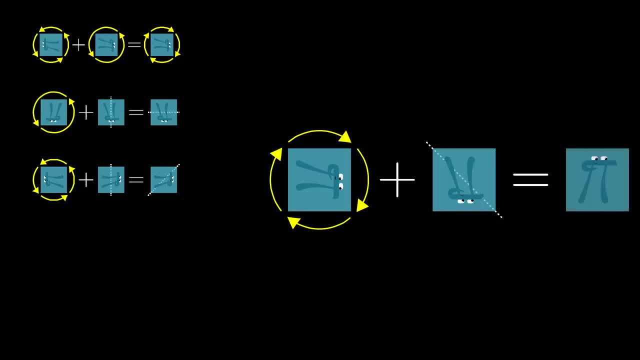 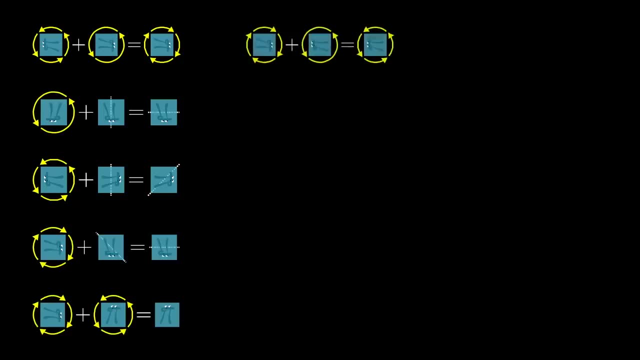 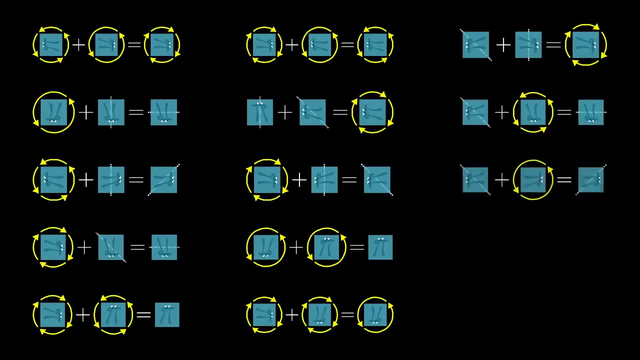 associations between pairs of actions and the single action. that's equivalent to applying one after the other. that's really what makes a group a group. It's actually crazy how much of modern math is rooted in well this, in understanding how a collection of actions is organized by this relation. 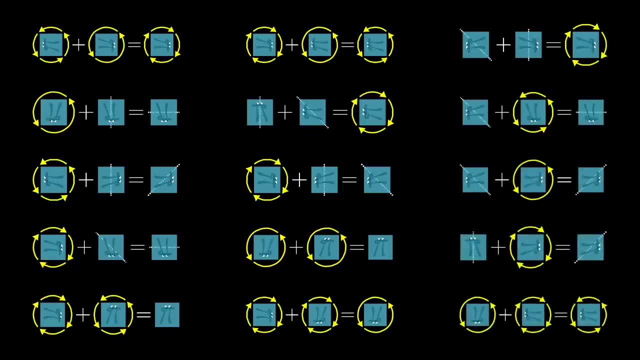 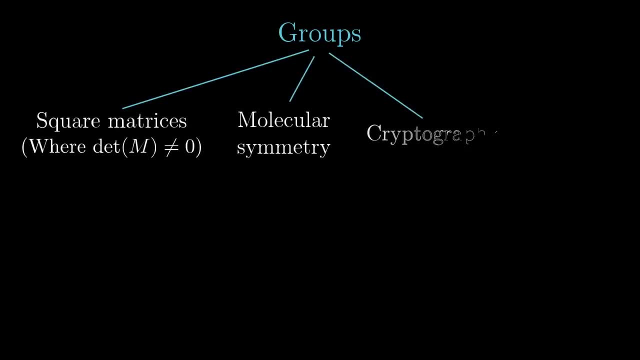 this relation between pairs of actions and the single action you get by composing them. Groups are extremely general. A lot of different ideas can be framed in terms of symmetries and composing symmetries, and maybe the most familiar example is numbers, just ordinary numbers, and there are actually. 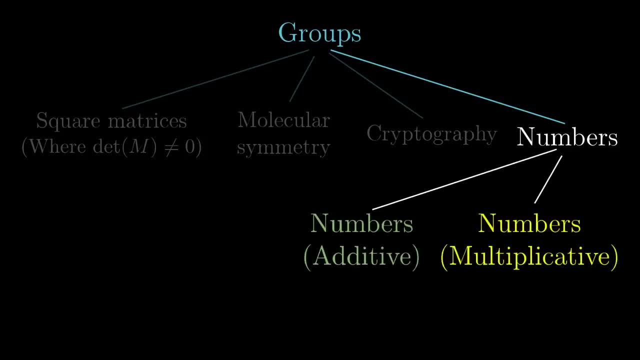 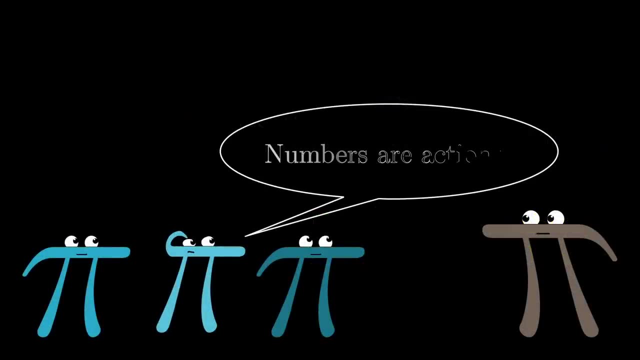 two separate ways to think about numbers as a group: one where composing actions is gonna look like addition and another where composing actions will look like multiplication. It's a little weird, because we don't usually think of numbers as actions. we usually think of them as counting things. 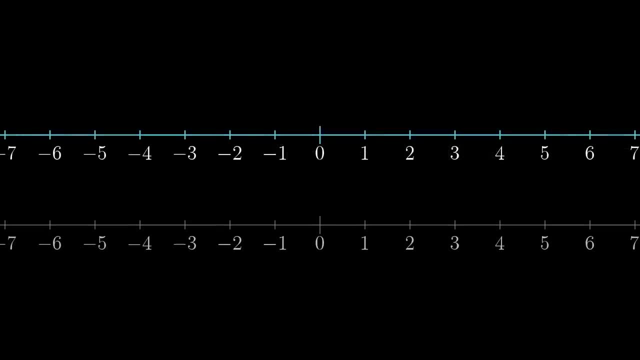 But let me show you what I mean. Think of all of the ways that you can slow down and compute and multiply things. if you can just think of them asWork slide a number line left or right along itself. This collection of all sliding actions is a group, what you might think of as the group. 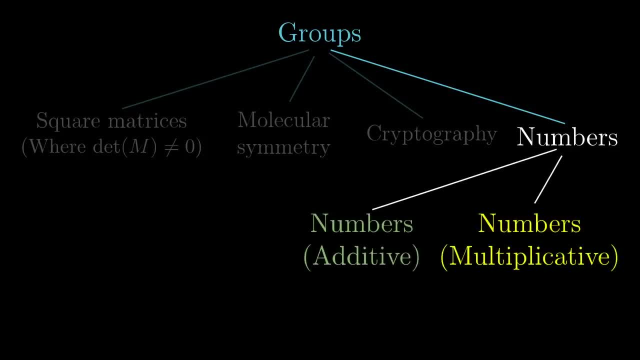 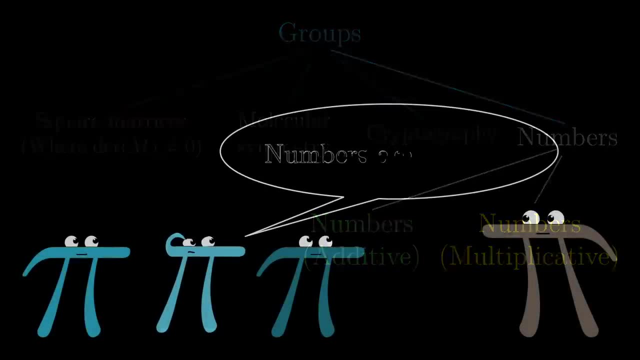 And there are actually two separate ways to think about numbers as a group: one where composing actions is gonna look like addition and another where composing actions will look like multiplication. It's a little weird, because we don't usually think of numbers as actions. We usually think of them as counting things. 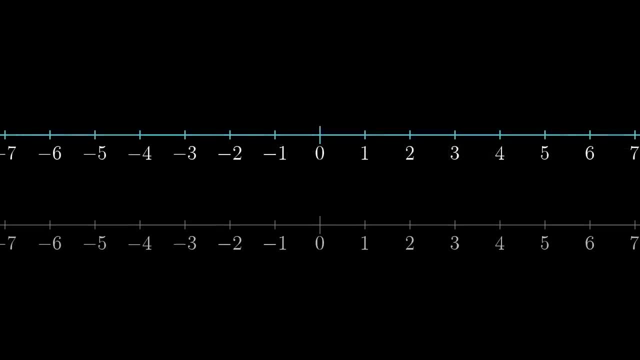 But let me show you what I mean. Think of all of the ways that you can slide a number line left or right along itself. This collection of all sliding actions is a group, what you might think of as the group of symmetries. 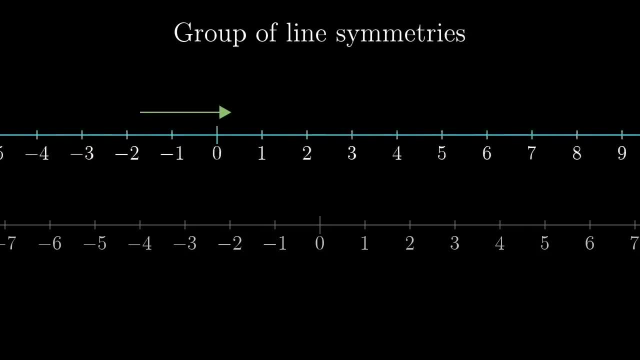 on an infinite line, And in the same way that actions from the circle group could be associated with individual points on that circle. this is another one of those special groups where we can associate each action with a unique point on the thing that it's actually acting on. 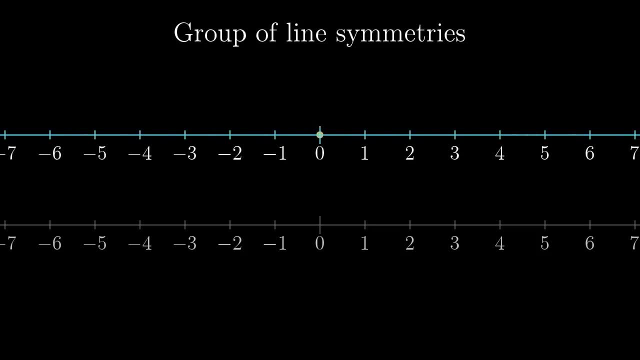 You just follow where the point that starts at zero ends up. For example, the number three is associated with the action of sliding right by three units. The number negative two is associated with the action of sliding two units to the left, since that's the unique action that drags the point at zero. 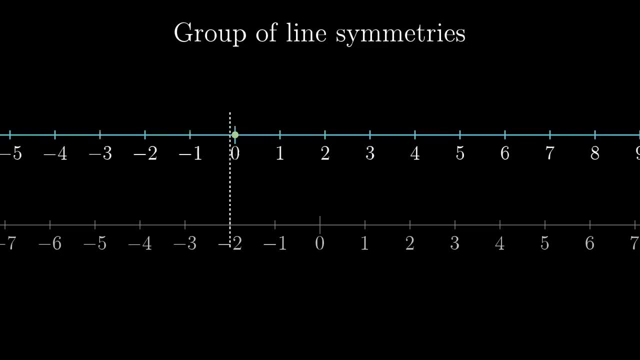 over to the point at negative two, The number zero itself. well, that's associated with the action of just doing nothing. This group of sliding actions, each one of which is associated with a unique real number, has a special name: It's the additive group of real numbers. 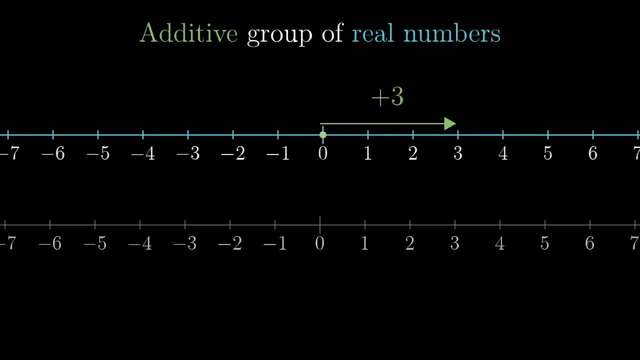 The reason the word additive is in there is because of what the group operation of applying one action followed by another looks like. If I slide right by three units and then I slide right by two units, the overall effect is the same as if I slid right. 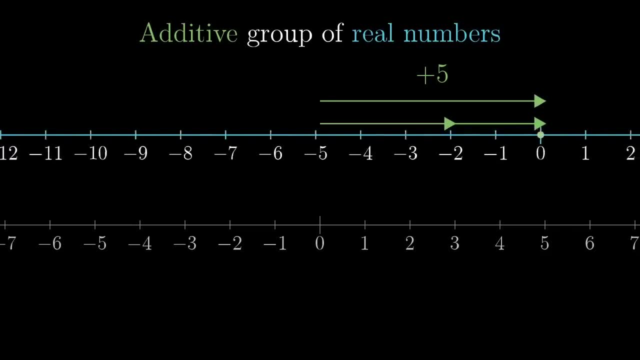 by 3 plus 2, or five units. Simple enough, we're just adding the distances of each slide. But the point here is that this gives an alternate view for what numbers even are. They are one example, a much larger category of groups, groups of symmetries acting on some object, and the 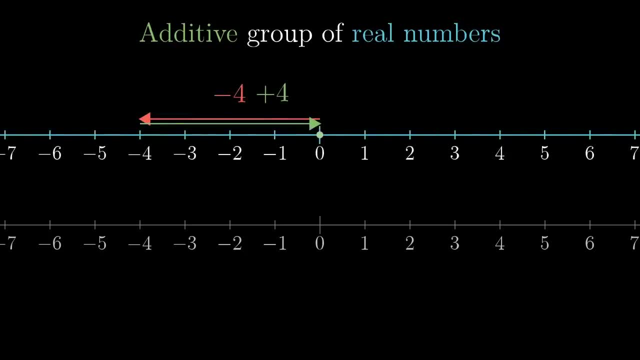 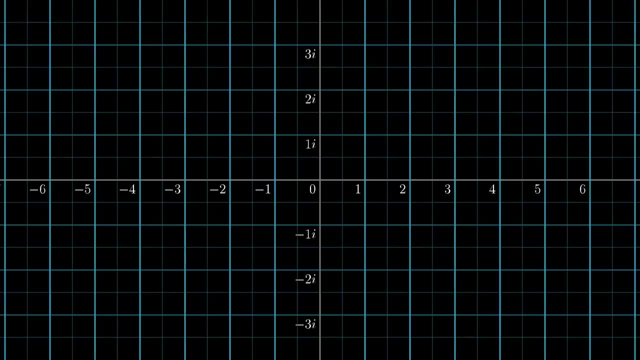 arithmetic of adding numbers is just one example of the arithmetic that any group of symmetries has within it. We could also extend this idea, instead asking about the sliding actions on the complex plane. The newly introduced numbers i, 2i, 3i and so on on this vertical line would all be associated. 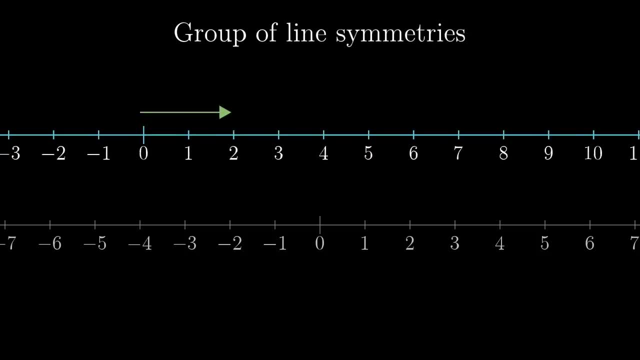 of symmetries on an infinite line, And in the same way that actions from the circle group could be associated with individual points on that circle, this is another one of those special groups where we can associate each action with a unique point on the thing that it's actually acting on. 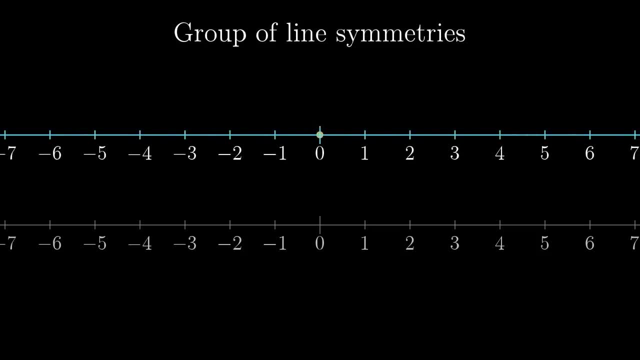 You just follow where the point that starts at 0 ends up. For example, the number 3 is associated with the action of sliding right by 3 units. The number negative 2 is associated with the action of sliding 2 units to the left, since 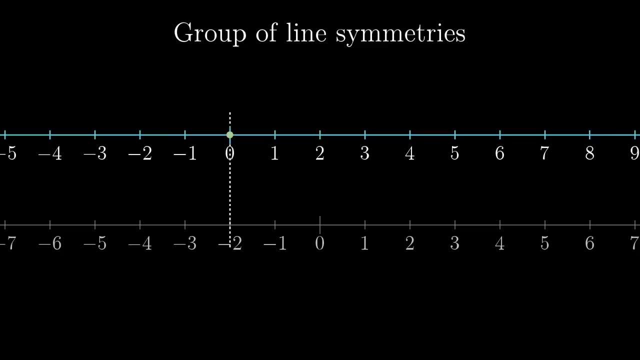 that's the unique action that drags the point at 0 over to the point at negative 2.. The number 0 itself is associated with the action of just doing nothing. This group of sliding actions, Each one of which is associated with a unique real number, has a special name: the additive. 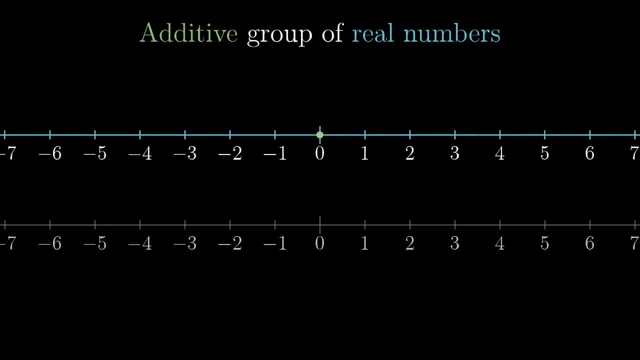 group of real numbers. The reason the word additive is in there is because of what the group operation of applying one action followed by another looks like. If I slide right by 3 units and then I slide right by 2 units, the overall effect is the. 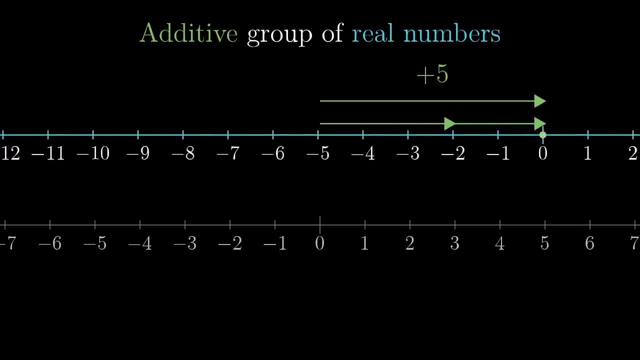 same as if I slid right by 3 plus 2, or 5 units. Simple enough, we're just adding the distances of each slide. But the point here is that this gives an alternate view for what numbers even are. They are one example in a much larger category of groups, groups of symmetries acting on. 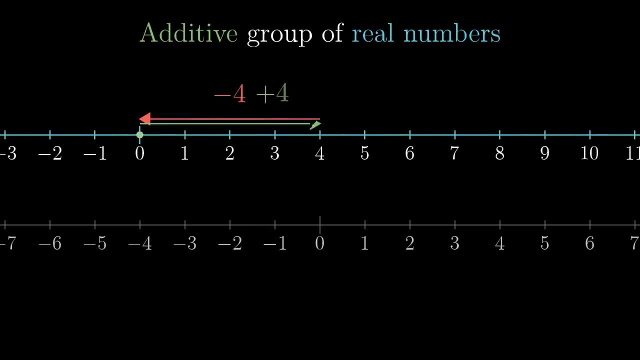 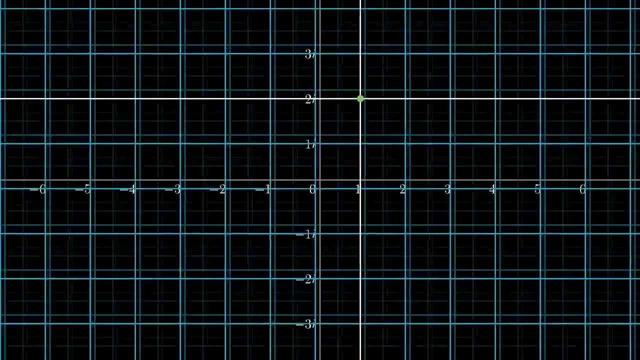 some object, And the arithmetic of adding numbers is just one example of the arithmetic that any group of symmetries has within it. We could also extend this idea instead asking about the sliding actions on the complex plane, The newly introduced numbers i, 2, r, etc. 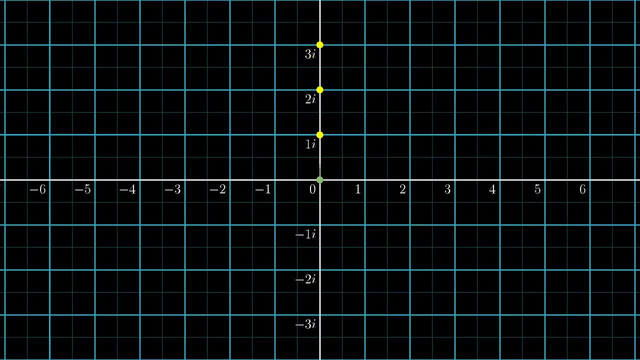 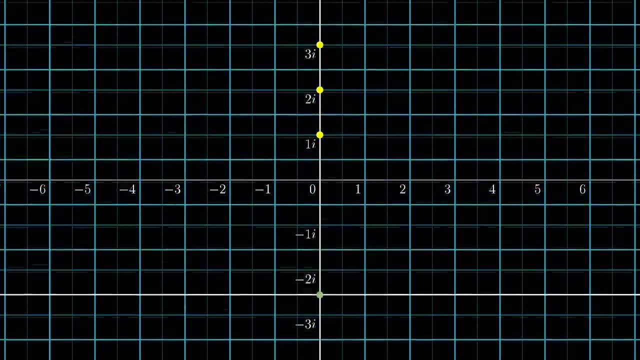 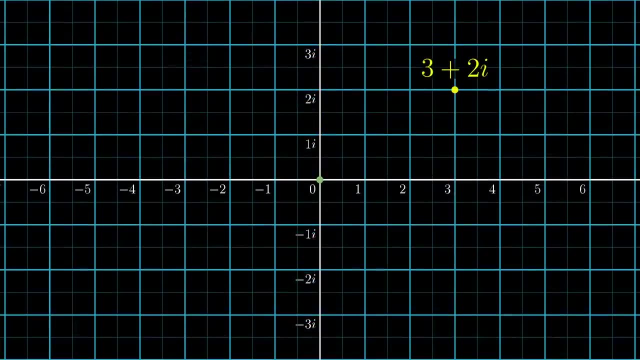 2i, 3i and so on on this vertical line would all be associated with vertical sliding motions, since those are the actions that drag the point at 0 up to the relevant point on that vertical line. The point over here, at 3 plus 2i, would be associated with the action of sliding the 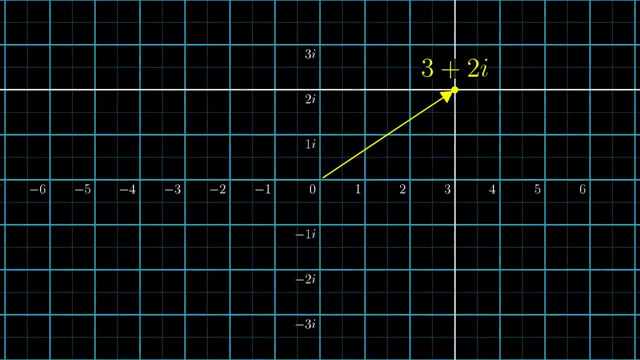 plane in such a way that drags 0 up and to the right to that point, And it should make sense why we call this 3 plus 2i Right. That diagonal sliding action is the same as first sliding by 3 to the right and then 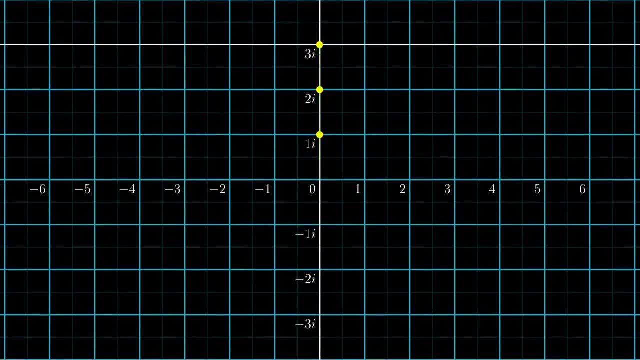 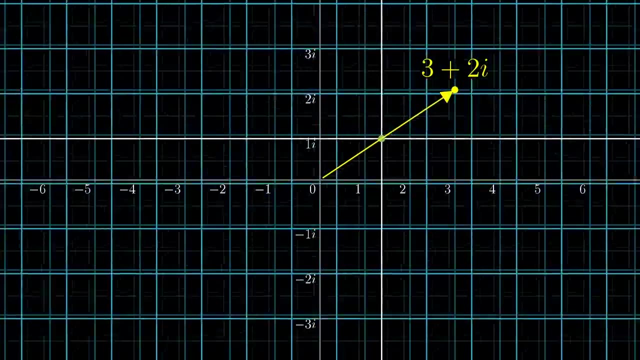 with vertical sliding motions, since those are the actions that drag the point at zero up to the relevant point on that vertical line. The point over here, at 3 plus 2i, would be associated with the action of sliding the plane in such a way that drags zero up and to the right to that point. 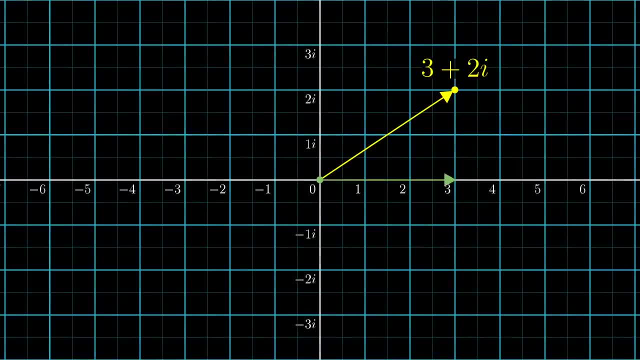 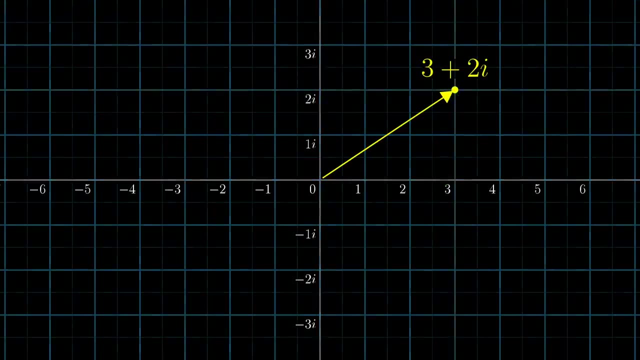 And it should make sense why we call this 3 plus 2i. That diagonal sliding action is the same as first sliding by 3 to the right and then following it with a slide that corresponds to 2i, which is two units vertically. Similarly, let's get a feel for how composing any two of these. 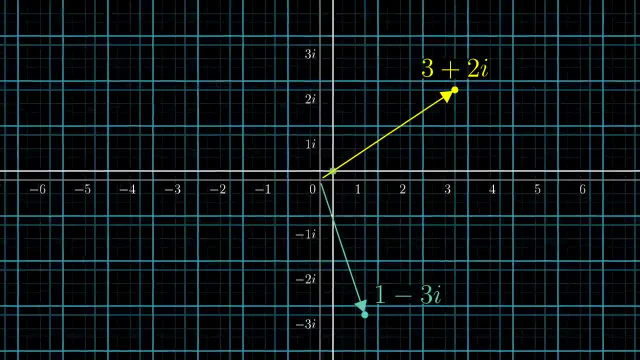 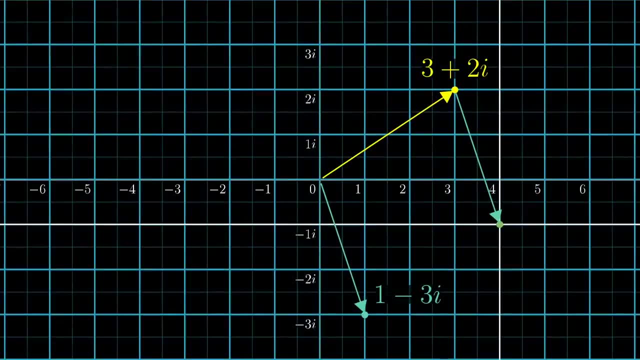 actions generally breaks down. Consider this slide by 3 plus 2i action as well as this slide by 1 minus 3i action, and imagine applying one of them right after the other. The overall effect, the composition of these two sliding actions. 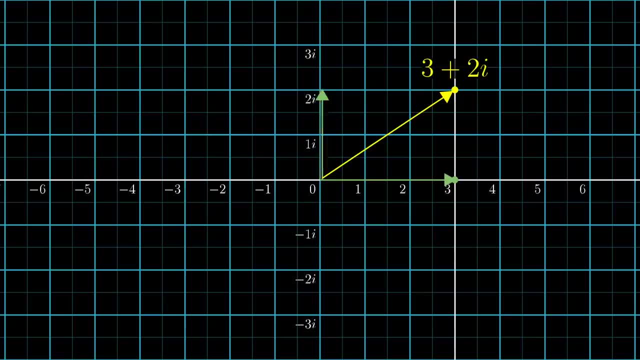 following it with a slide that corresponds to 2i, which is 2 units vertically. Similarly, let's get a feel for how composing any two of these actions generally breaks down. Consider this slide by 3 plus 2i action, as well as this slide by 1 minus 3i action, and. 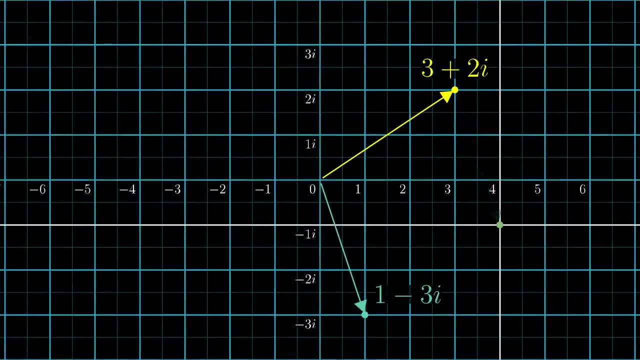 imagine applying one of them right after the other. The overall effect, the composition of these two sliding actions, is the same as if we had slid 3 plus 1 to the right and 2 minus 3 vertically. Notice how that involves adding together each component. 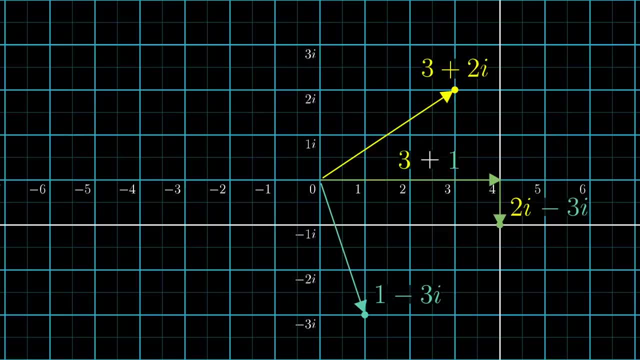 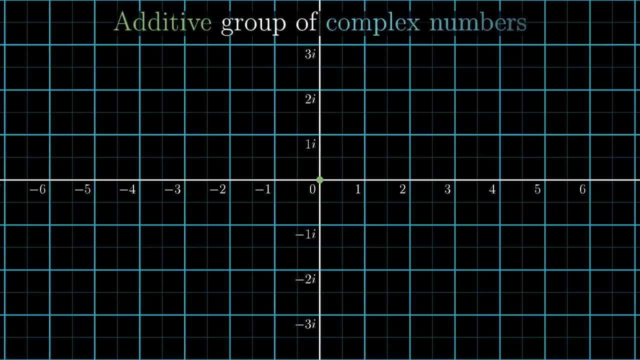 So composing sliding actions is another way to think about what adding complex numbers actually means. This collection of all sliding actions on the 2D complex plane goes by the name the additive group of complex numbers. Again, the upshot here is that numbers, even complex numbers, are just one example of 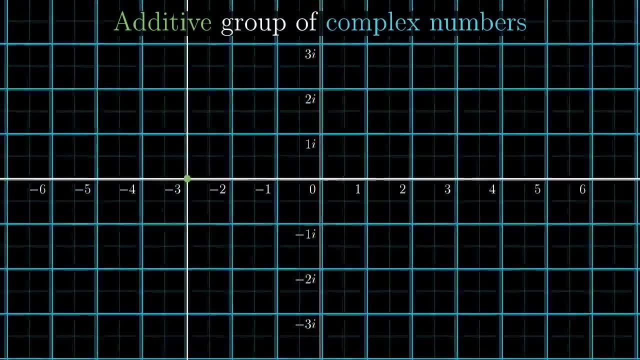 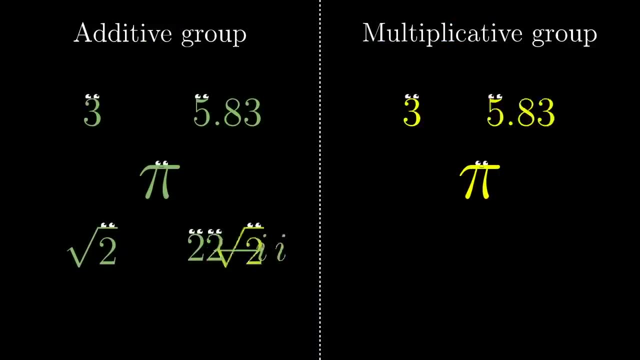 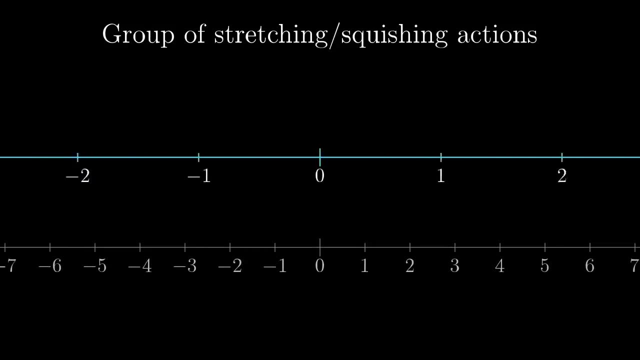 a group and the idea of addition can be thought of in terms of successively applying actions. But numbers, schizophrenic as they are, also lead a completely different life as a completely different kind of group. Consider a new group of actions on the number line, all ways that you can stretch or squish. 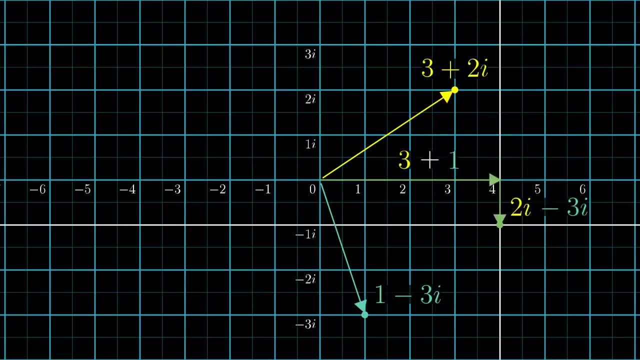 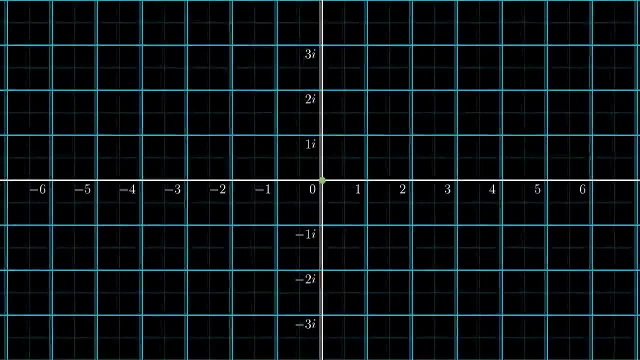 is the same as if we had slid 3 plus 1 to the right and 2 minus 3 vertically. Notice how that involves adding together each component. So composing sliding actions is another way to think about what adding complex numbers actually means. This collection of all sliding actions on the 2d complex plane goes by. 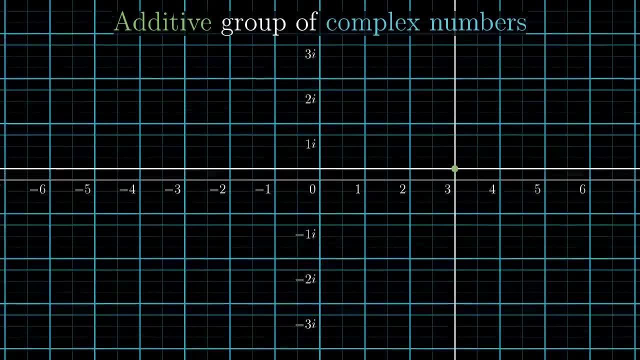 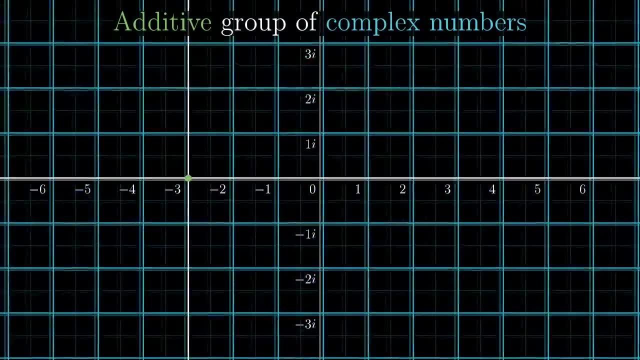 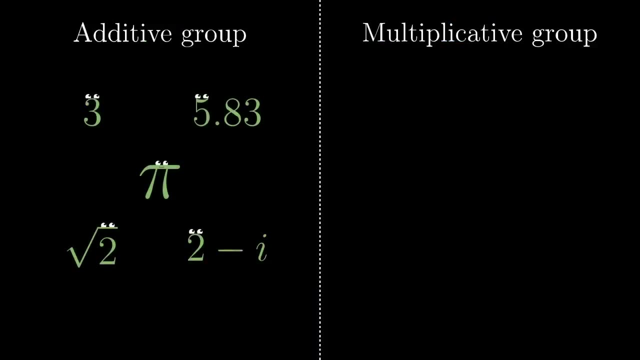 the name, the additive group of complex numbers. Again, the upshot here is that numbers, even complex numbers, are not always the same. Numbers are just one example of a group and the idea of addition can be thought of in terms of successively applying actions. But numbers, schizophrenic as they, 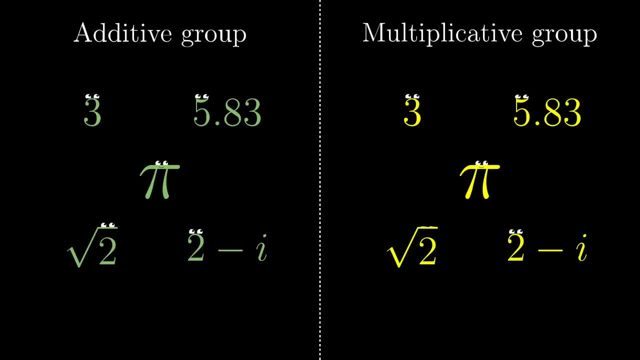 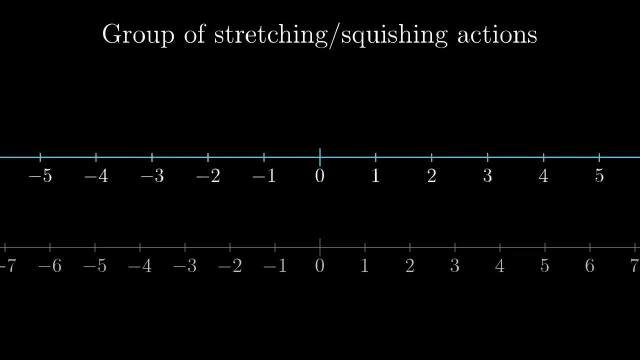 are also lead a completely different life as a completely different kind of group. Consider a new group of actions on the number line, all ways that you can stretch or squish it, keeping everything evenly spaced and keeping that number zero fixed in place Yet again. this group of actions has that nice. 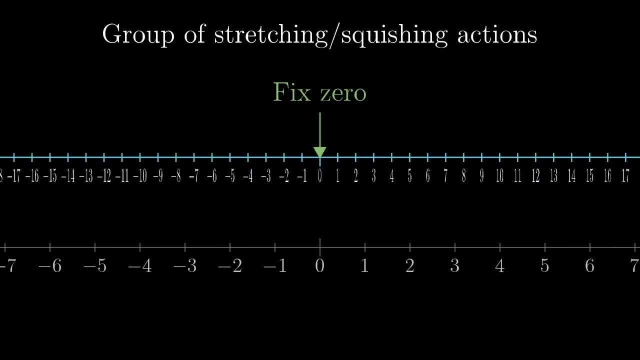 property, where we can associate each action in the group with a specific point on the thing that it's acting on. In this case, follow where the point that starts at the number one goes. There is one and only one stretching action that brings that point at one to the point at three, for instance, namely stretching by. 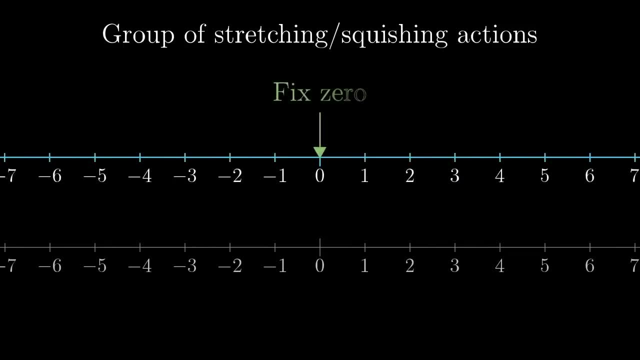 it, keeping everything evenly spaced and keeping that number zero fixed in place. Yet again, this group of actions has that nice property where we can associate each action in the group with a specific point on the thing that it's acting on, In this case, follow where the point that starts at the number 1 goes. 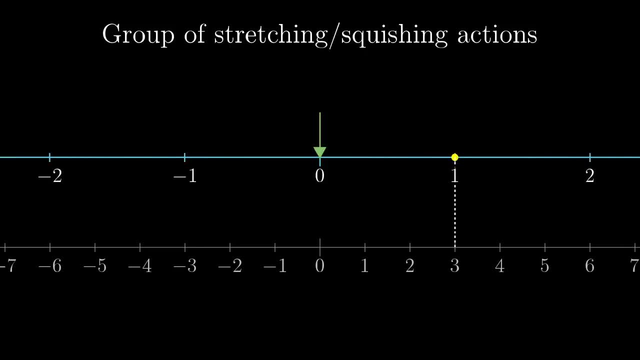 There is one and only one stretching action that brings that point at 1 to the point at 3, for instance, namely stretching by a factor of 3.. Likewise, there is one and only one action that brings that point at 1 to the point at. 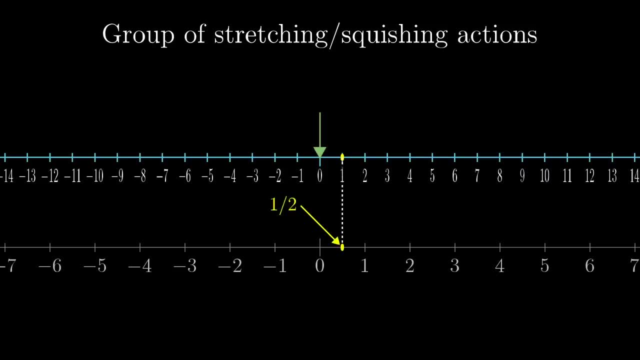 1⁄2, namely squishing by a factor of 1⁄2.. I like to imagine using one hand to fix the number zero in place and using the other to drag the number 1 wherever I like, while the rest of the number line just does whatever. 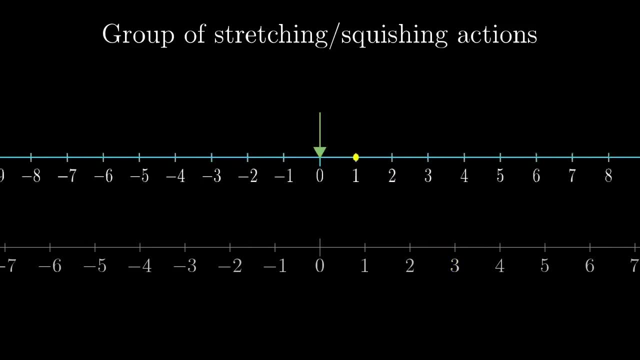 a factor of three. Likewise, there is one and only one action that brings that point at one to the point at one-half, namely squishing by a factor of one-half. I like to imagine using one hand to fix the number zero in place and using the. 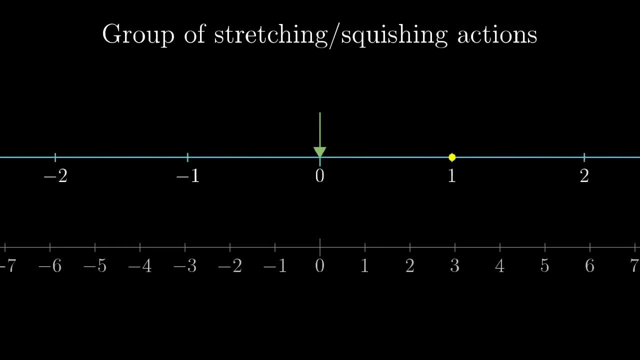 other to drag the number one wherever I like, while the rest of the number line just does whatever it takes to stay evenly spaced. In this way, every single positive number is associated with a unique stretching or squishing action. Now notice what composing actions look like in this group If I apply the 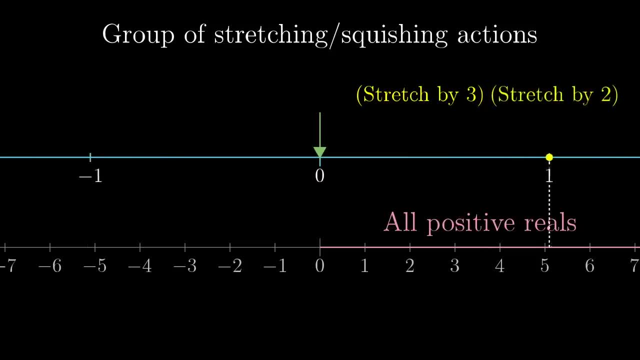 stretch-by-three action and then follow it with a longer-stretching action, then it should look like this: then follow it with the stretch by two action. the overall effect is the same as if I had just applied the stretch by six action, the product of the two original numbers. 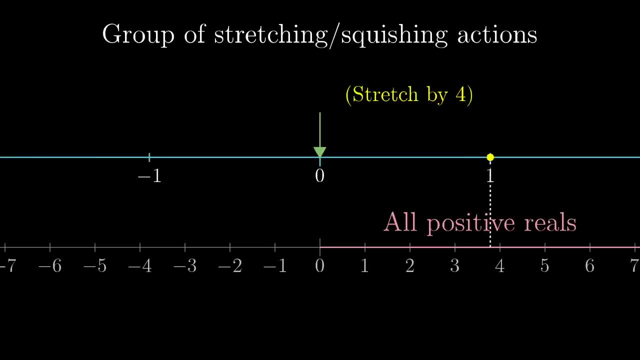 And, in general, applying one of these actions followed by another corresponds with multiplying the numbers that they're associated with. In fact, the name for this group is the multiplicative group of positive real numbers. So multiplication- ordinary familiar multiplication- is one more example of this very general and very far-reaching idea of groups and the arithmetic within groups. 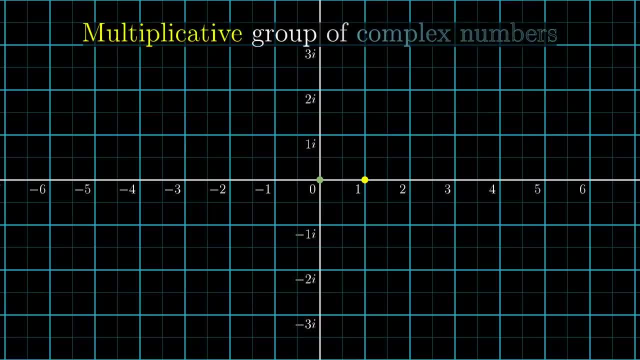 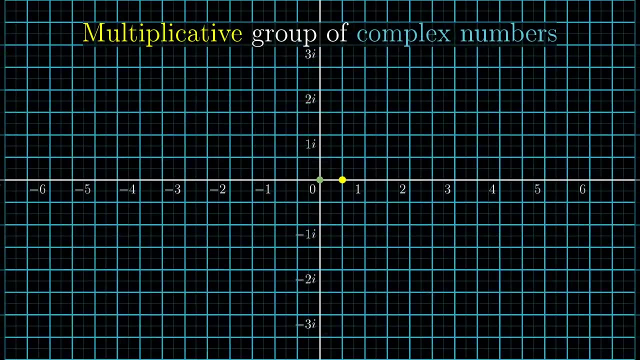 And we can also extend this idea to the complex plane. Again, I like to think of fixing zero in place with one hand and dragging around the point at one, keeping everything else evenly spaced while I do so, But this time as we drag the number one to places that are only 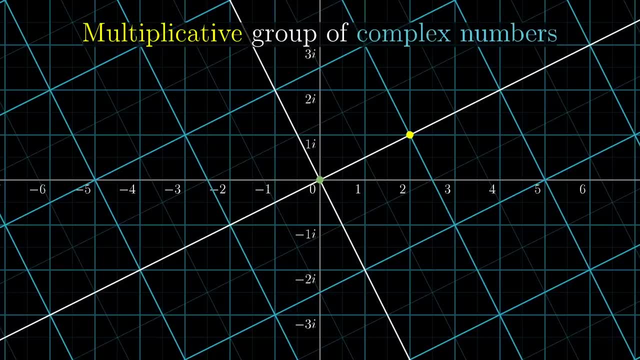 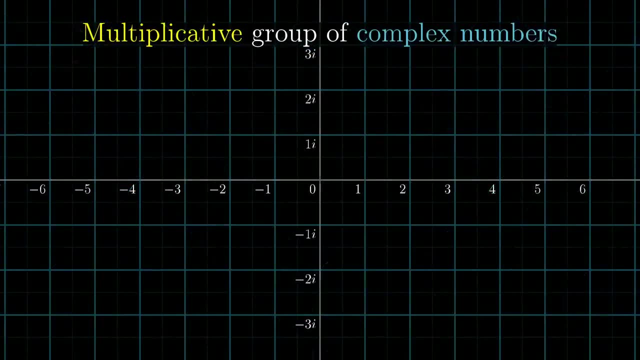 off the real number line, we see that our group includes not only stretching and squishing actions, but actions that have some rotational component as well. The quintessential example of this is the action associated with that point at i, one unit above zero. 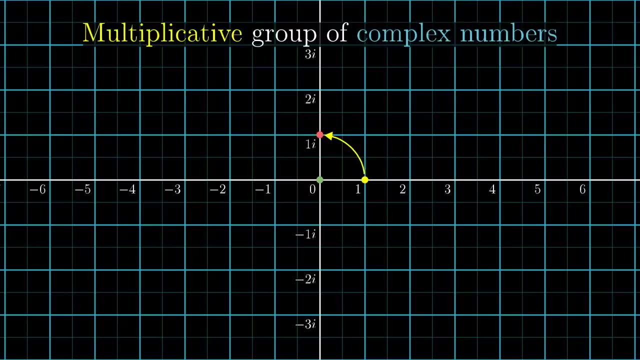 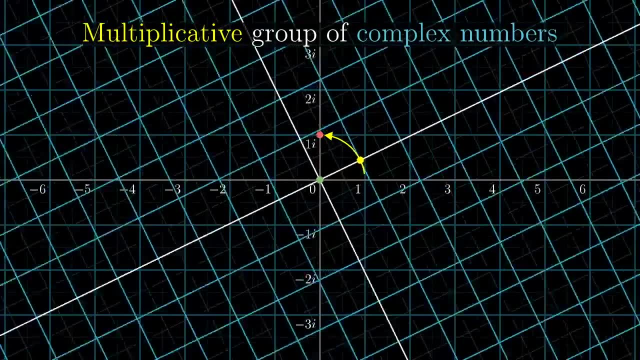 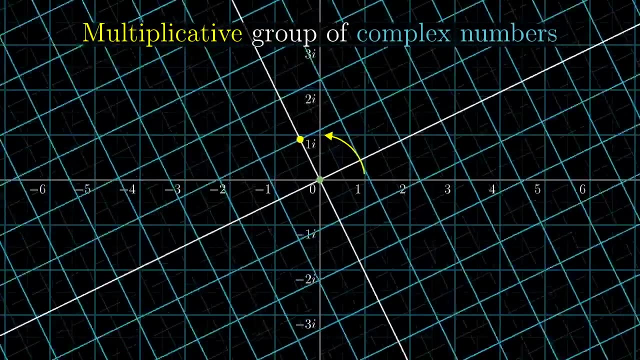 What it takes to drag the point at one to that point at i is a 90-degree rotation. So the multiplicative action associated with i is a 90-degree rotation. And notice, if I apply that action twice in a row, the overall effect is to flip the plane 180 degrees. 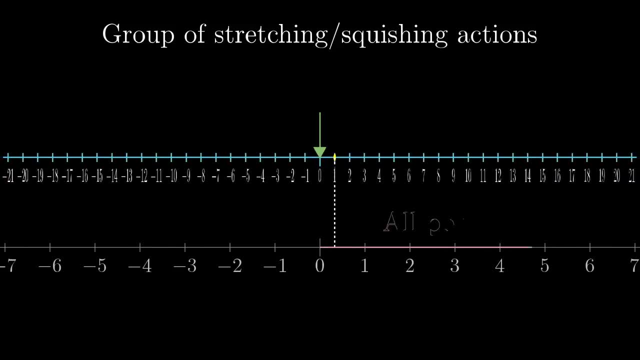 it takes to stay evenly spaced. In this way, every single positive number is associated with a unique stretching or squishing action. Now notice what composing actions looks like in this group. If I apply the stretch by 3 action and then follow it with the stretch by 2 action, the 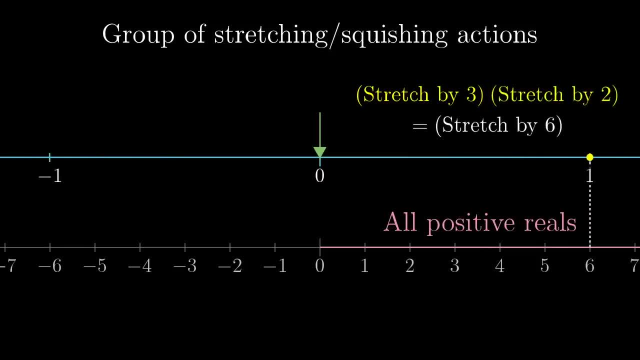 overall effect is the same as if I had just applied the stretch by 6 action, the product of the two original numbers. And in general, applying one of these actions followed by another corresponds with multiplying the numbers they are associated with. In fact, the name for this group is the multiplicative group of positive real numbers. 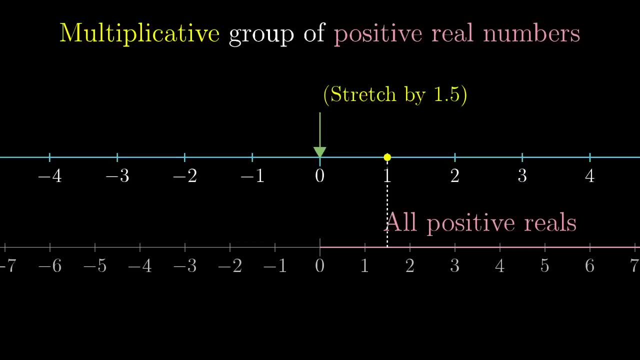 If I apply the stretch by 3 action and then follow it with the stretch by 2 action, the result is the same as if I had just applied the stretch by 3 action. So multiplication, ordinary familiar multiplication, is one more example of this very general and 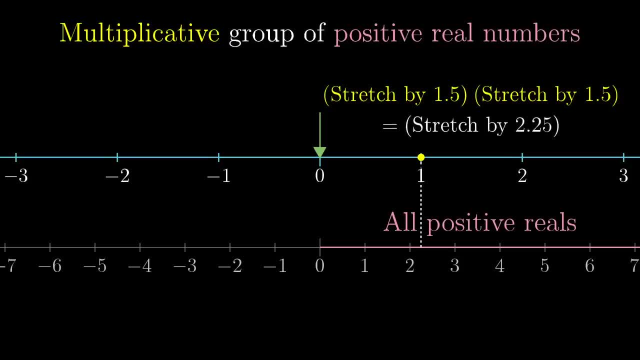 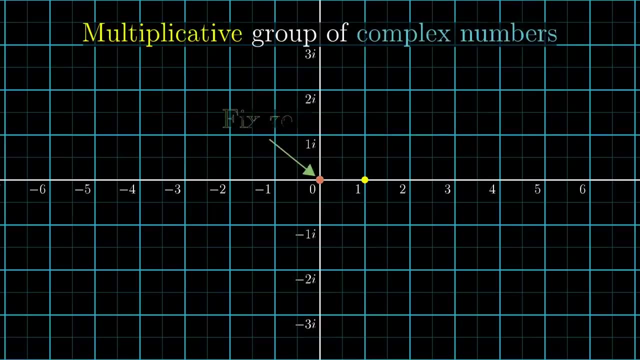 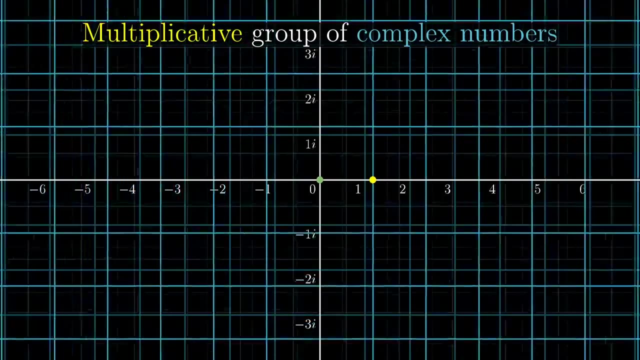 very far-reaching idea of groups and the arithmetic within groups, And we can also extend this idea to the complex plane. Again, I like to think of fixing zero in place with one hand and dragging around the point at 1, keeping everything else evenly spaced while I do so. But this time, as we drag the number 1 to places that are on the line, we can also extend the number 1 to places that are on the line. So if I apply the stretch by 3 action and then follow it with the stretch by 2 action, 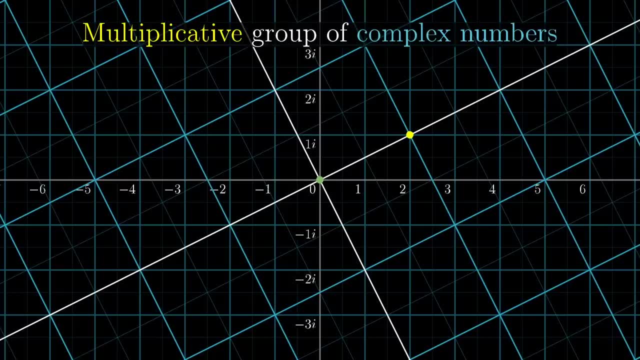 we can also extend the number 1 to places that are on the line, but that will also be front and back. And when we drag the blue point at 1 off the real number line, we see that our group includes not only stretching and squishing actions but actions that have some rotational component. 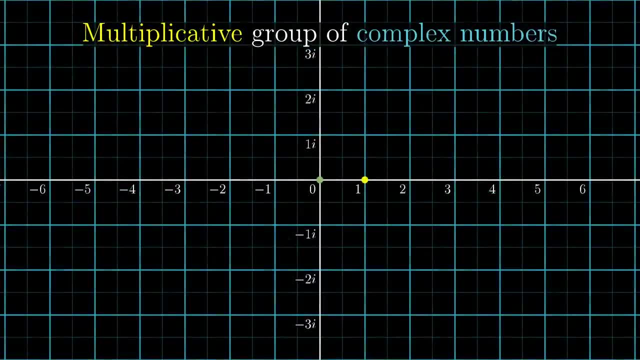 as well. The quintessential example of this is the action associated with that point at i, one unit above zero. What it takes to drag the point at 1 to that point at i is a 90 degree rotation. So the multiplicative action associated with i is a 90 degree rotation. 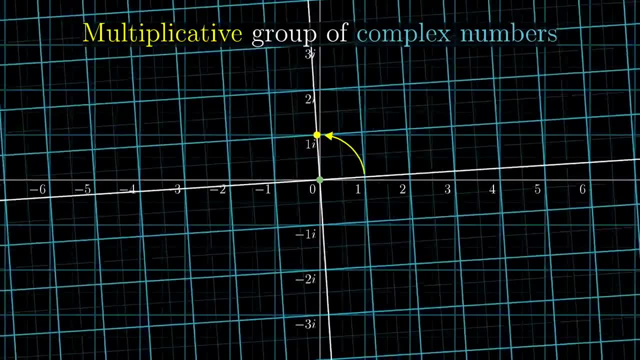 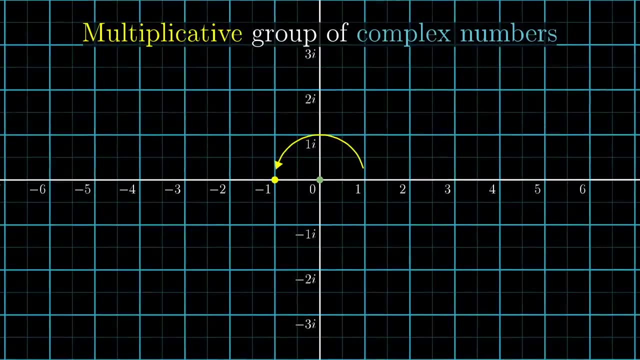 And notice, if I apply that action twice in a row, the overall effect is to flip the plane 180 degrees And that is the unique action that brings the point at 1 over to negative 1.. So in this sense, i times i equals negative 1, meaning the action associated with i followed. 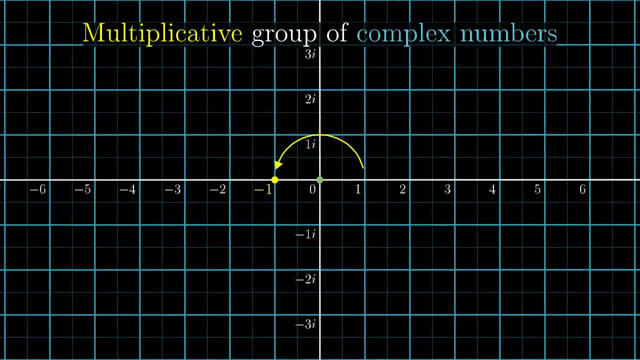 And that is the unique action that brings the point at one over to negative one. So in this sense, i times i equals negative one, meaning the action associated with i, followed by that same action associated with i, has the same overall effect as the action associated with negative one. 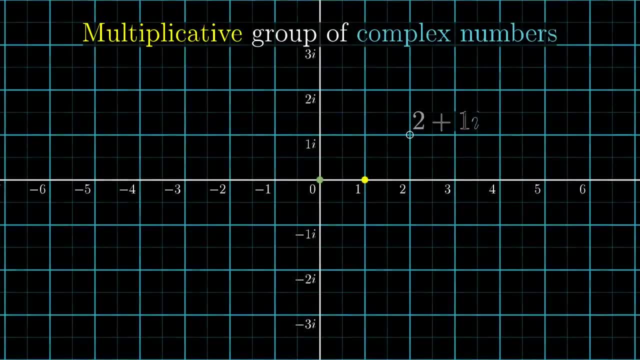 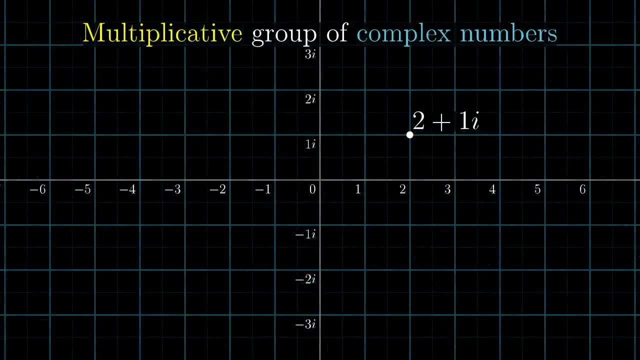 As another example, here's the action associated with 2 plus. i dragging one up to that point. If you want, you could think of this as broken down as a rotation by 30 degrees, followed by a stretch by a factor of square root of 5.. 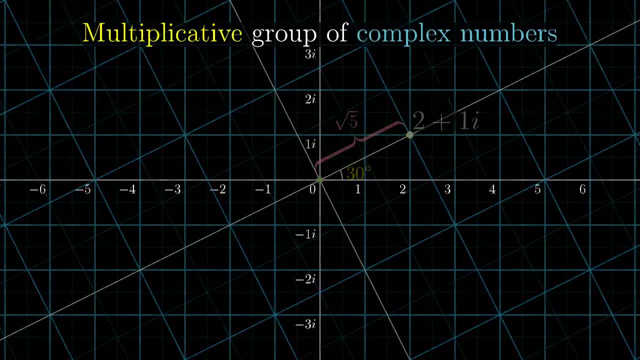 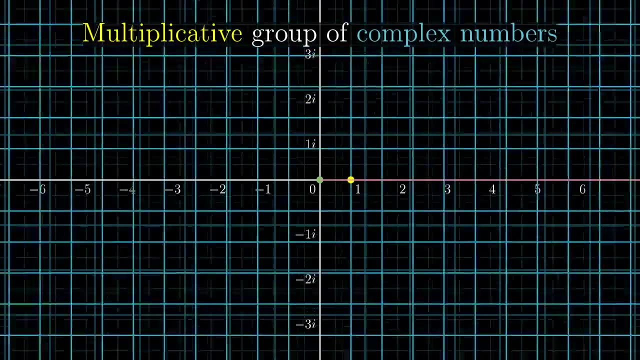 And, in general, every one of these multiplicative actions is some combination of a stretch or a squish, an action associated with some point on the positive real number line, followed by a pure rotation, Where pure rotations are associated with points on this circle, the one with radius 1.. 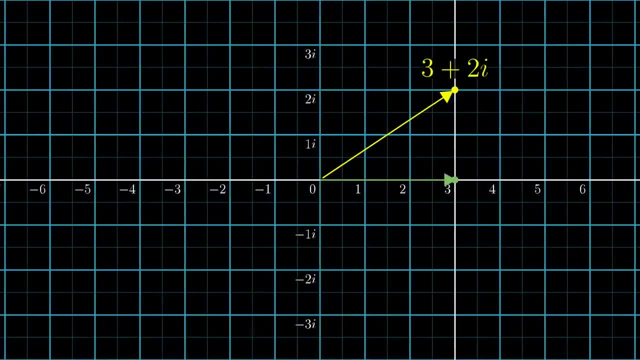 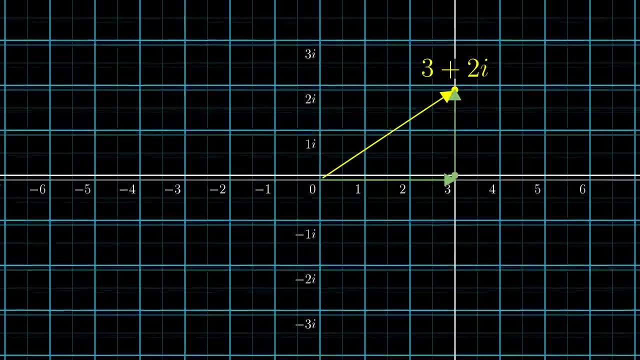 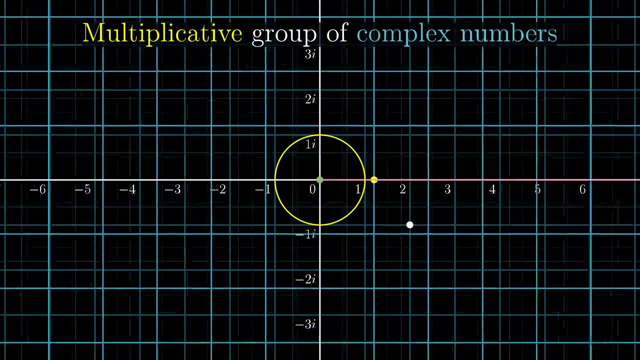 This is very similar to how the sliding actions in the additive group could be broken down as some pure horizontal slide, represented with points on the real number line, plus some purely vertical slide represented with points on that vertical line. That comparison of how actions in each group breaks down is going to be important, so remember it. 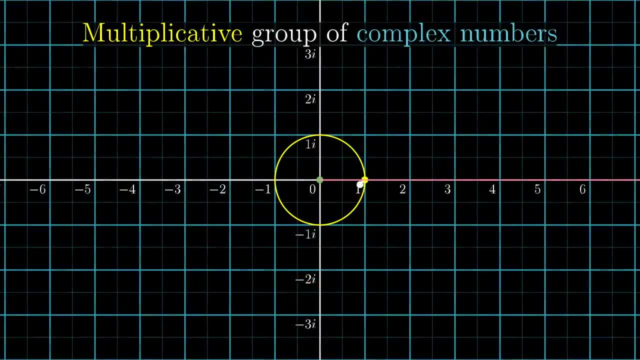 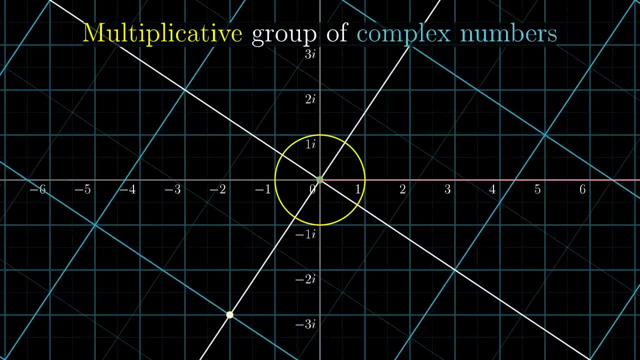 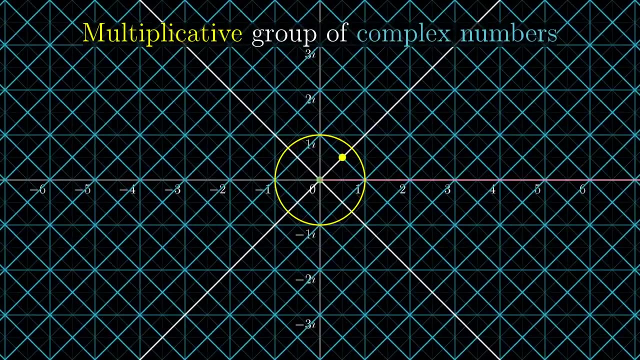 In each one. you can break down any action as some purely real number action, followed by something that's specific to complex numbers, whether that's vertical slides for the additive group or pure rotations for the multiplicative group. So that's our quick introduction to groups. 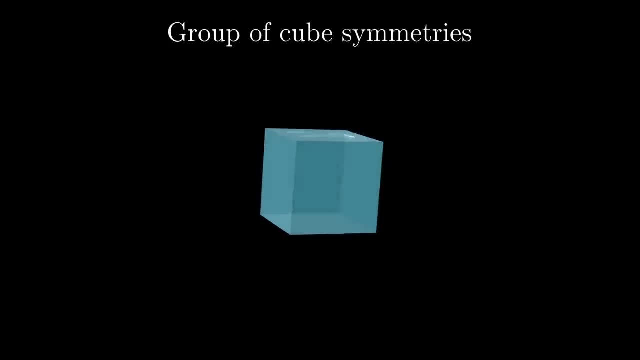 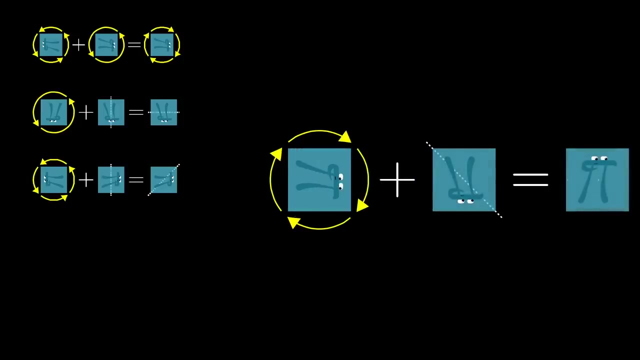 A group is a collection of symmetric actions on some mathematical object, whether that's a square, a circle, the real number line or anything else you dream up, And every group has a certain arithmetic where you can combine two actions by applying one after the other and asking what other action from the group gives the same overall effect. 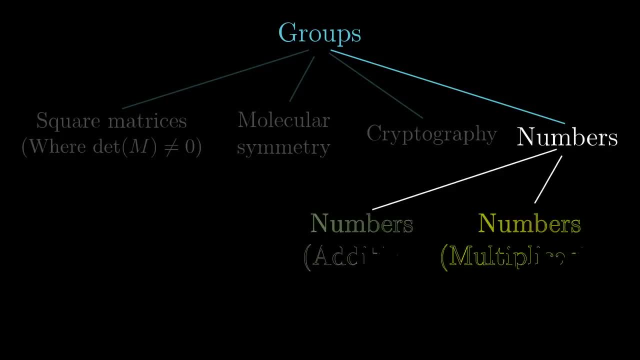 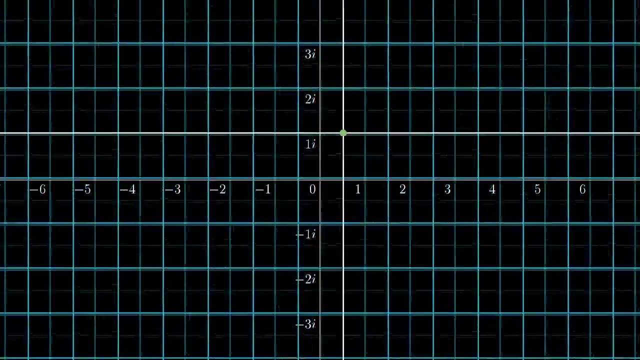 Numbers, both real and complex. numbers, can be thought of in two ways. as a group, They can act by sliding, in which case the group arithmetic just looks like ordinary addition. or they can act by this stretching, squishing, rotating actions, in which case 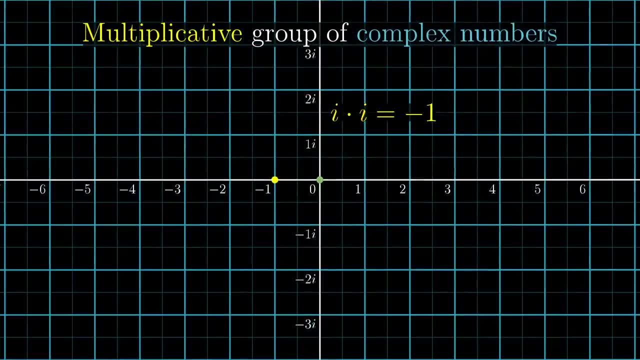 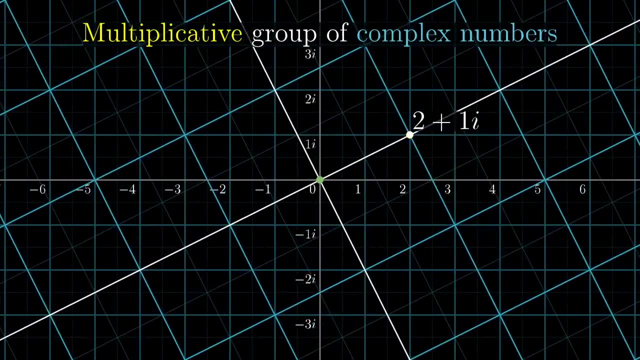 by that same action associated with i has the same overall effect as the action associated with negative 1.. As another example, here's the action associated with 2 plus i, dragging 1 up to that point. If you want, you could think of this as broken down as a rotation by 30 degrees followed. 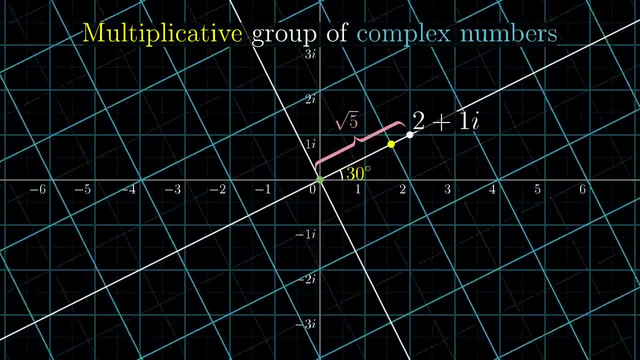 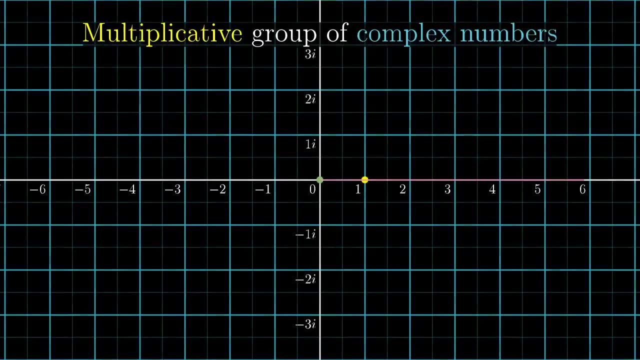 by a stretch, by a factor of square root of 5.. And, in general, every one of these multiplicative actions is some combination of a stretch or a squish, an action associated with some point on the positive real number line, followed by a pure rotation, where pure rotations are associated with points on this circle. 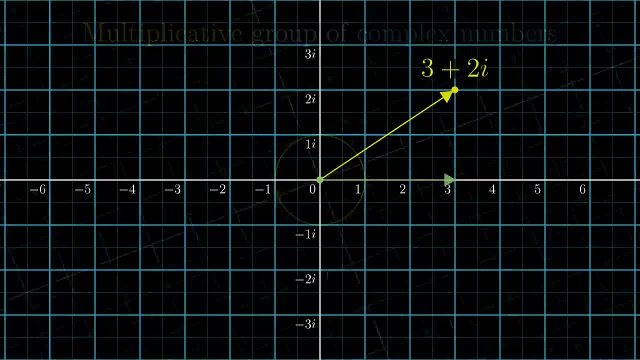 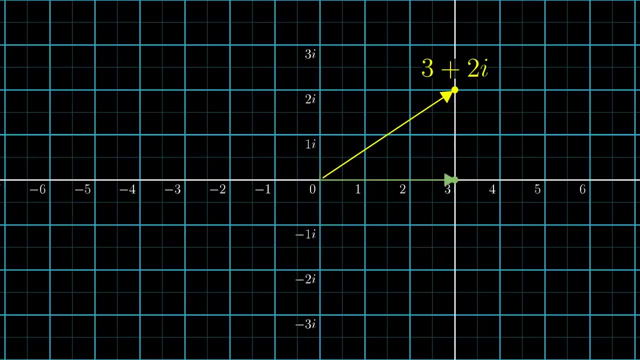 the one with radius 1.. This is very similar to how the sliding actions in the additive group could be broken down as some pure horizontal slide, represented with points on the real number line, plus some purely vertical slide represented with points on that vertical line. 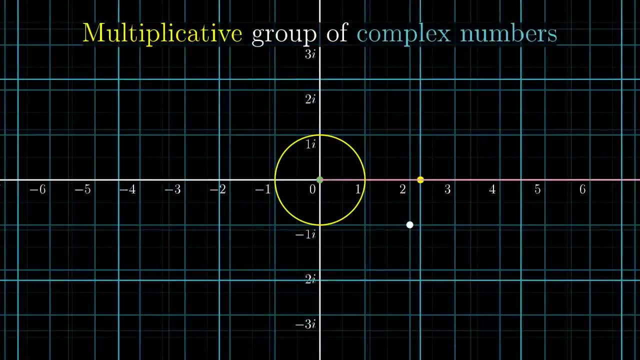 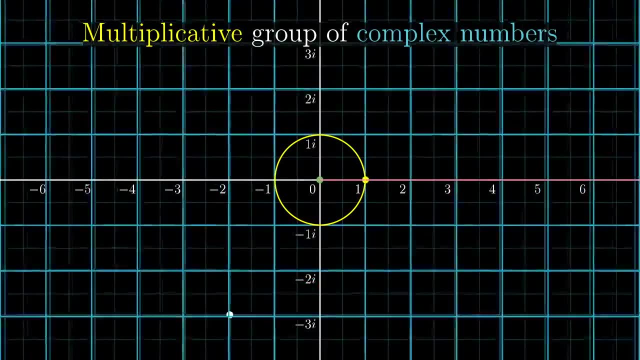 That comparison of how actions in each group breaks down is going to be important, so remember it. In each one, you can break down any action as some purely real number action, followed by something that's specific to complex numbers, whether that's vertical slides for the additive. 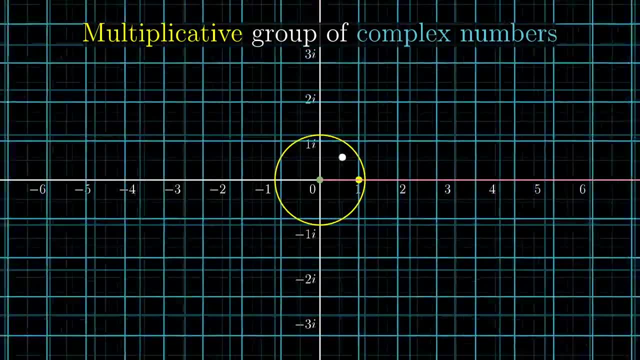 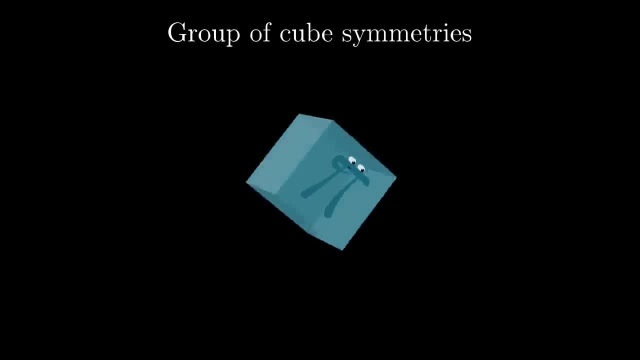 group or pure rotations for the multiplicative group. So that's our quick introduction to groups. A group is a collection of symmetric actions on some mathematical object, whether that's a square, a circle, the real number line or anything else you do. 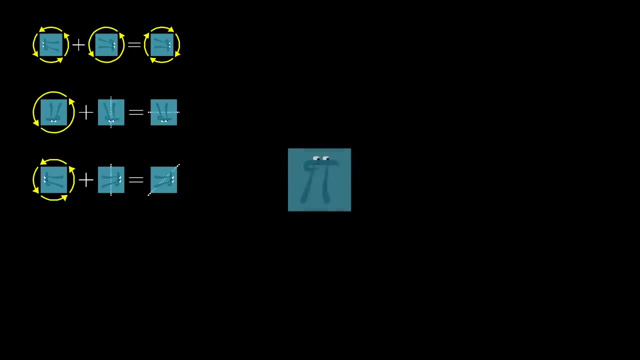 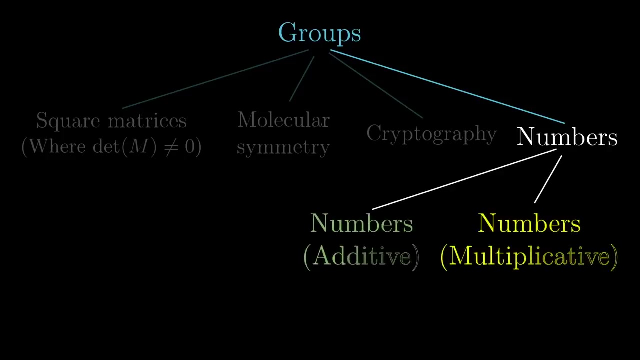 And every group has a certain arithmetic where you can combine two actions by applying one after the other and asking what other action from that group gives the same effect. Numbers, both real and complex numbers, can be thought of in two different ways as a group. 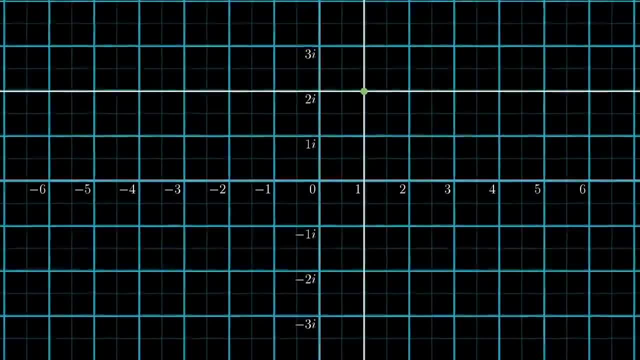 They can act by sliding, or by stretching, squishing and rotating actions in the case of the group arithmetic. Or they can act by sliding, in the case of the group arithmetic- in the case of the group arithmetic, or by strictly rotating actions. 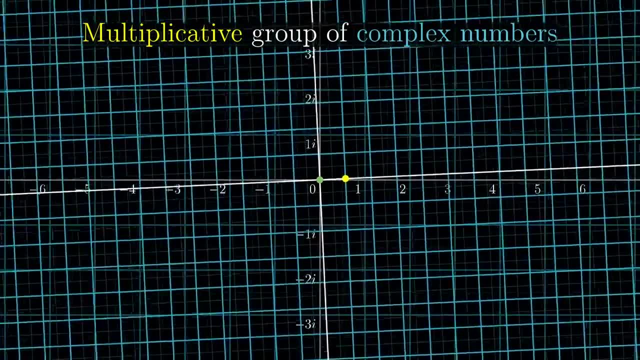 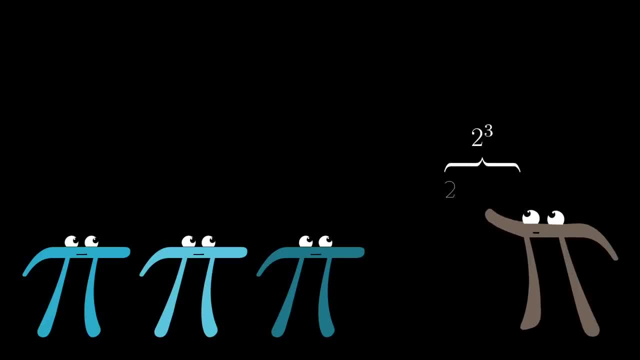 actions, in which case the group arithmetic looks just like multiplication. And with that, let's talk about exponentiation. Our first introduction to exponents is to think of them in terms of repeated multiplication. right, I mean, the meaning of something like 2 cubed is to take 2 times 2 times 2, and the meaning? 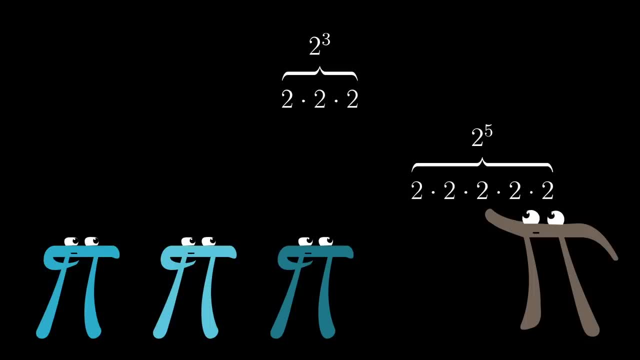 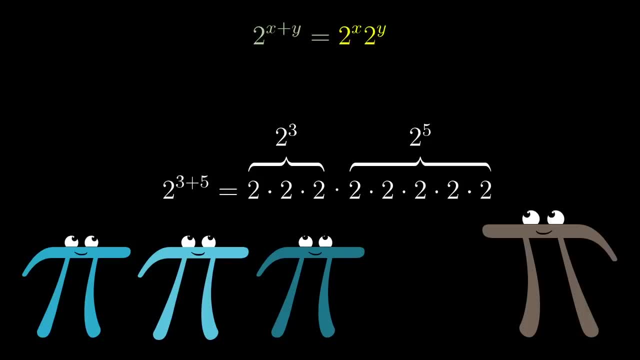 product of 2 to the third times 2 to the 5.. And when you expand things, this seems reasonable enough, right, But expressions like 2 to the one half or 2 to the negative 1, and much less 2 to the. 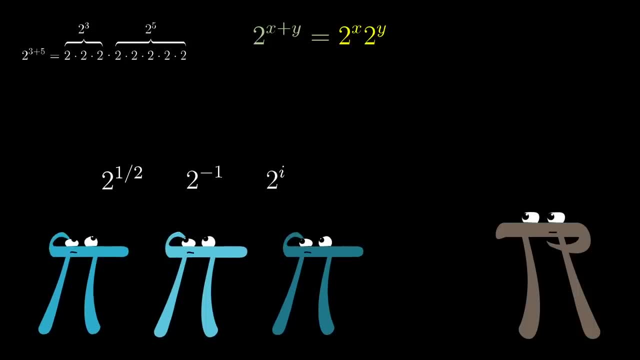 i don't really make sense when you think of exponents as repeated multiplication. I mean, what does it mean to multiply 2 by itself, half of a time, or negative one of a time? So we do something very common throughout math and extend beyond the original definition. 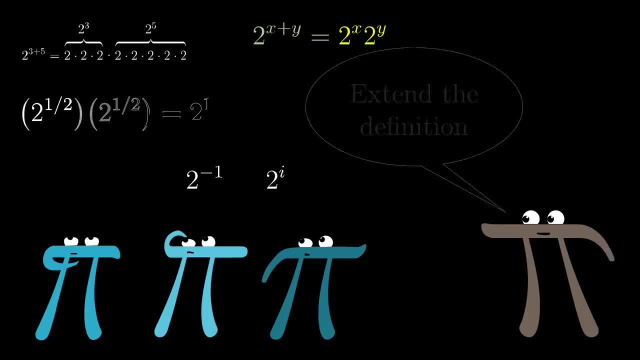 which only makes sense for counting numbers- to something that applies to all sorts of numbers. But we don't just do this randomly. If you think back to how fractional and negative exponents are defined, it's always motivated by trying to make sure that this property, 2 to the x plus y- equals 2 to the x plus y. 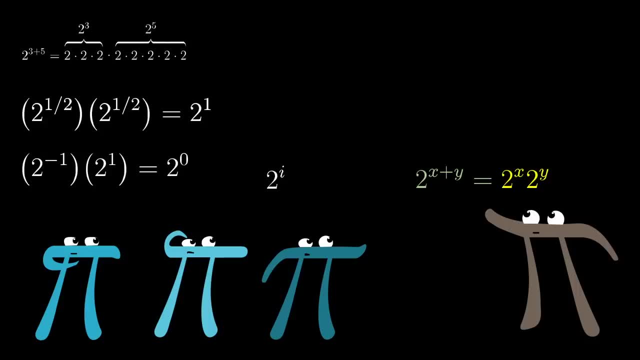 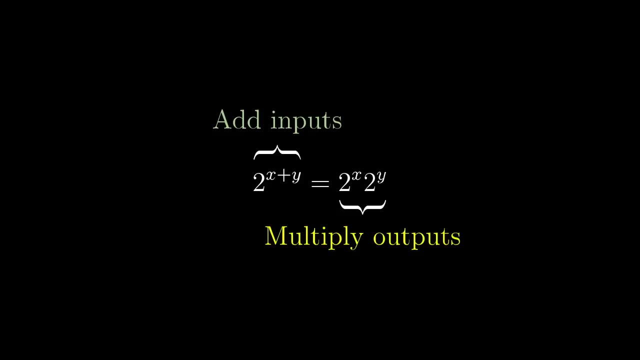 equals 2 to the x plus y. So what does this mean for complex exponents? Think about what this property is saying from a group theory light. It's saying that adding the inputs corresponds with multiplying the outputs, And that makes it very tempting to think of the inputs not merely as numbers, but as members. 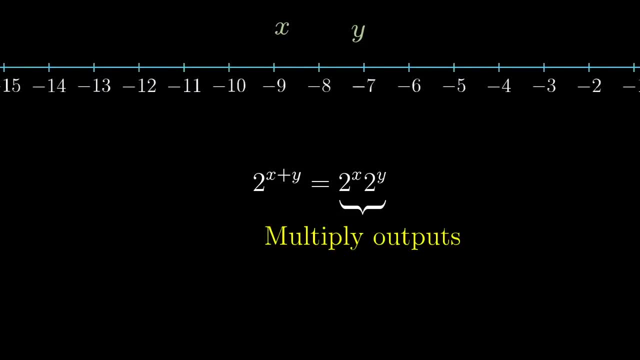 of the additive group of sliding actions. And to think of the outputs not merely as numbers but as members of this multiplicative group. And to think of the outputs not merely as numbers but as members of the additive group of sliding actions. And to think of the outputs not merely as numbers but as members of this multiplicative. 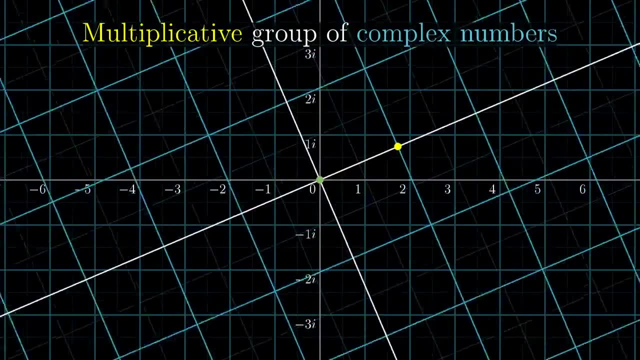 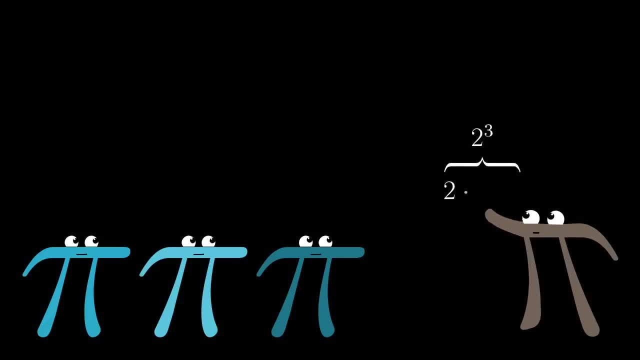 the group. arithmetic looks just like multiplication, And with that let's talk about exponentiation. Our first introduction to exponents is to think of them in terms of repeated multiplication, right, I mean, the meaning of something like 2 cubed is to take 2 times 2 times 2,. 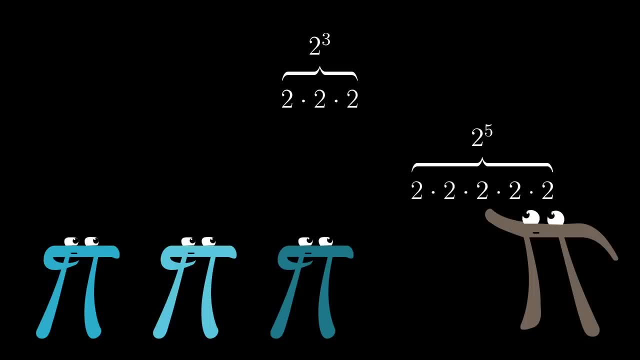 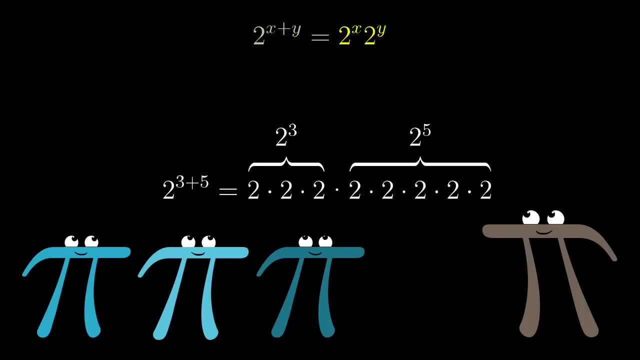 as the product of 2 to the third times 2 to the 5.. And when you expand things, this seems reasonable enough, right, But expressions like 2 to the one half, or 2 to the negative 1, and much less 2 to the, i don't really make sense when you think of. 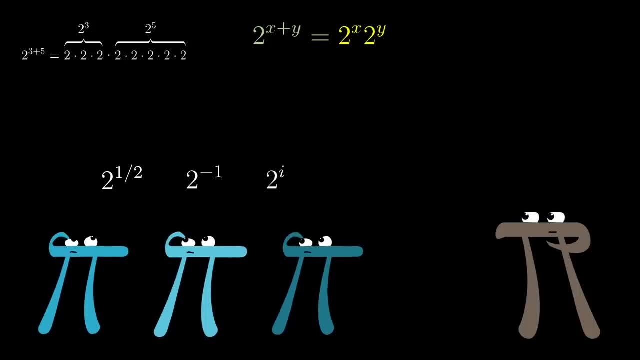 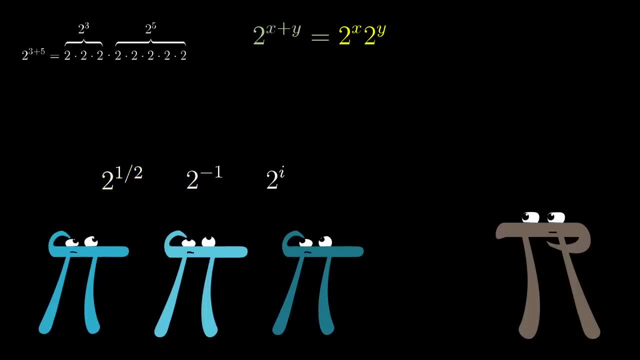 Half of a time or negative 1 of a time. So we do something very common throughout math and extend beyond the original definition, which only makes sense for counting numbers, to something that applies to all sorts of numbers. But we don't just do this randomly, If you think. 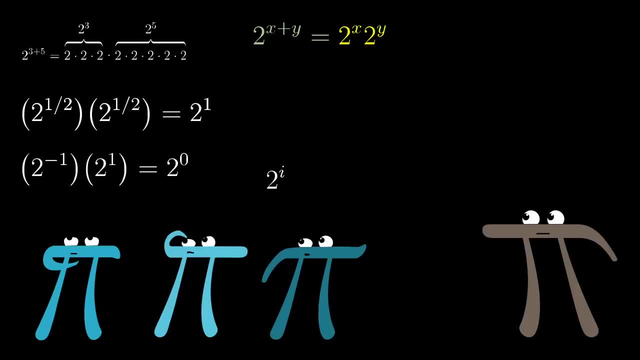 back to how fractional and negative exponents are defined. it's always motivated by trying to make sure that this property- 2 to the x plus y equals 2 to the x times 2 to the y- still holds To see what this might mean for complex exponents. think about what this property is saying from. 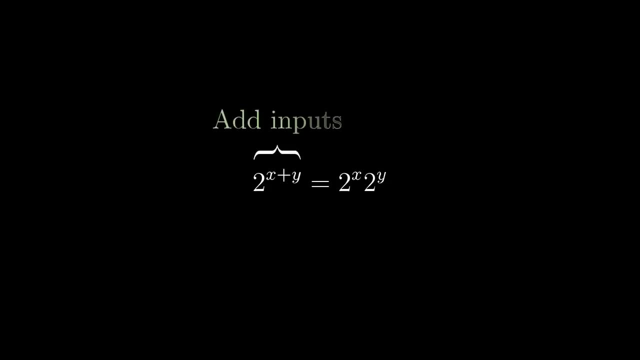 a group theory light. It's saying that adding the inputs corresponds with multiplying the outputs, and that makes it very tempting to think of the inputs not merely as numbers but as members of the additive group of sliding actions, and to think of the outputs not merely as numbers. 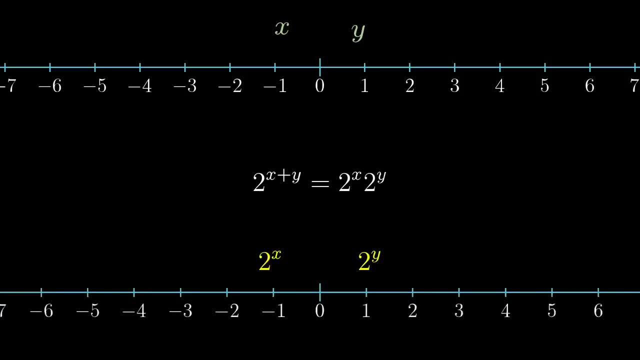 but as members of this multiplicative group of stretching and squishing actions. Now, it is weird and strange to think about functions that take in one kind of action and spit out another kind of action, but this is something that actually comes up all the time throughout group theory. 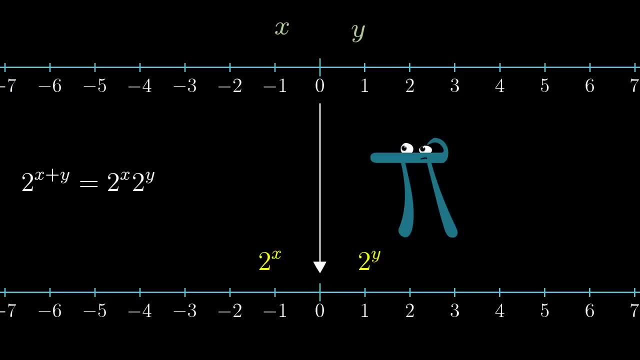 group. Now it is weird and strange to think about functions that take in one kind of action and spit out another kind of action, But this is something that actually comes up all the time throughout group theory, And this exponential property is very important for this association between groups. 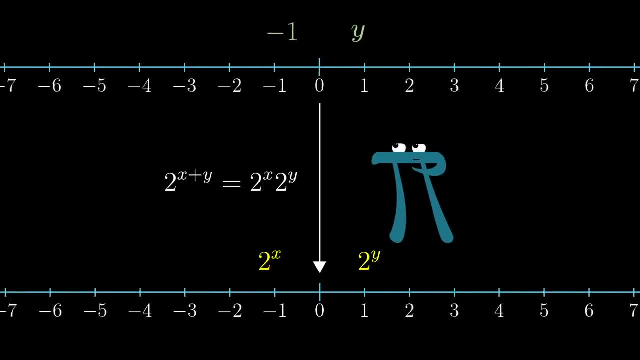 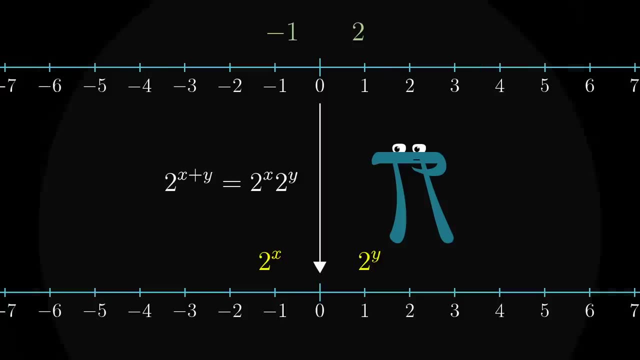 It guarantees that if I compose two sliding actions, maybe a slide by negative 1, and then a slide by positive 2. It corresponds to the number of numbers that I have. So what does this mean? It corresponds to composing the two output actions. 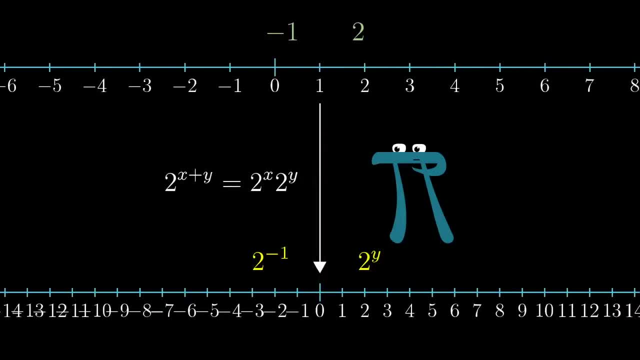 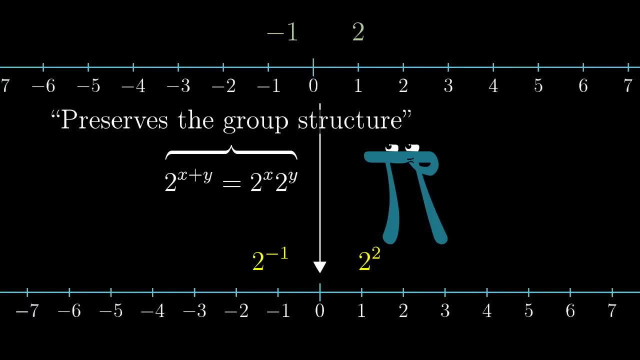 In this case squishing by 2 to the negative 1, and then stretching by 2. squared Mathematicians would describe a property like this by saying that the function preserves the group structure, in the sense that the arithmetic within a group is what gives it. 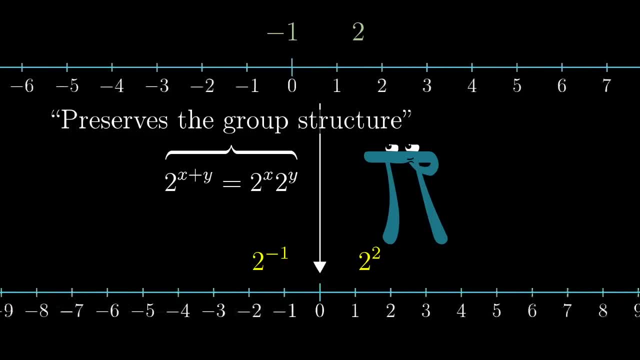 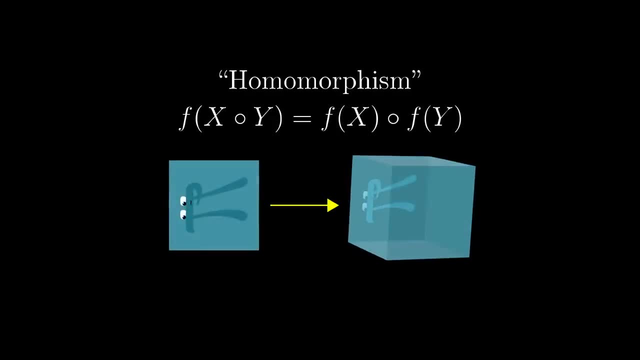 its structure, And a function like this, exponential, plays nicely with that arithmetic. So what does this mean? Well, it means that the arithmetic within a group is what gives it its structure. Functions between groups that preserve the arithmetic like this are really important throughout group theory, enough so that they've earned themselves a nice fancy name: homomorphisms. 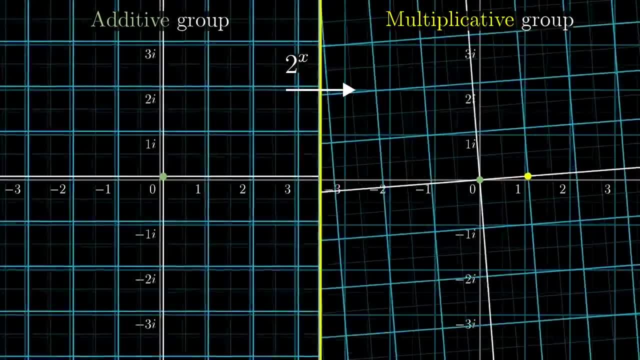 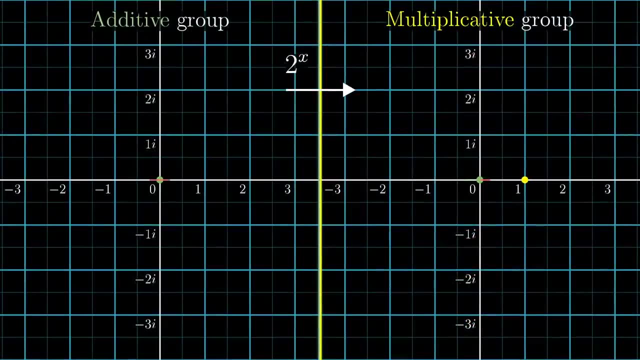 Now think about what all of this means for associating the additive group in the complex plane with the multiplicative group in the complex plane. We already know that when you plug in a real number to 2, to the x, you get out a real number. 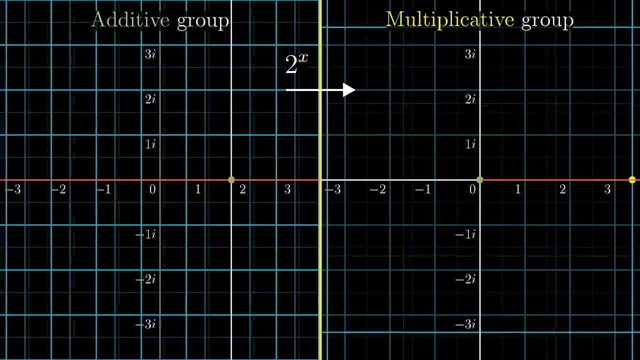 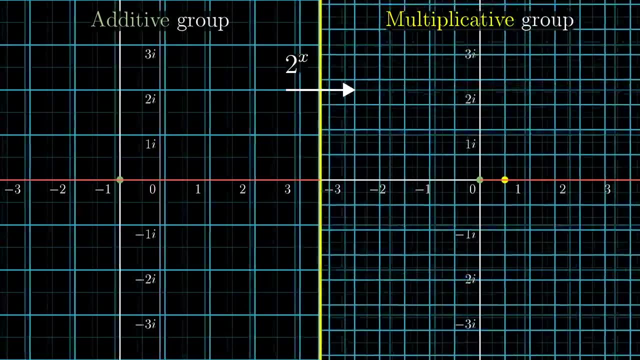 A positive real number, in fact. So this is a real number. This exponential function takes any purely horizontal slide and turns it into some pure stretching or squishing action. So wouldn't you agree that it would be reasonable for this new dimension of additive actions? 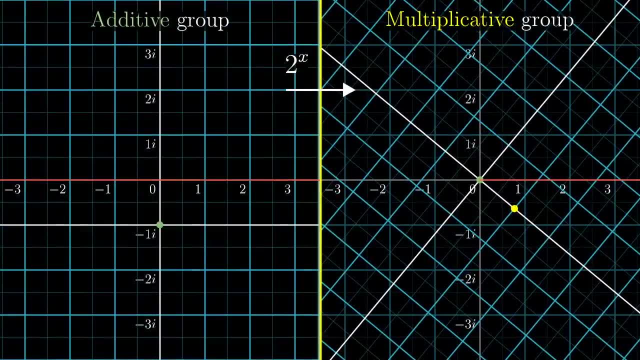 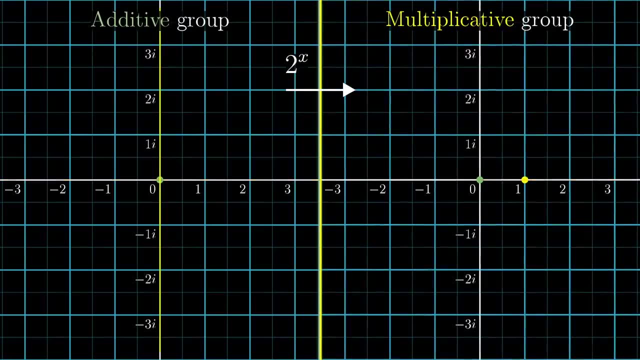 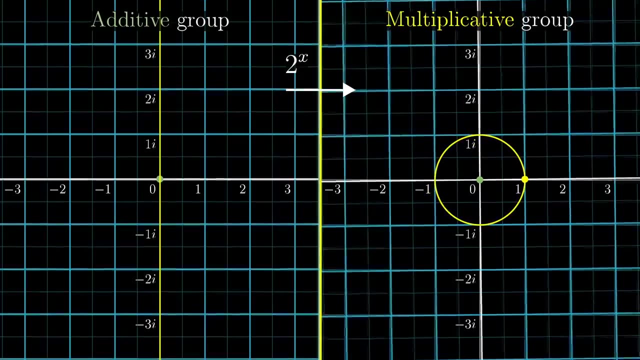 slides up and down to map directly into this new dimension of multiplicative actions: pure rotations. Those vertical sliding actions correspond to points on this vertical axis and those rotating multiplicative actions correspond to points on this vertical axis. Those rotating multiplicative actions correspond to points on the circle with radius 1.. 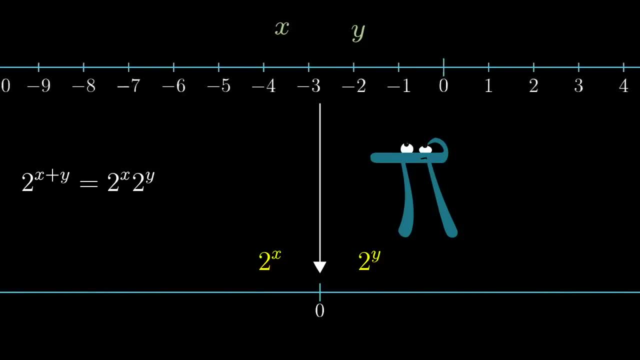 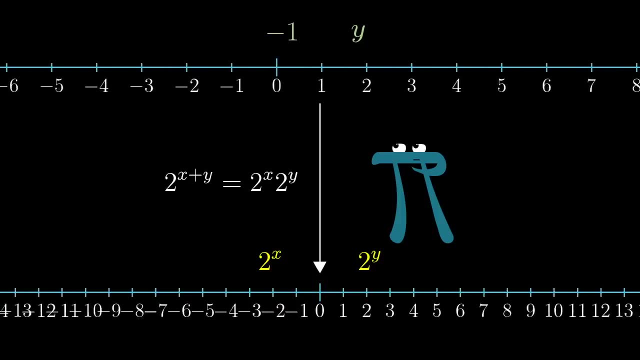 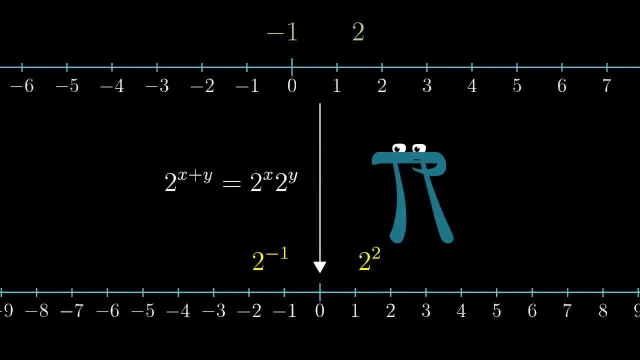 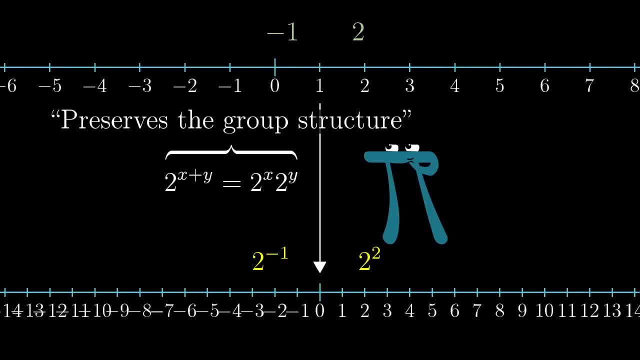 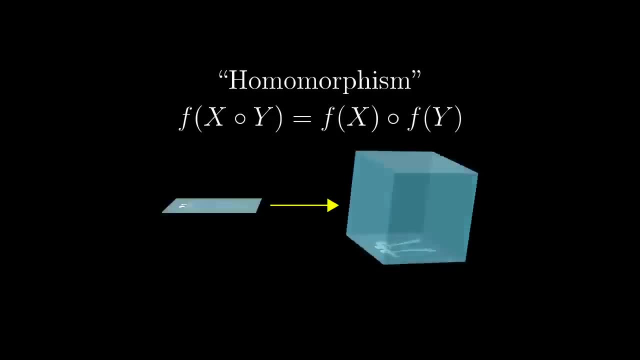 is what gives it its structure, and a function like this exponential plays nicely with that arithmetic. Functions between groups that preserve the arithmetic like this are really important throughout group theory, enough so that they've earned themselves a nice fancy name: homomorphisms. 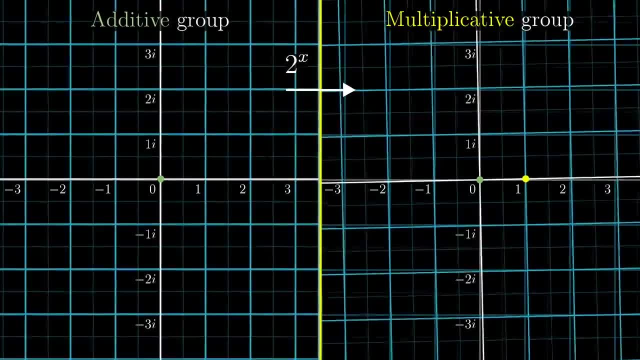 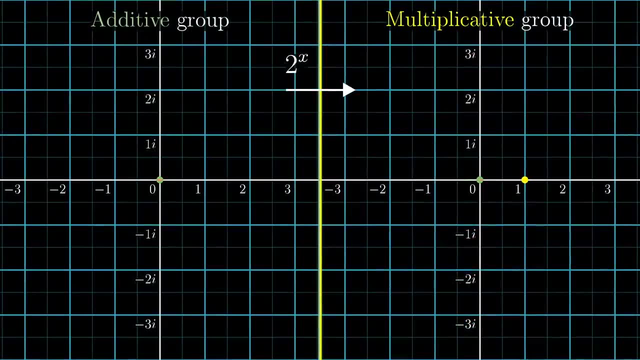 Now think about what all of this means for associating the additive group in the complex plane with the multiplicative group in the complex plane. We already know that when you plug in a real number to 2, to the x, you get out a real number, a positive real number in fact. 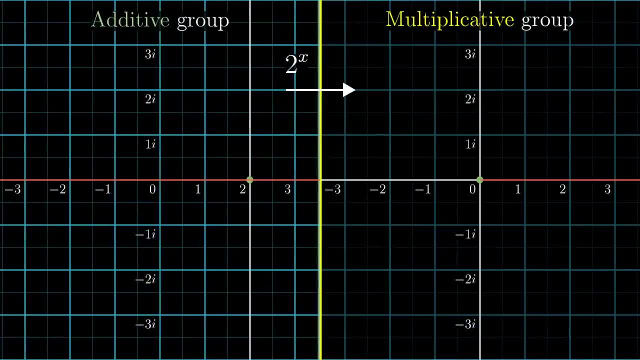 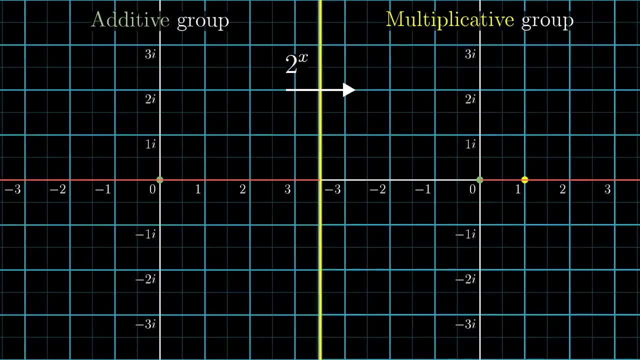 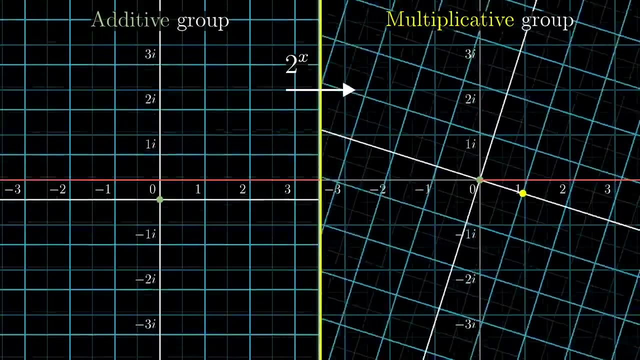 So this exponential function takes any purely horizontal slide and turns it into some pure stretching or squishing action. So wouldn't you agree that this would be reasonable for this new dimension of additive actions slides up and down to map directly into this new dimension of? 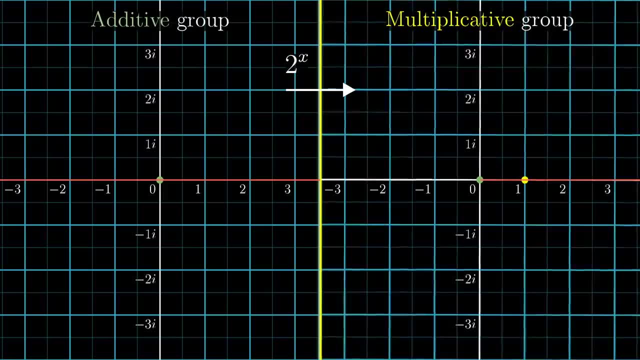 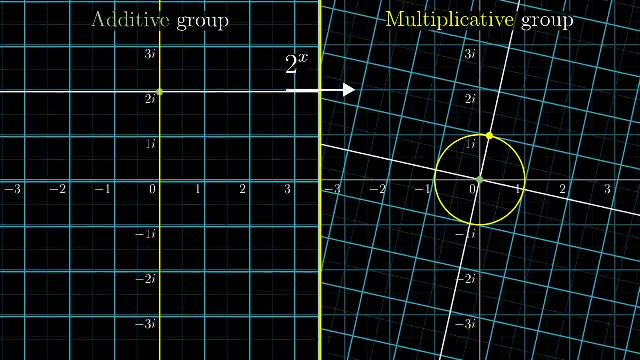 multiplicative actions, pure rotations. Those vertical sliding actions correspond to points on this vertical axis and those rotating multiplicative actions correspond to points on the circle with radius 1.. What it would mean for an exponential function like 2 to the x to map purely vertical slides into pure rotations. 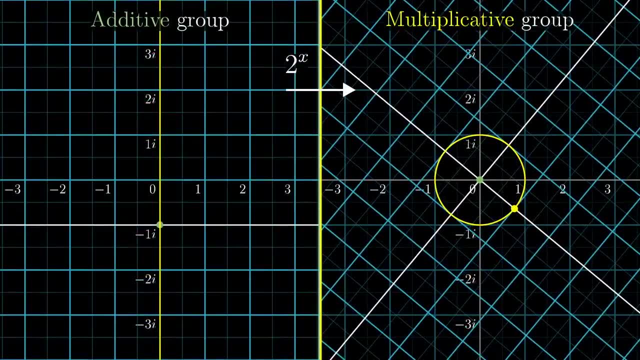 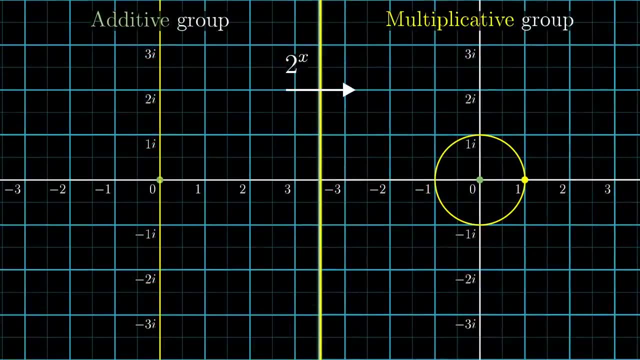 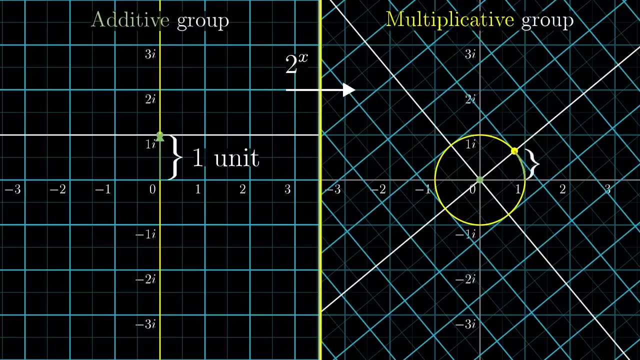 would be that complex numbers on this vertical line, multiples of i, get mapped to complex numbers on this unit circle. In fact, for the function 2 to the x, the input i, a vertical slide of one unit, happens to map to a rotation of about. 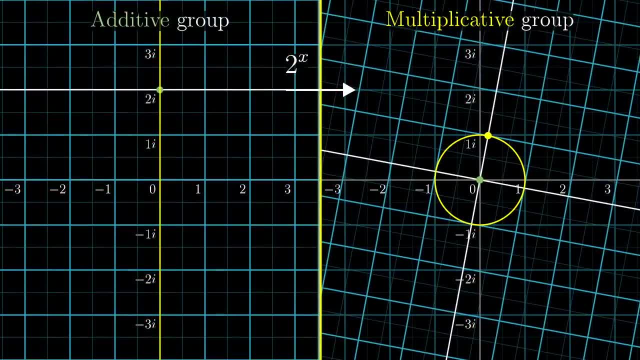 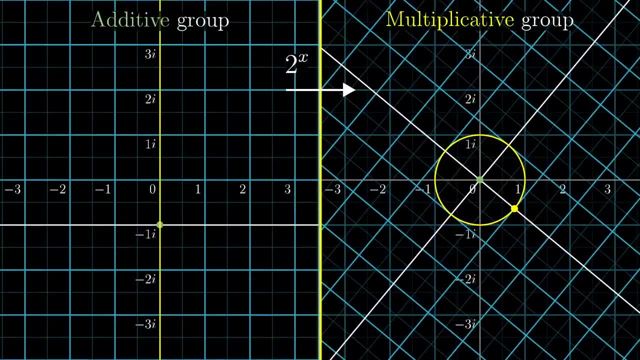 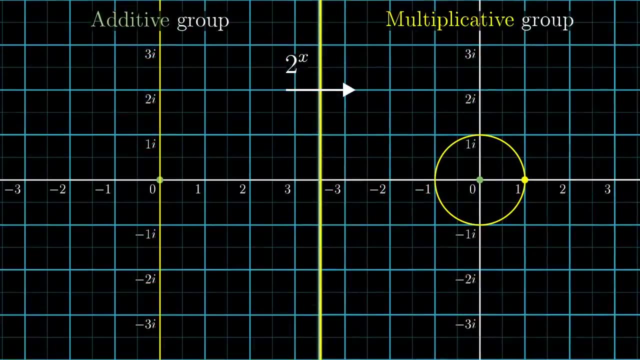 So what it would mean for an exponential function like 2 to the x to map purely vertical slides into pure rotations would be that complex numbers on this vertical line, multiples of i- get mapped to complex numbers on this unit circle. In fact, for the function 2 to the x, the input i, a vertical slide of one unit happens. 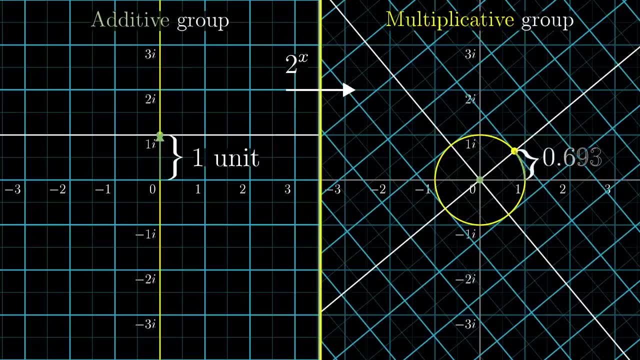 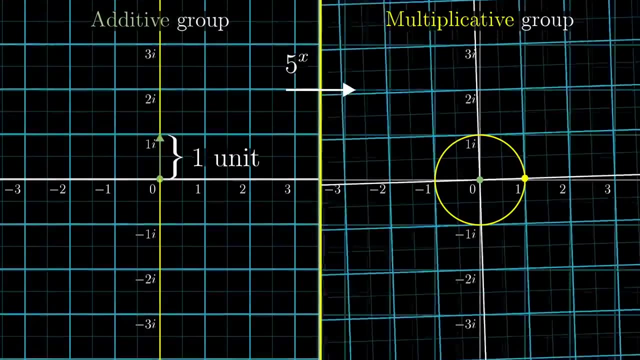 to map to a rotation of about 0.693 radians. That is a walk around the unit circle that covers 0.693 units of distance With a different exponential function, say 5 to the x. that input i a vertical slide. 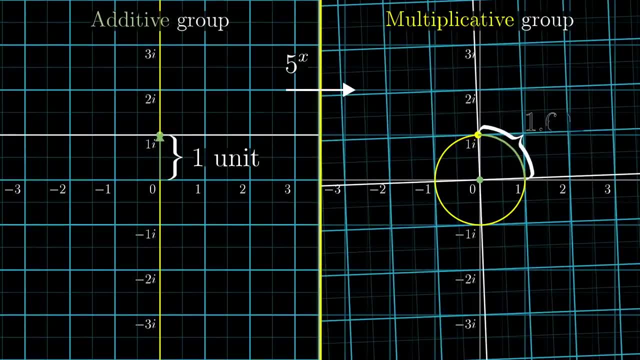 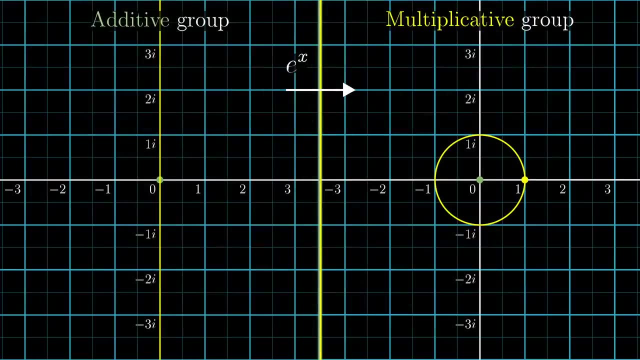 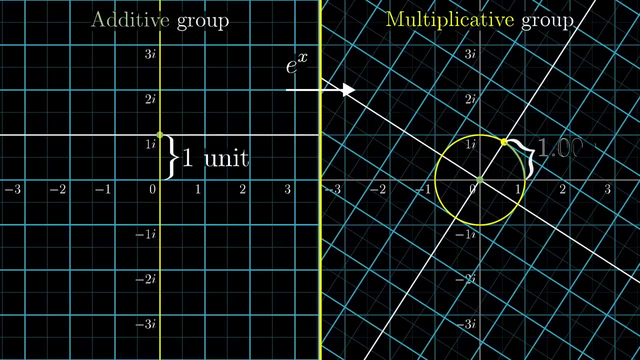 of one unit would map to a rotation of about 1.609 radians, a walk around the unit circle covering exactly 1.609 units of distance. This makes the number e special because when the exponential e to the x maps vertical slides to rotations, a vertical slide of one unit corresponding to i maps to a rotation. 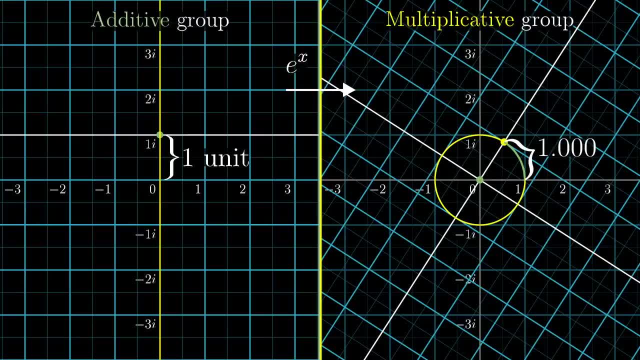 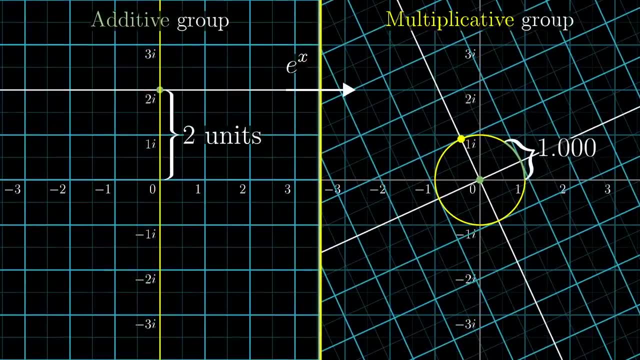 of exactly 1 radian, a walk around the unit circle covering a distance of exactly 1.. So a vertical slide of 2 units would map to a rotation of 2 radians. a 3 unit slide up would map to a rotation of 3 radians. 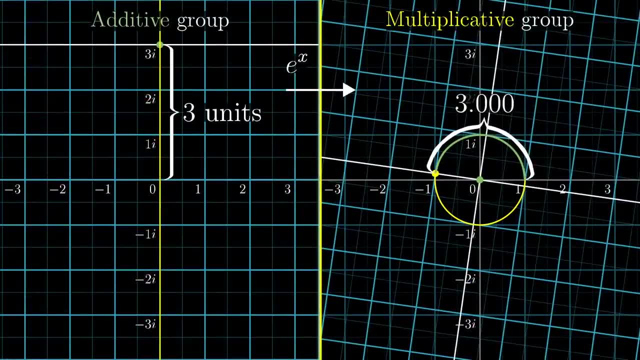 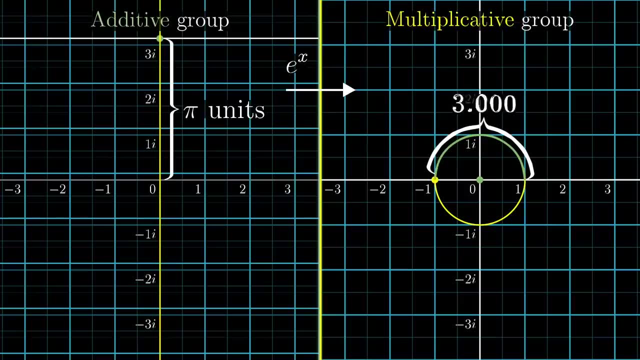 The vertical slide of 2 units would map to a rotation of 2 radians. a 3 unit slide up would map to a rotation of 3 radians And a vertical slide of exactly pi units up corresponding to the input pi times i maps. 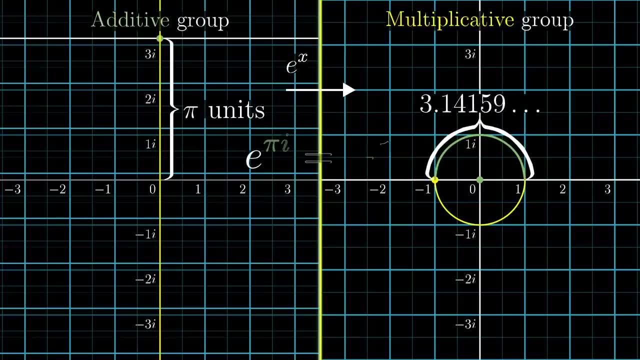 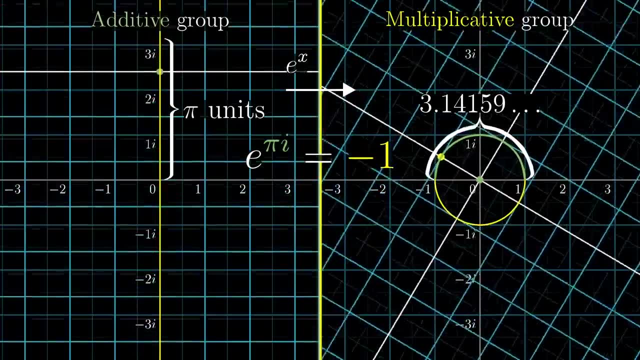 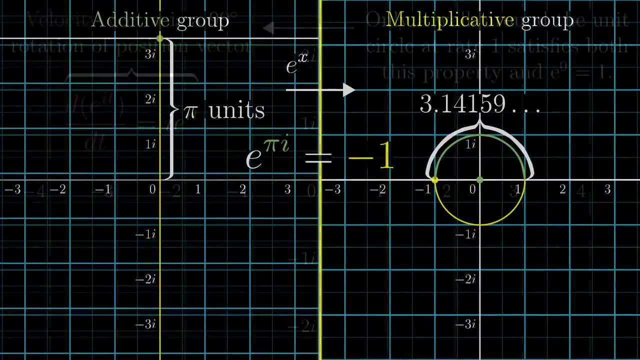 to a rotation of exactly pi radians halfway around the circle, And that's the multiplicative action associated with the number negative 1.. Now you might ask: why e? Why not some other base? The full answer resides in calculus. that's the birthplace of e and where it's even. 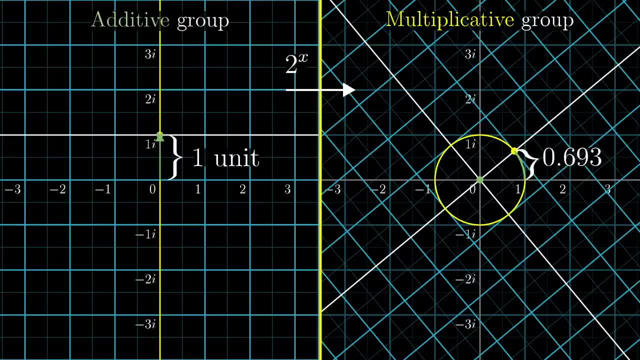 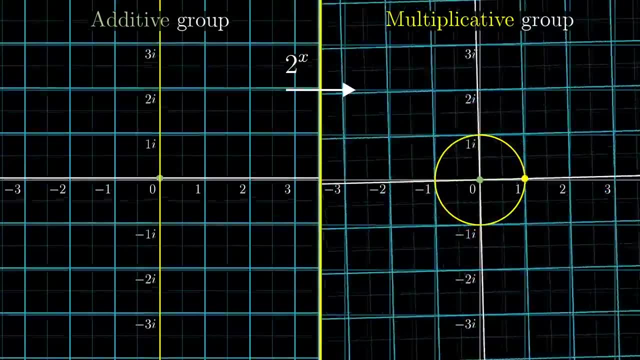 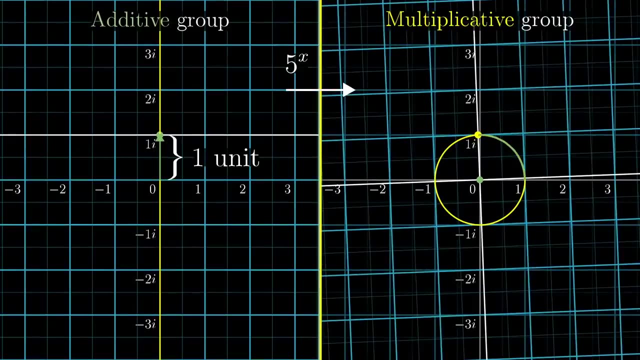 0.693 radians. that is a walk around the unit circle that covers 0.693 units of distance With a different exponential function, say 5 to the x. that input i, a vertical slide of one unit, would map to a rotation of about 1.609 radians a walk. 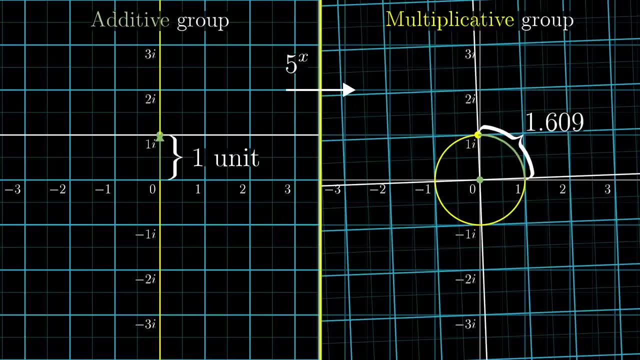 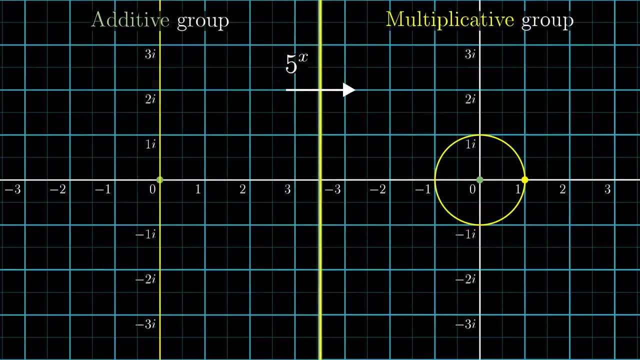 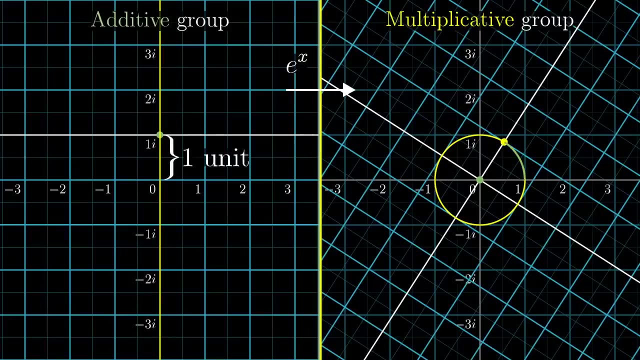 around the unit circle covering exactly 1.609 units of distance. What makes the number e so important is the fact that the number of radians on the x-axis is an integral, but when the exponential e to the x maps vertical slides to rotations. a vertical slide of 1 unit corresponding to i maps to a rotation of 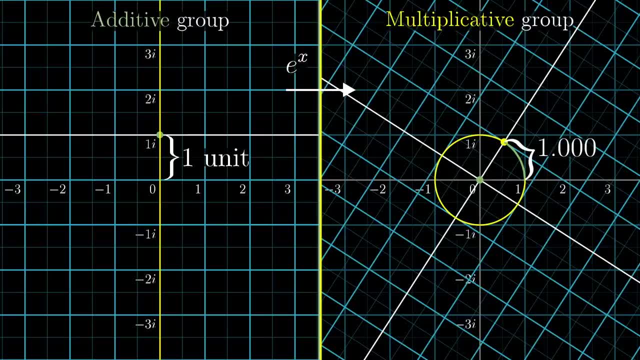 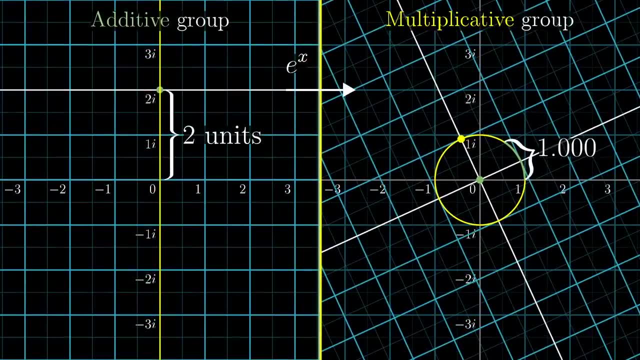 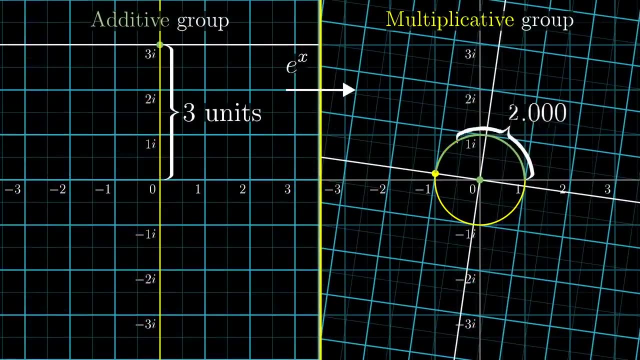 exactly 1 radian, a walk around the unit circle covering a distance of exactly 1.. So a vertical slide of 2 units would map to a rotation of 2 radians. a three unit slide up corresponds to a rotation of 3 radians and a vertical slide of a. 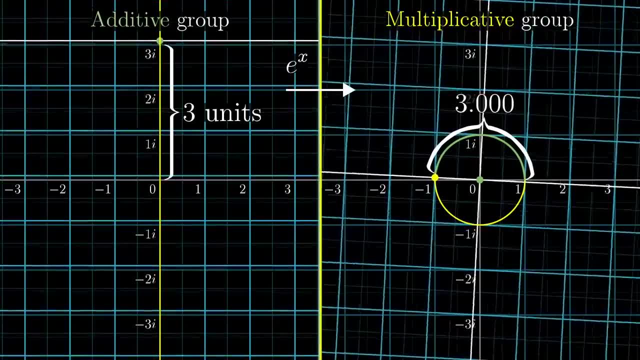 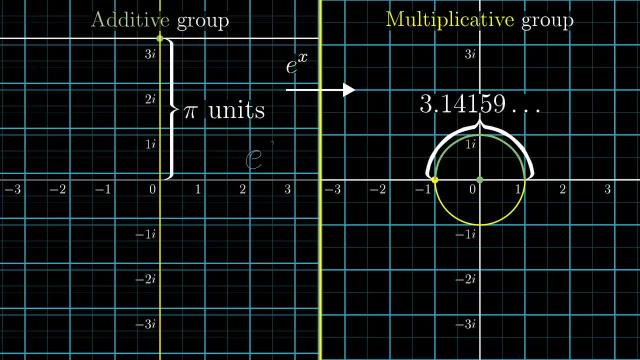 three unit slide up corresponds to a rotation of 3 radians. It is queda valid. The vertical slide of exactly pi units up corresponding to the input pi times. i maps to a rotation of exactly pi radians halfway around the circle And that's the multiplicative action associated with the number negative 1.. 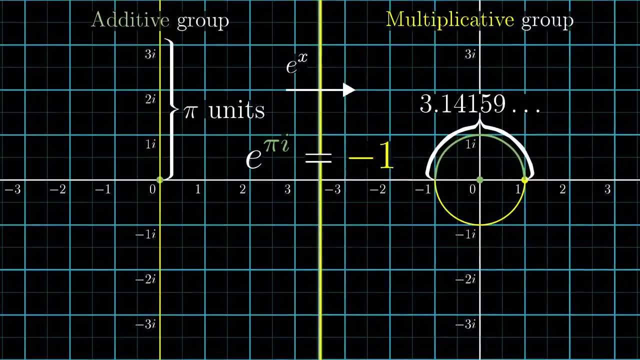 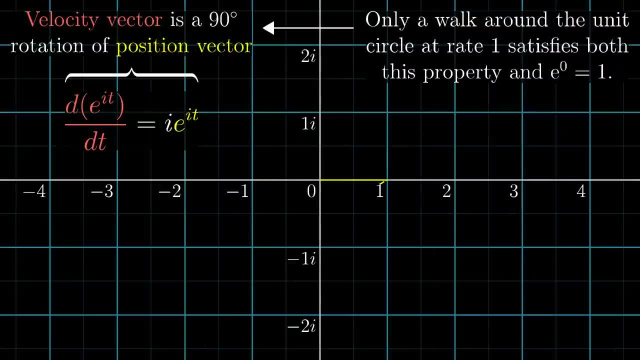 Now you might ask: why E? Why not some other base? Well, the full answer resides in calculus. that's the birthplace of E and where it's even defined. Again, I'll leave up another explanation on the screen if you're hungry for a fuller. 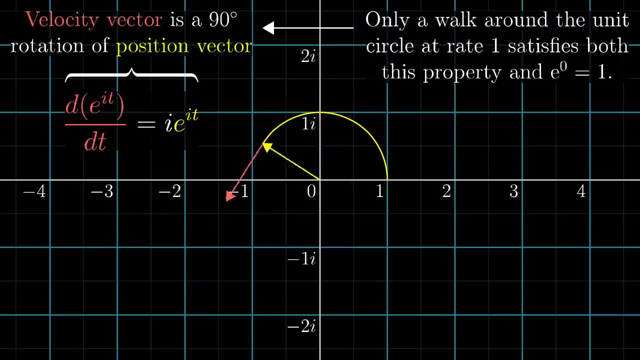 description and if you're comfortable with the calculus, but at a high level, I'll say that it has to do with the fact that all exponential functions are proportional to their own derivative, but E to the x alone is the one that's actually equal to its own derivative. 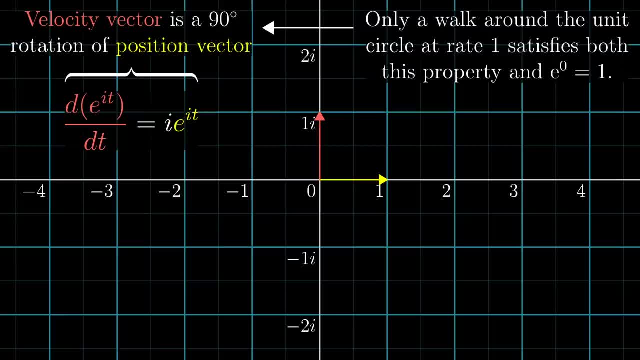 defined. There's another explanation on the screen. if you're hungry for a fuller description and if you're comfortable with calculus, But at a high level, I'll say it has to do with the fact that all exponential functions are proportional to their own derivative, but e to the x alone is the one that is actually. 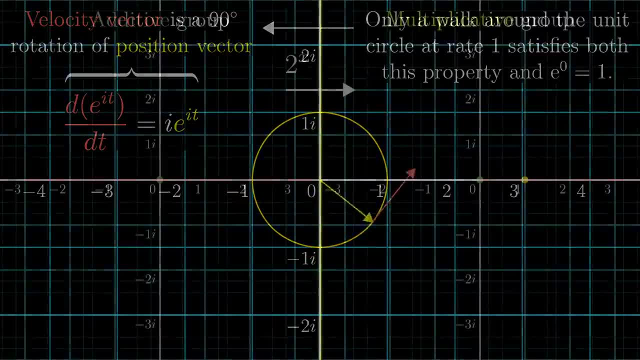 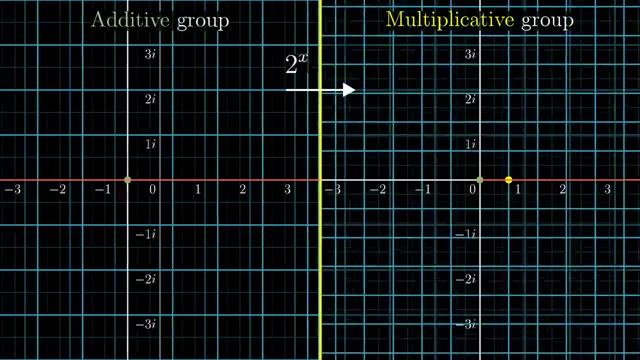 equal to its own derivative. The important point I want to make here is that if you view things from the lens of group theory- thinking of the inputs to an exponential function as sliding actions and thinking of the outputs as sliding actions- you wouldn't have a group theory in your mind. 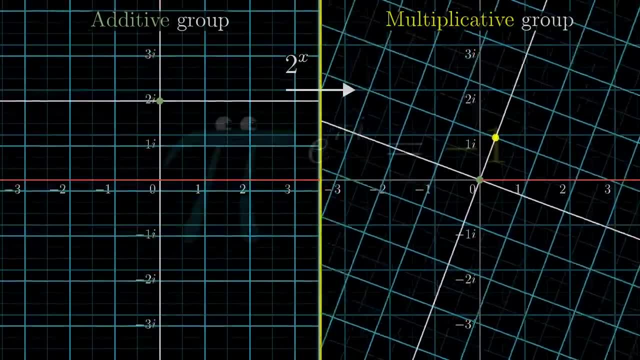 If you think of the inputs to an exponential function as sliding actions and thinking of the outputs as sliding actions, you wouldn't have a group theory in your mind as stretching and rotating actions. it gives a very vivid way to read what a formula like this: 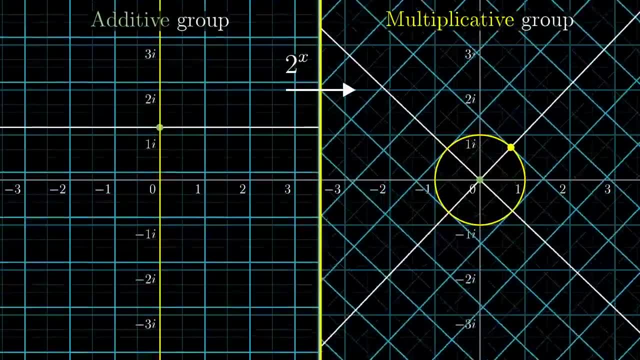 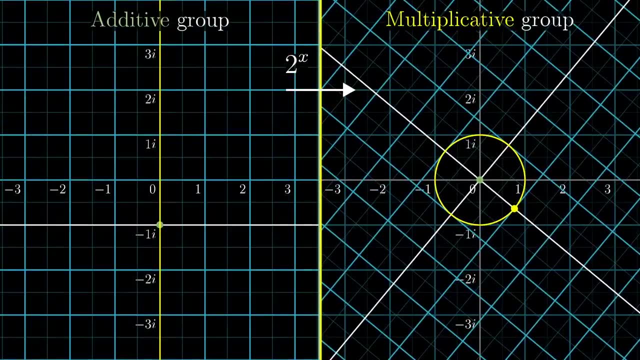 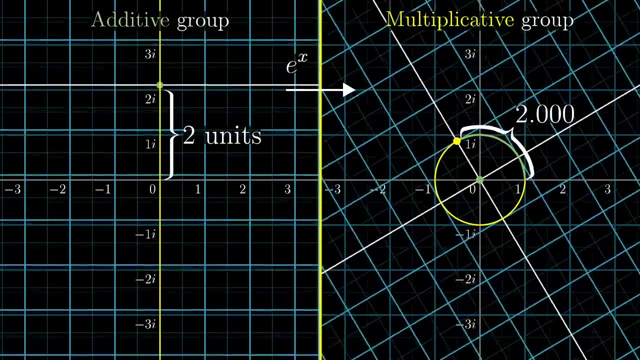 is even saying. When you read it you can think that exponentials in general map purely vertical slides, the additive actions that are perpendicular to the real number line into pure rotations which are in some sense perpendicular to the real number stretching actions And, moreover, 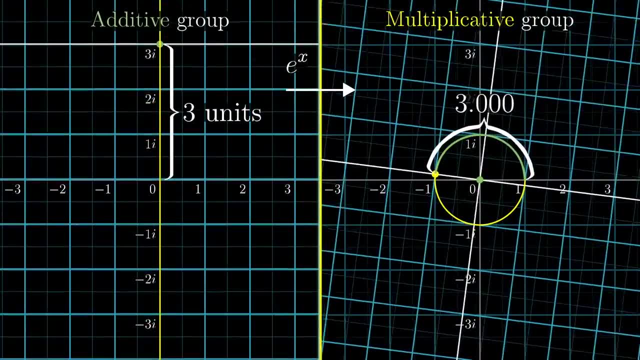 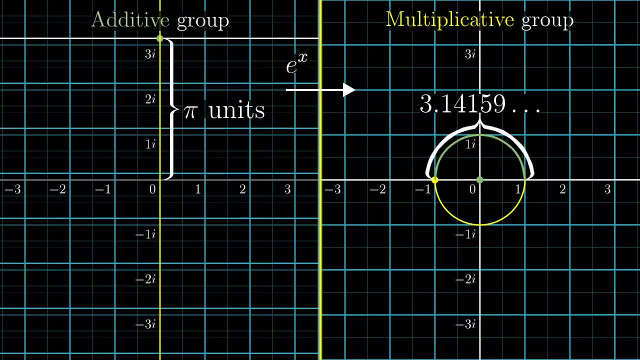 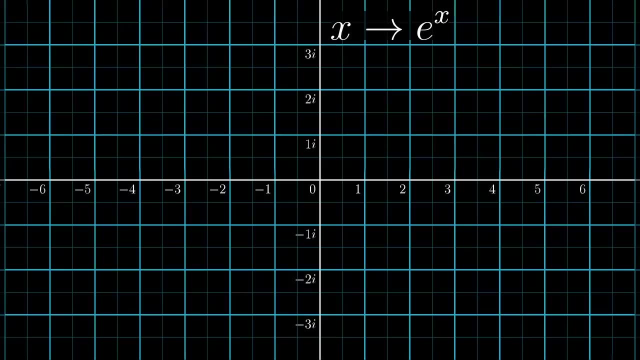 e to the x does this in a very special way that ensures that a vertical slide of pi units corresponds to a rotation of exactly pi radians, the 180 degree rotation associated with the number negative one. To finish things off here, I want to show a way that you can think about. 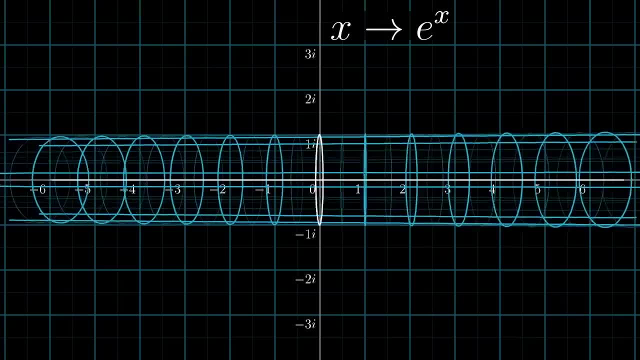 this function e to the x as a transformation of the complex plane. But before that, just two quick messages. I've mentioned before just how thankful I am to you, the community, for supporting me in this work. I hope you enjoyed this video and, if you did, 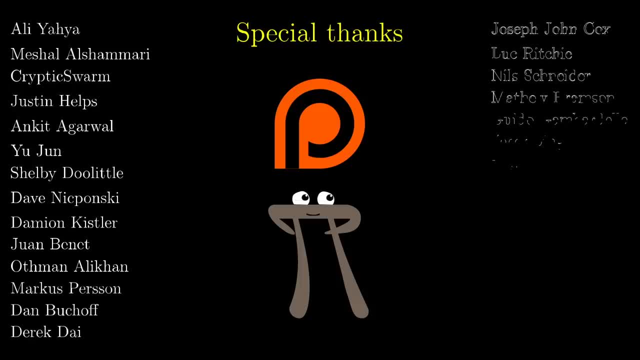 give it a thumbs up and I'll see you in the next one. But in much the same way that numbers become more meaningful when you think of them as actions, gratitude is also best expressed as an action, So I've decided to turn off ads on new videos. 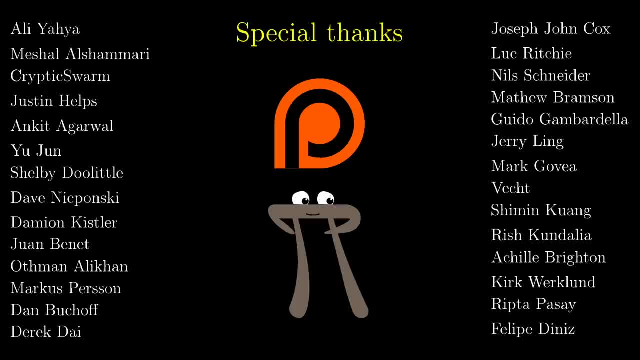 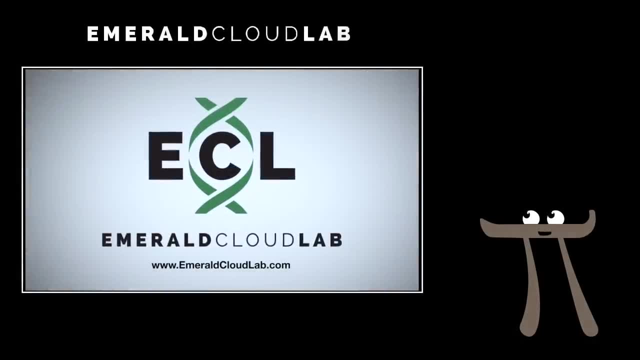 for their first month, in the hopes of giving you all a better viewing experience. This video was sponsored by Emerald Cloud Lab, and actually I was the one to reach out to them on this one, since it's a company I find particularly inspiring. Emerald is a very 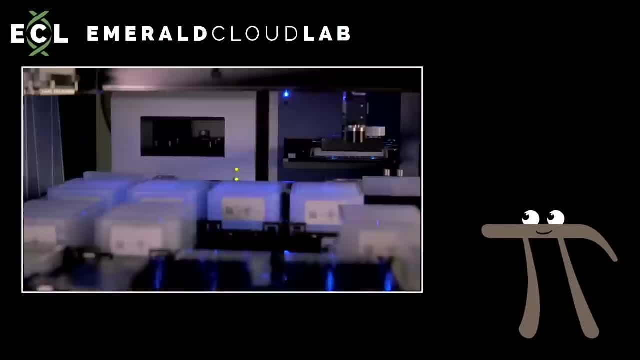 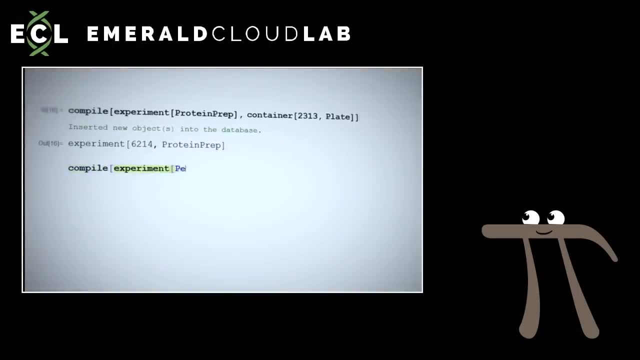 unusual startup: half software, half biotech. The cloud lab they're building essentially enables biologists and chemists to conduct research through a software platform instead of working in a lab. Scientists can program experiments which are then executed remotely and robotically. 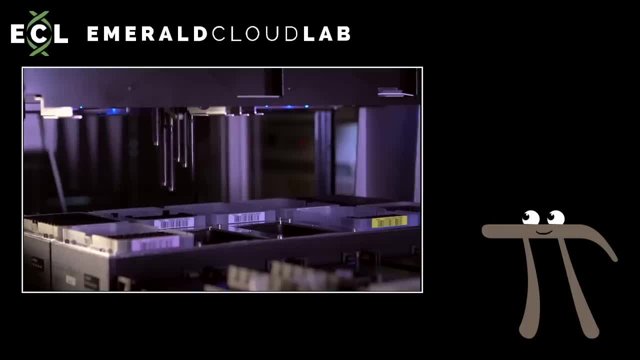 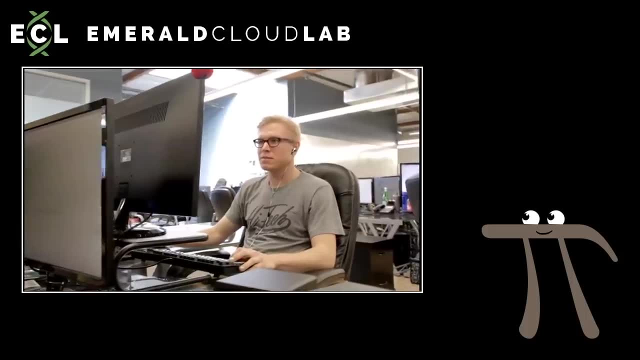 in Emerald's industrialized research lab. I know some of the people at the company and the software challenges they're working on are really interesting. Currently they're looking to hire software engineers and web developers for their engineering team as well as apply to. 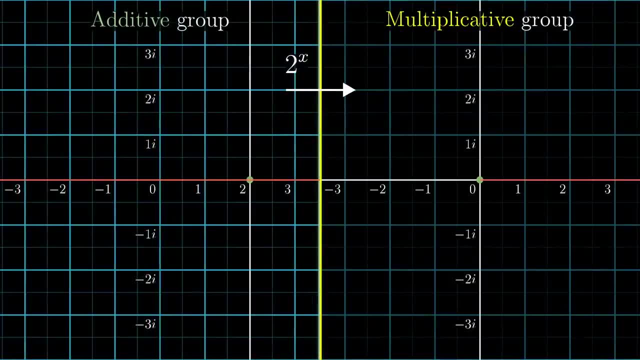 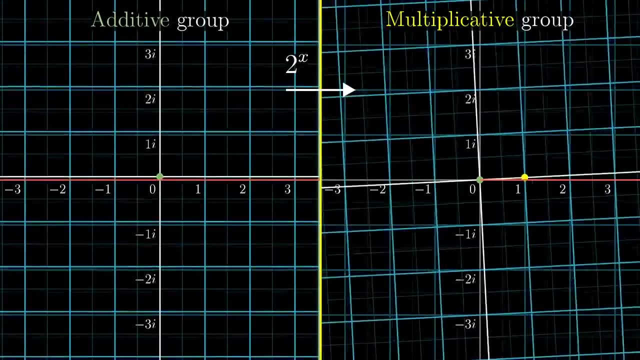 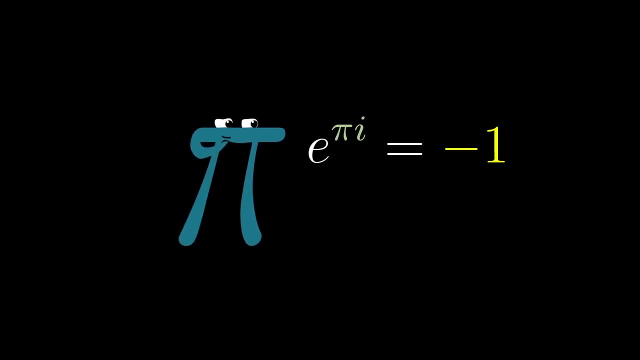 The important point that I want to make here, though, is that, if you view things from the lens of group theory, thinking of the inputs to an exponential function, as sliding actions, and thinking of the outputs as stretching and rotating actions- it gives a very vivid way to read what a formula like this is even saying. 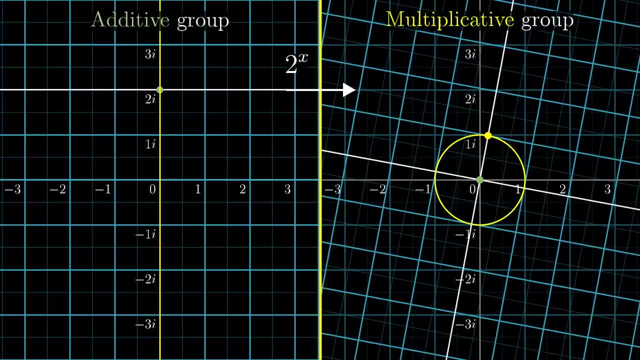 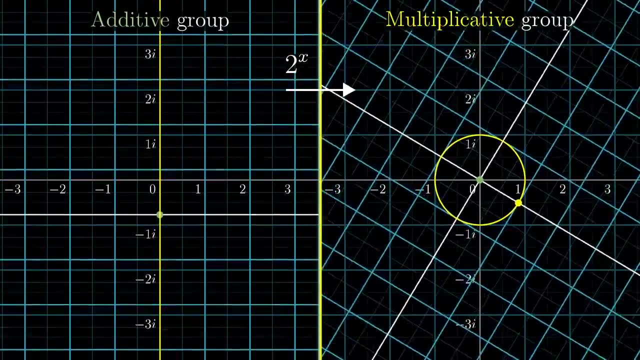 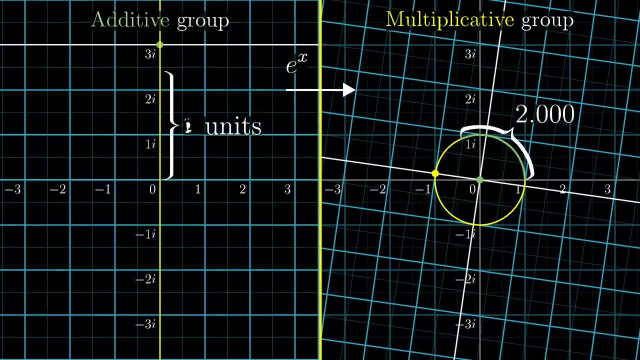 When you read it you can think that exponentials in general map purely vertical, slides the additive actions that are perpendicular to the real number line into pure rotations which are in some sense perpendicular to the real number stretching actions, And, moreover, E to the x, does this in the very special way that ensures that a vertical 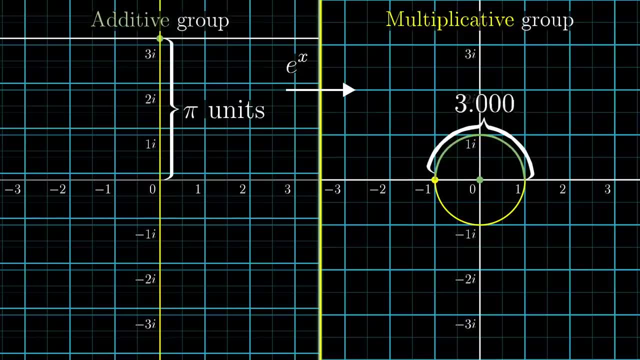 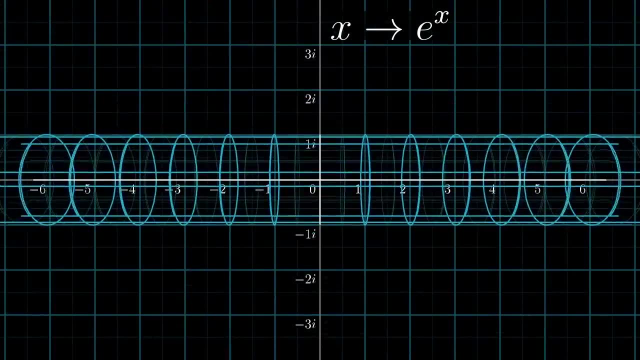 slide of pi units corresponds to a rotation of exactly pi radians, The 180 degree rotation associated with the number negative one. To finish things off here, I want to show a way that you can think about this function E to the x as a transformation of the complex plane. 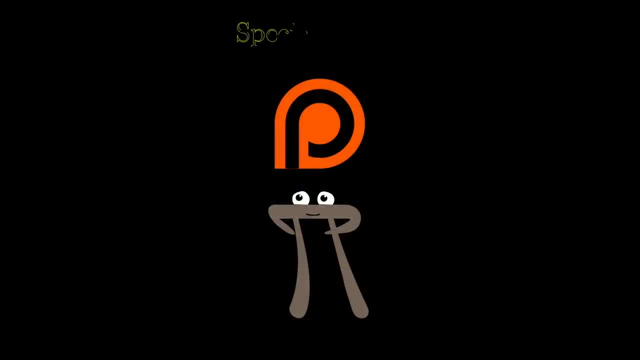 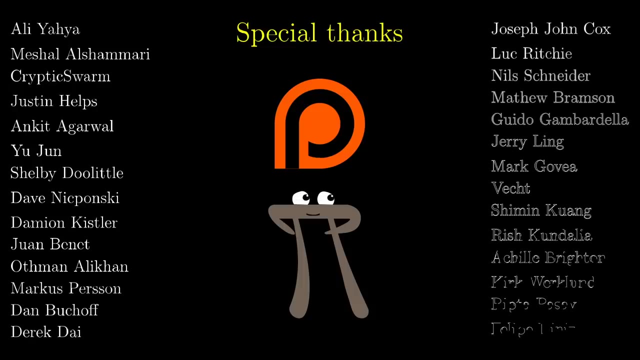 But before that, just two quick messages. I've mentioned before just how thankful I am to you, the community, for making these videos possible through Patreon. But in much the same way that numbers become more meaningful when you think of them as actions, 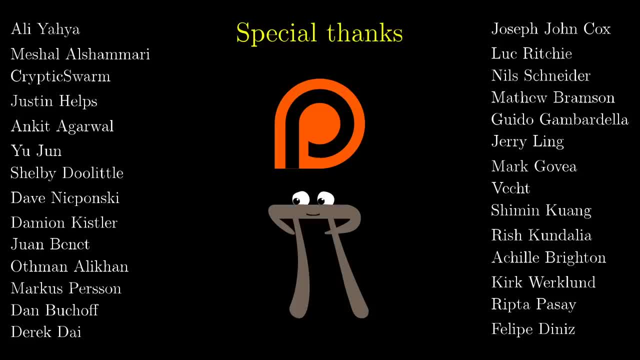 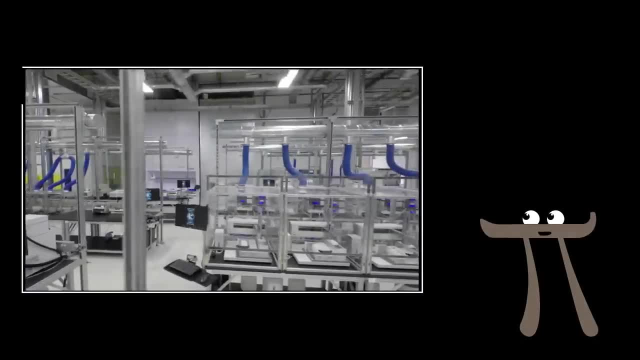 Ad is also best expressed as an action, So I've decided to turn off ads on new videos for their first month, in the hopes of giving you all a better viewing experience. This video was sponsored by Emerald Cloud Lab, and actually I was the one to reach out. 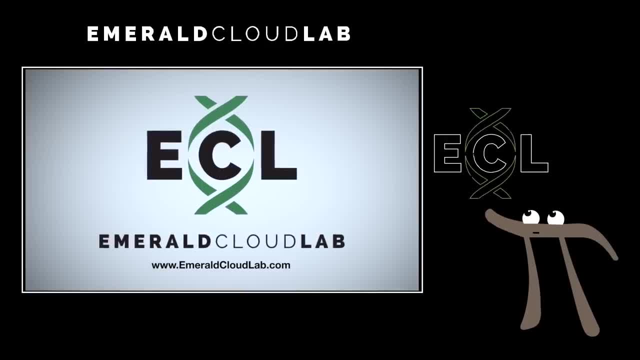 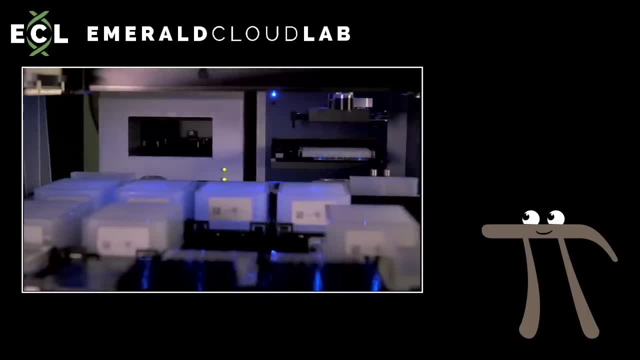 to them on this one, since it's a company I find particularly inspiring. Emerald is a very unusual startup: half software, half biotech. The Cloud Lab that they're building essentially enables biologists and chemists to conduct research through a software platform. 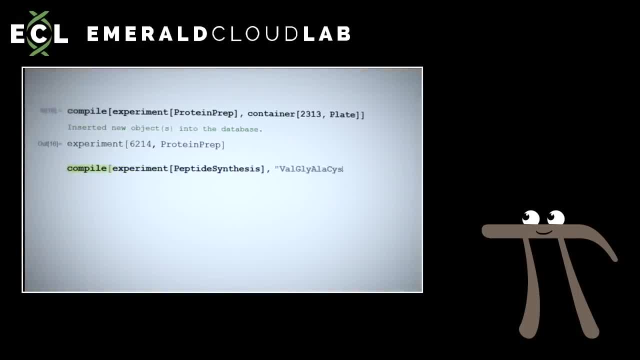 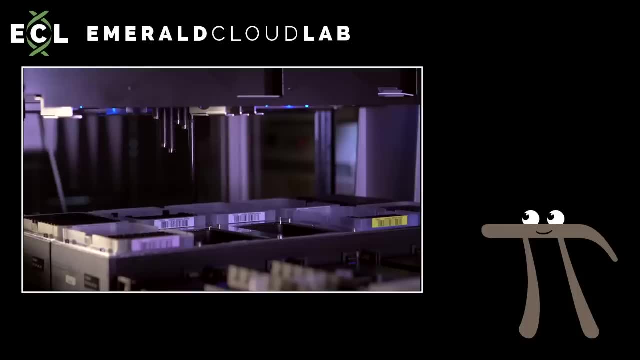 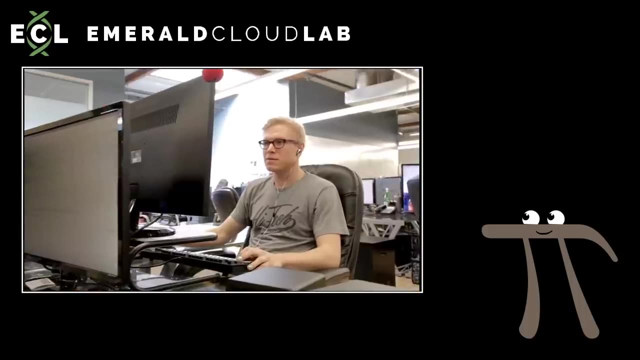 Instead of working in a lab, scientists can program experiments which are then executed remotely and robotically in Emerald's industrialized research lab. I know some of the people at the company and the software challenges they're working on are really interesting. Currently they're looking to hire software engineers and web developers for their engineering. 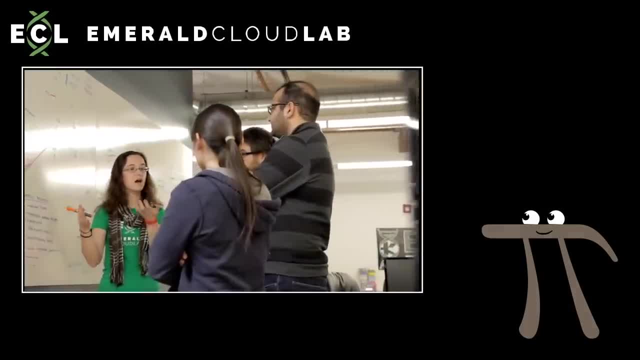 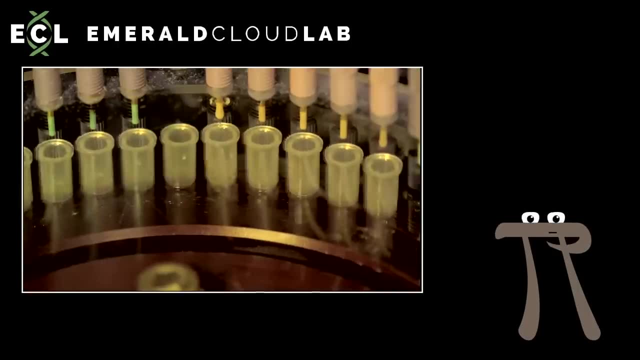 team, as well as applied mathematicians and computer scientists for their scientific computing team. If you're interested in applying- whether that's now or a few months from now- there are a couple special links in the description of this video and if you apply through those, 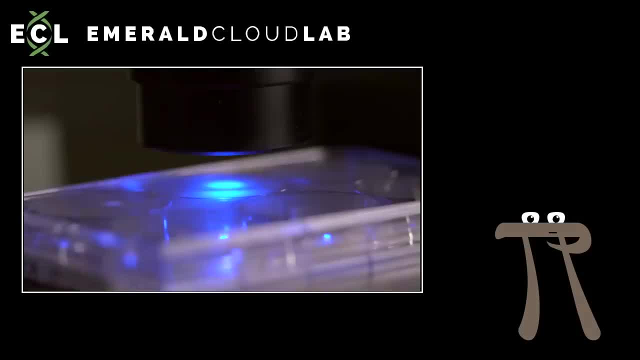 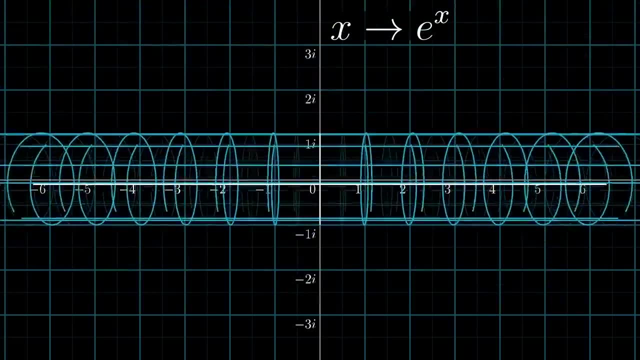 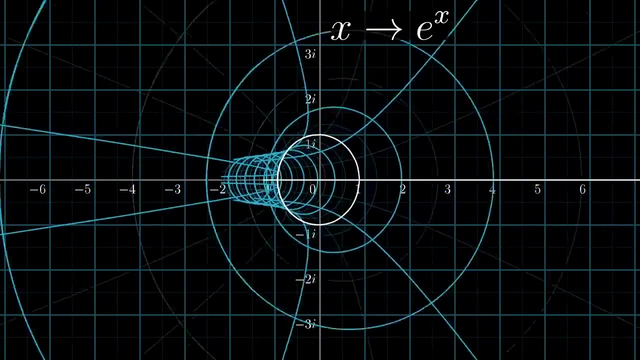 it lets Emerald know that you heard about them through this channel. Alright, so e to the x: transforming the plane. I like to imagine first rolling that plane into a cylinder, wrapping all those vertical lines into circles, and then taking that cylinder and smushing it onto the plane around zero. 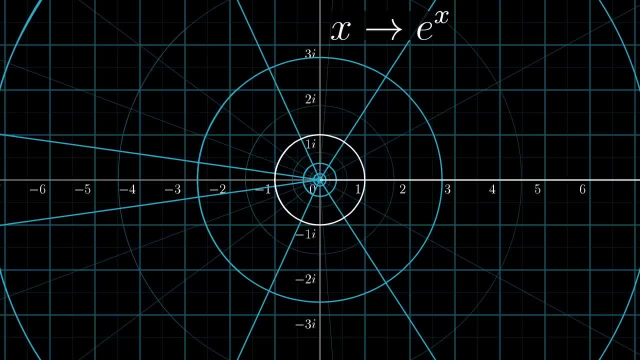 where each of those concentric circles spaced out exponentially correspond with what started off as vertical lines. So that's pretty much it for this video and I'll see you guys in the next one. Thanks for watching. I'll see you guys in the next one. 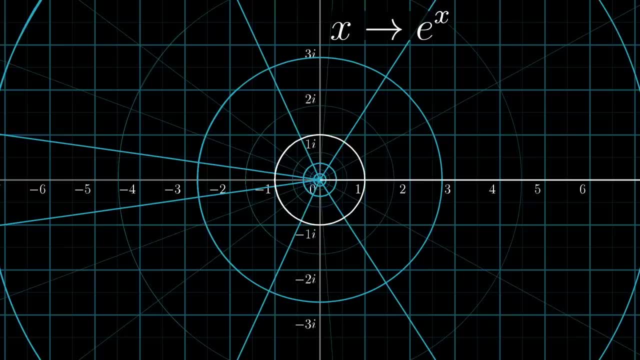 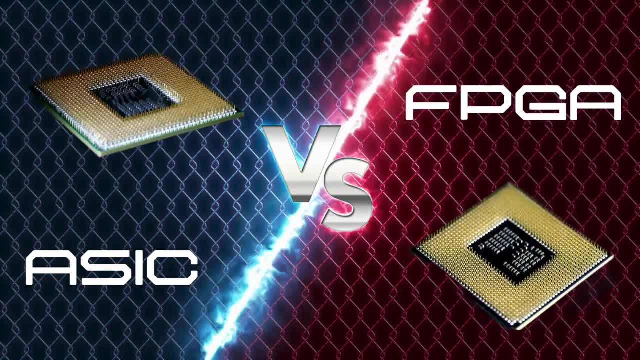 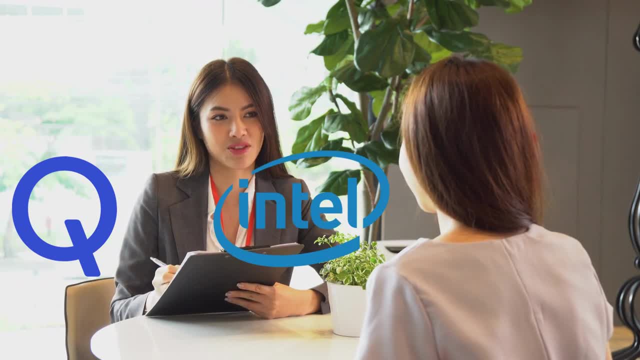 Hello everyone, welcome to my channel. In today's video we will find out the major differences in ASICs and FPGAs. This is often asked in interviews of companies like Qualcomm, Intel and Nvidia. This is your friend, part-time coder. Please like and subscribe to my channel. 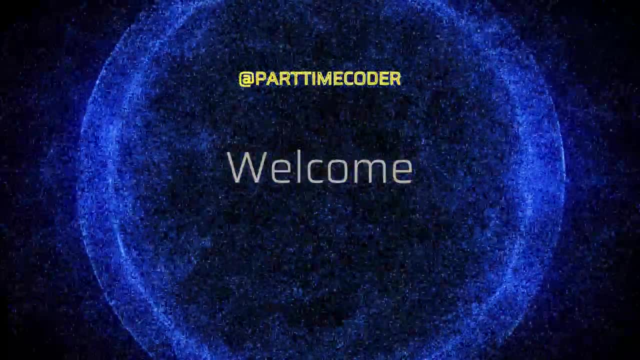 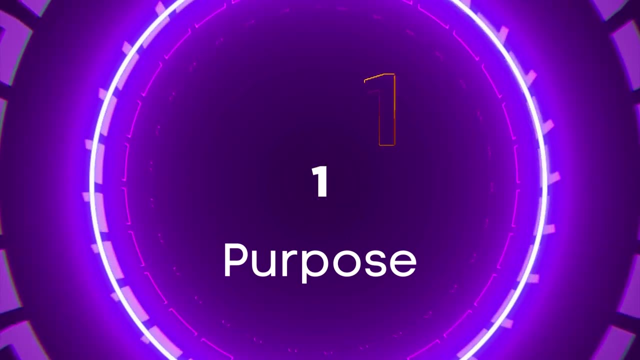 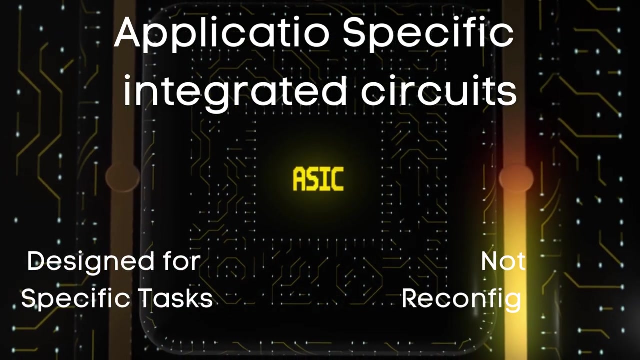 if you like this video. In this video we will go over six major differences. First we will discuss about purpose. ASIC stands for Application Specific Integrated Circuits. These are designed for specific tasks and are not reconfigurable. For example, an ASIC designed for office lift cannot be. 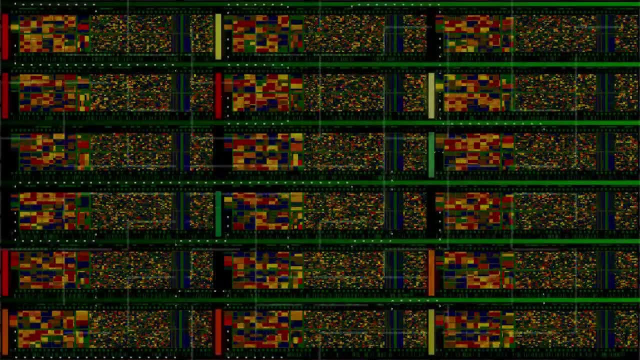 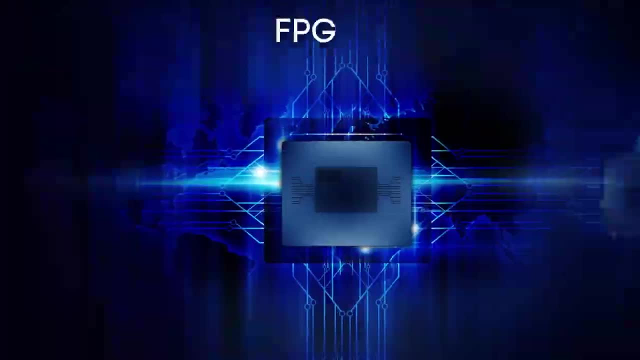 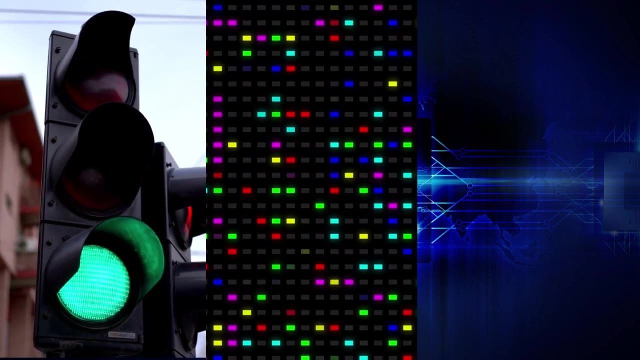 configured to do any other task. FPGA stands for Field Programmable Gate Arrays. They are highly flexible and can be reconfigured to adapt to changing gates. So, basically, you can program an FPGA to be used as a traffic light controller, or you can use it as a display driver or even as a temperature controller. 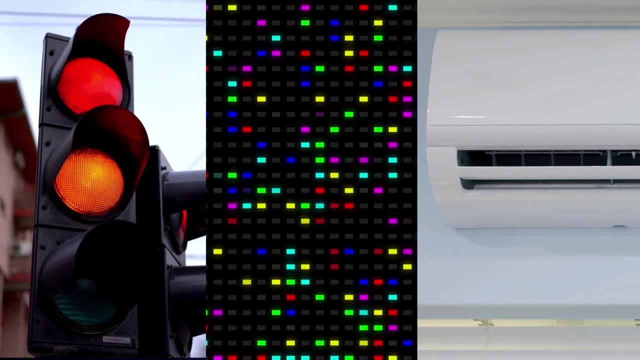 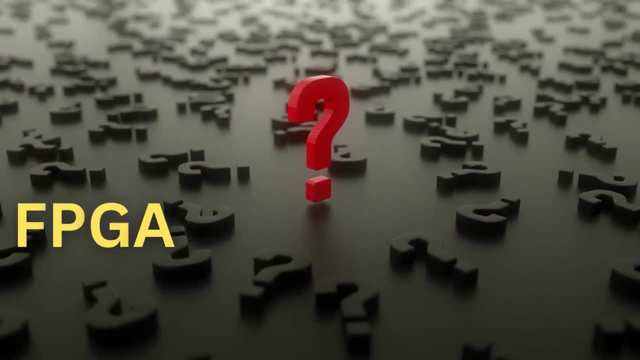 in AC. They allow for the application to be configured to be used as a display driver or even as a remote controller. They also allow for the implementation of various designs, making them a versatile option for multiple applications. Now you must be thinking if FPGAs are so much reconfigurable and can be used in multiple 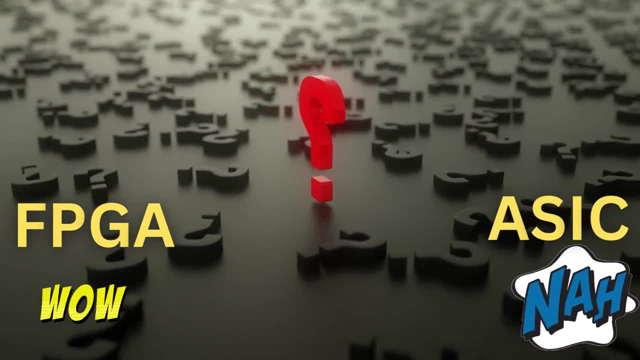 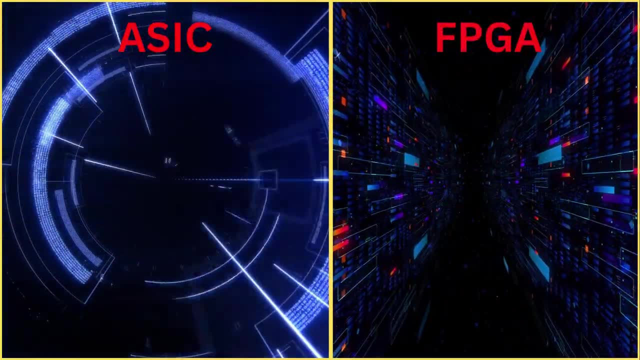 applications. why do we need ASICs? We will understand the need of ASICs in upcoming points. Second is performance. ASICs offer a significant advantage in performance as they are specifically designed for a specific task and therefore run faster. For example, an ASIC designed